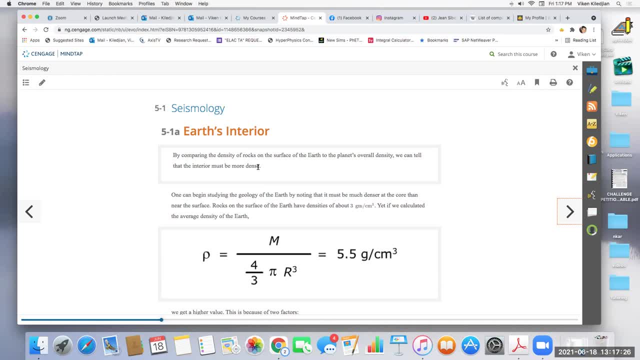 important quantities to describe something. So it tells you how much mass is compacted into a certain volume, right? So one can begin studying the geology of the Earth by noting that it must be much denser at the core than near the surface. 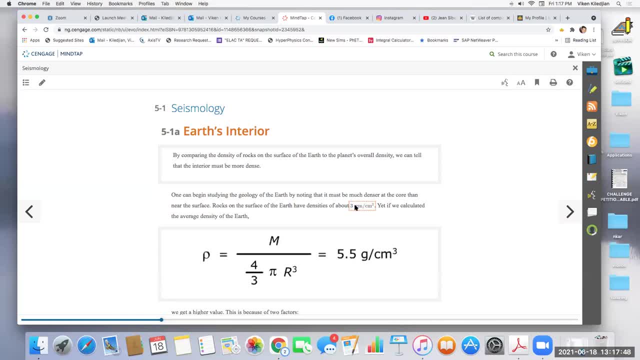 Rocks on the surface of the Earth have densities of about two grams per cubic centimeter. So that's the density of the rocks at the surface of the Earth. They're about three grams per cubic centimeter. You can see why the density size for the Earth is so big. but when we calculate the average density of 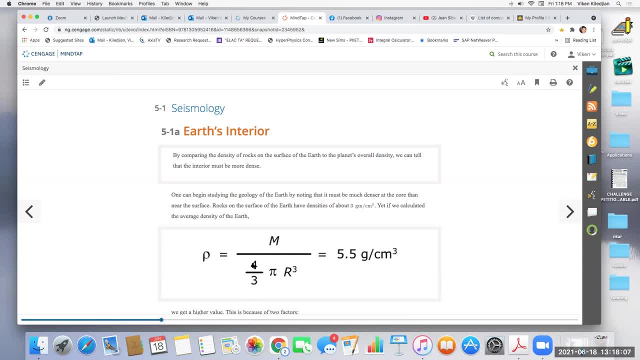 the Earth by taking its mass, by multiplying by the volume of the Earth. this is this is the equation for the volume of the sphere. So if you do the volume of the Earth and then you take its mass and you divide them, you get 5.5 grams per cubic centimeter. So you see, you could tell that the overall density of the Earth is denser than the density of the rock's at the surface. So that means the interior water density is smaller the surface density of the rock. 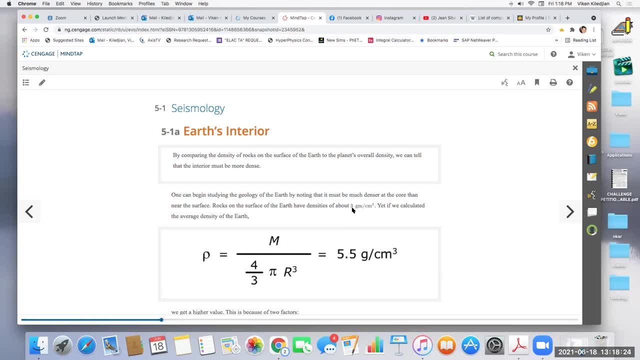 And now the other point is: toкольку You get aだけ difference in weight from a volume that represent a battery pepper on the earth to a volume of a FREELESS nature. So, But in order to calculate a bit more specific thing, we're not taking this talking about balance or just uh, but we're taking a lot of information from Earth. 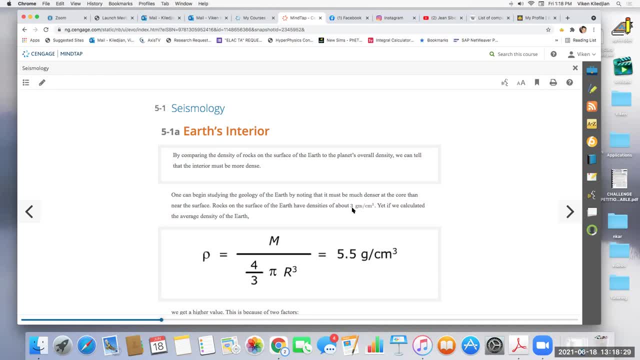 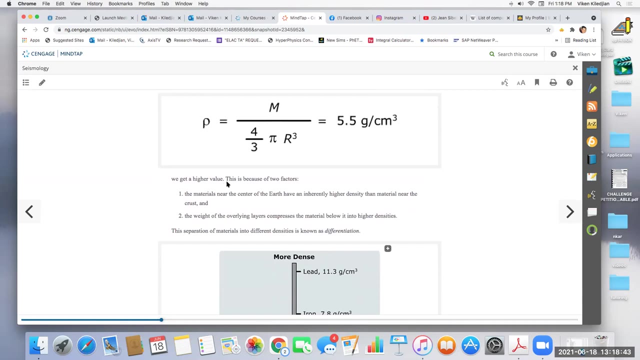 So that means the inside of the earth must be denser. It must be keep getting denser and denser as you go to the core of the earth. So it says this is because of two factors: The materials near the center of the earth. 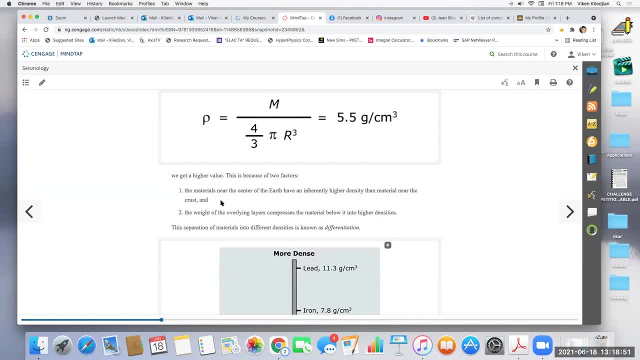 have an inherently higher density than the material near the crust. Yeah, I see, kind of like I said, the denser material sinks down into the core of the earth, And this is also similar for other planets. So we would expect that the denser materials are in the core. Then the second one is the weight of the overlying layers compresses the material below it into a higher densities. That means that also causes the density of the core to be higher because you've got all the weight of the objects on top of it pressing down on it. 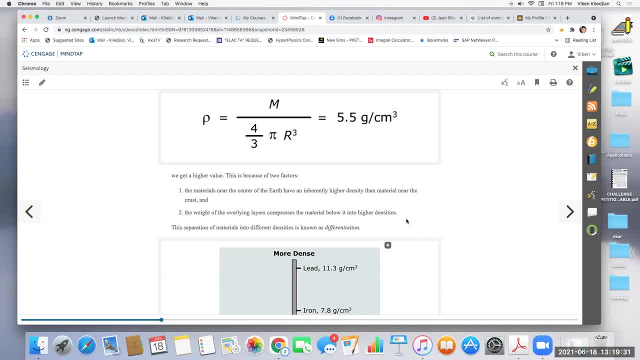 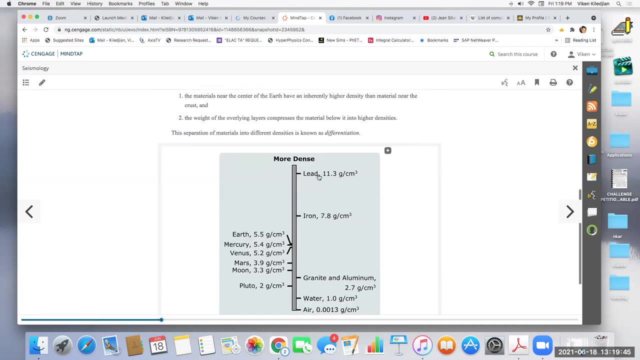 So it compresses it into a smaller volume. By doing that, it makes the density even higher. This separation of materials into different densities is known as differentiation. So, for example, they give you materials here and their densities lead is 11.3 gram per cubic centimeter. Oh, The density of the earth is 7.8 gram per cubic centimeter. And then you got the densities of some of the planets. Earth is the densest planet, with a density of 5.5 gram per cubic centimeter. Mercury is a close next 5.4.. 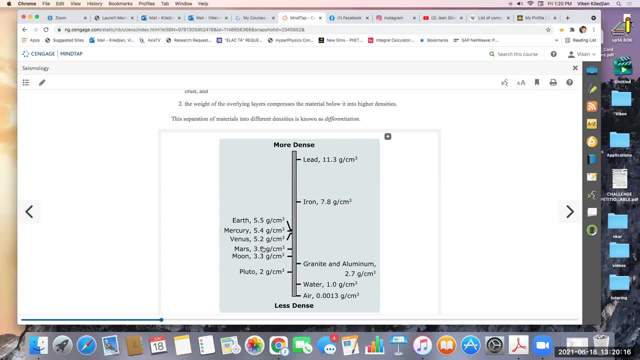 Venus is next, Mars is less, and then the moon is even less, So the less the density of the planet. that means that planet is more dominated by rocky material. The moon is probably more rocks and granite or whatever You see. here we can see that granite and aluminum. have a density of 2.7.. That means the moon is mostly made up of those kinds of materials like granite rocks. maybe slightly denser. Mars probably has some more stuff in its interior, but not that much. But Mercury and Venus. they're more like earths. 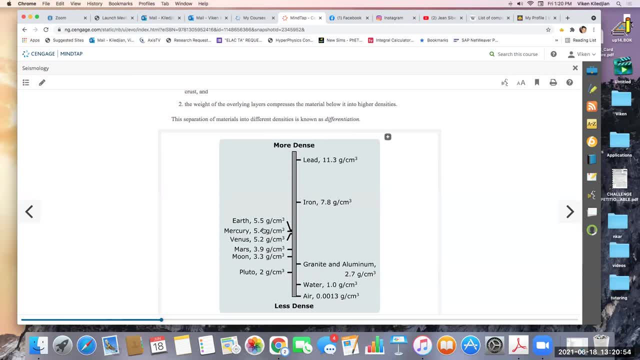 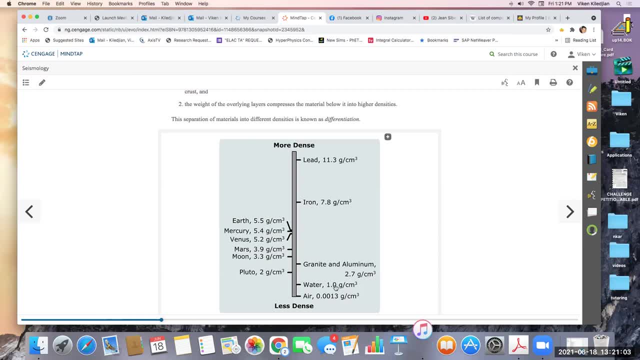 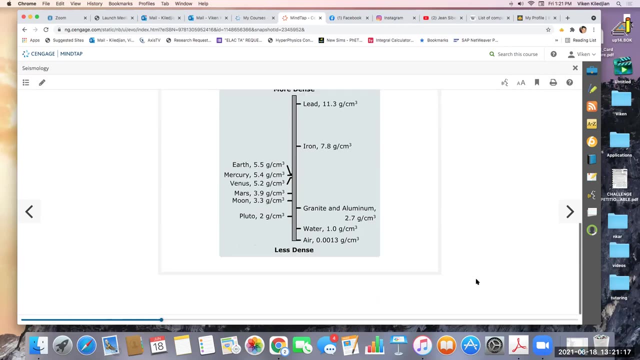 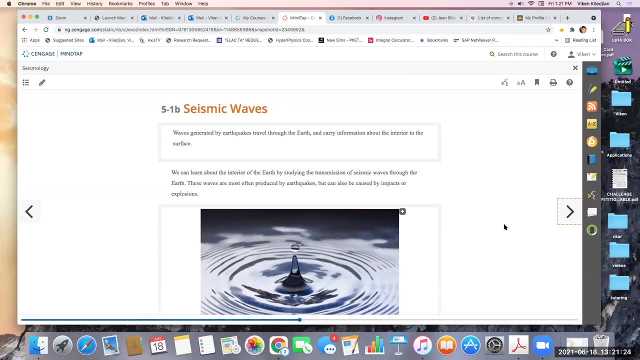 That means it's probably just a little bit more or twice more dense than water, So that means it's primarily composed of water and ice and some other heavier material, but not that much Okay. So seismic waves- Waves generated by earthquakes- travel through the earth. 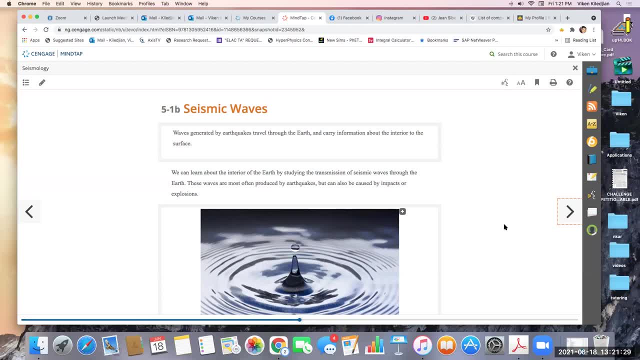 and carry information about the interior to the surface. We can learn about the interior of the earth by studying the transmission of seismic waves through the earth. These waves are most often produced by earthquakes, but can also be caused by impacts or explosions. Seismologists identify two different types. 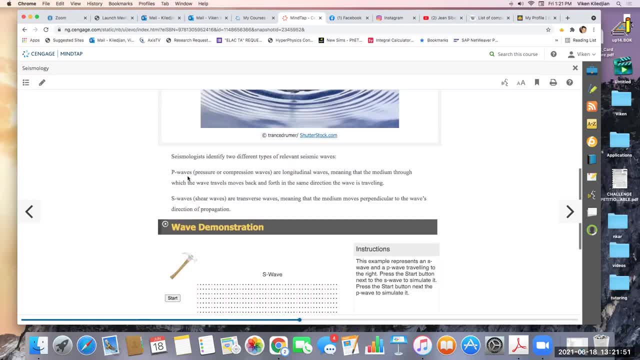 of relevant seismic waves: P waves, which is a wave of pressure or compression wave. This is a pressure or a compression wave- are longitudinal waves, meaning that the medium through which the wave travels moves back and forth in the same direction that the wave is traveling. 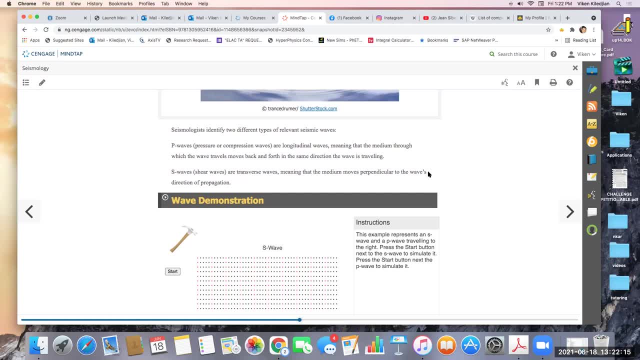 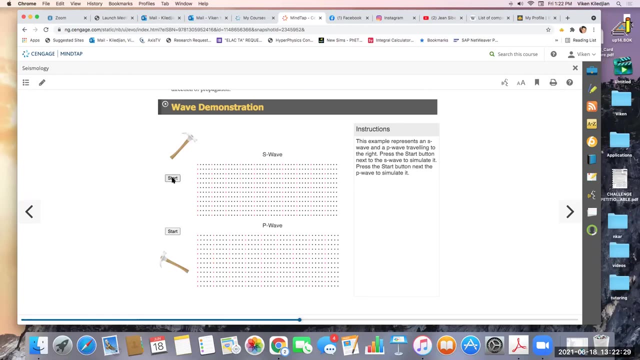 S waves are transverse waves, meaning that the medium moves perpendicular to the wave's direction of travel. So S is perpendicular, are longitudinal, which means it's parallel. so let's look at a simulation here. this would be an S wave. you see how the material goes up and down and the 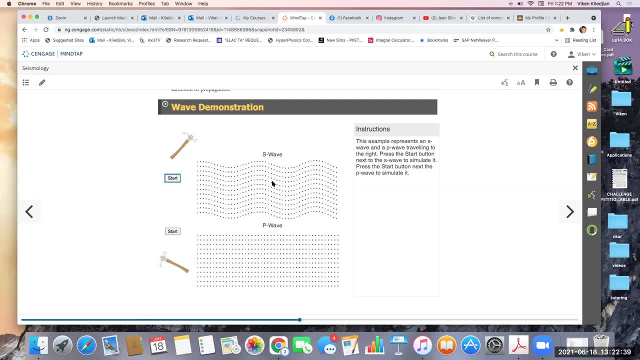 wave travels from left to right and back and forth, and back and forth, but the material is going perpendicular to it, up and down, you see. so if a S wave is coming to your house, your house would shake up and down as the earthquake is passing by you. I believe S waves would do more damage to the house, to buildings P. 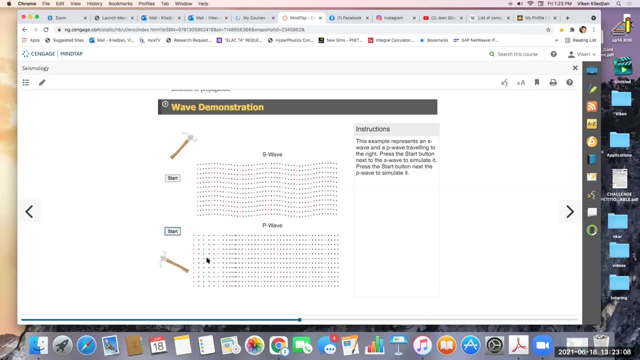 waves is this way. you see, then the house would shake left and right like this. so this is a longitudinal wave. the objects are going back and forth as the wave is traveling from left to right and back and forth. In other words, they're oscillating in the same direction, parallel. 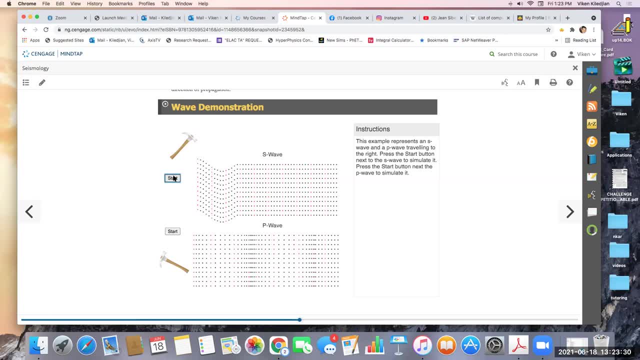 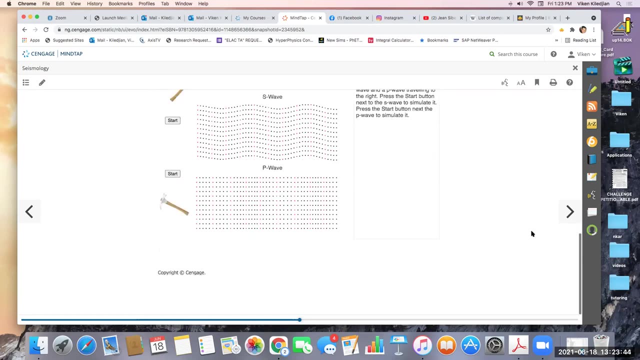 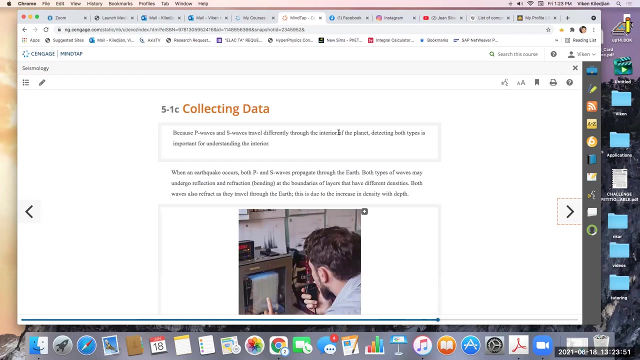 I like doing that. Yeah, P waves would not do as much damage to buildings as much as the S wave. Okay next. So because P waves and S waves travel differently through the interior of the Earth, detecting both types is important for understanding the interior. When an earthquake occurs, both P and S waves propagate through the Earth. Both types of waves may undergo reflection and refraction. That means bending, Okay, So they can reflect. They can reflect, refract and bend right at the boundaries of layers that have different densities. 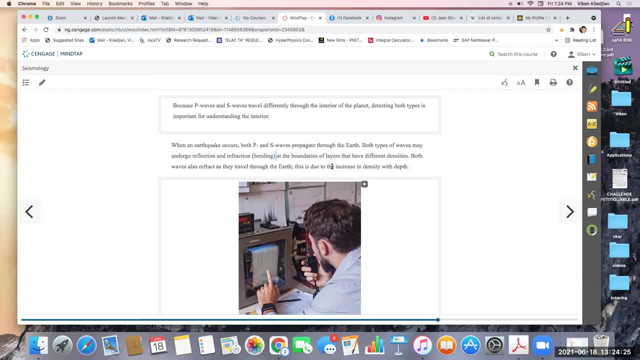 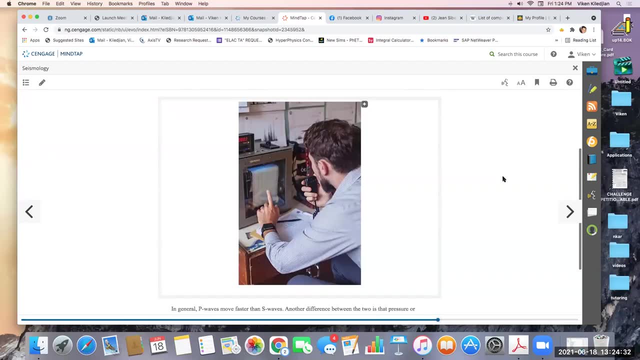 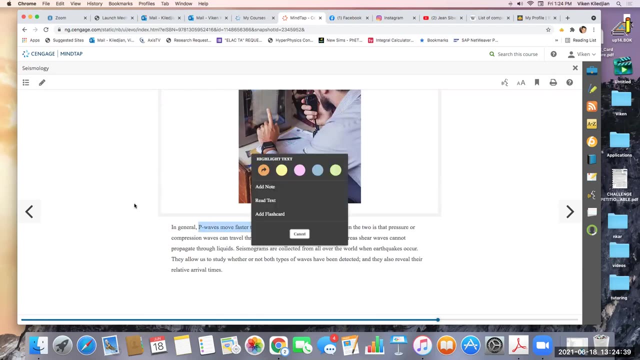 Both waves also refract as they travel through the Earth. This is due to the increase in density with depth. So in general P waves move faster than S waves. So that's one thing to note. P and you can kind of remember P with the word primary and S with the word secondary. 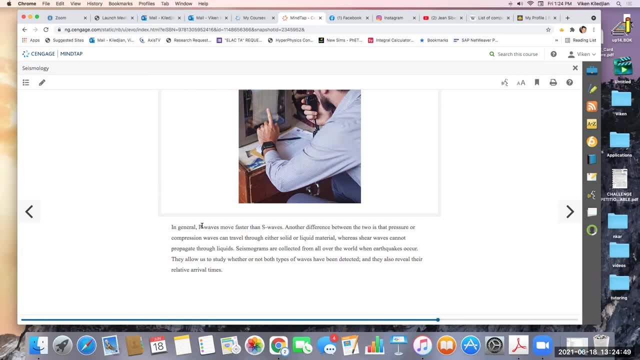 So the P wave is the one that's going to reach your house first. That's the primary wave, Then, a little bit time later, the S wave, the secondary wave, is going to reach you, And that's going to shake you up and down. 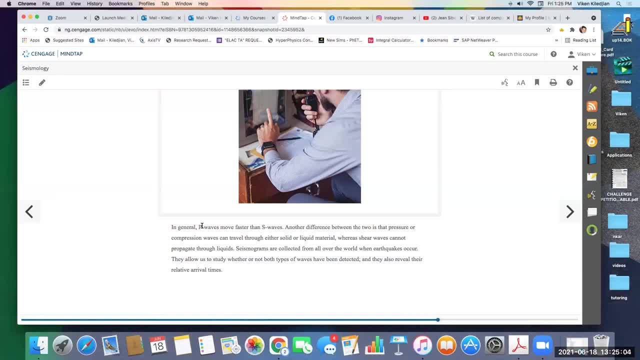 Whereas the P wave is going to shake your left and right. So another difference between the two is that the pressure or compression waves can travel through either solids or liquids. So that means these guys can travel through solids. So they can travel through solids or liquids, both. 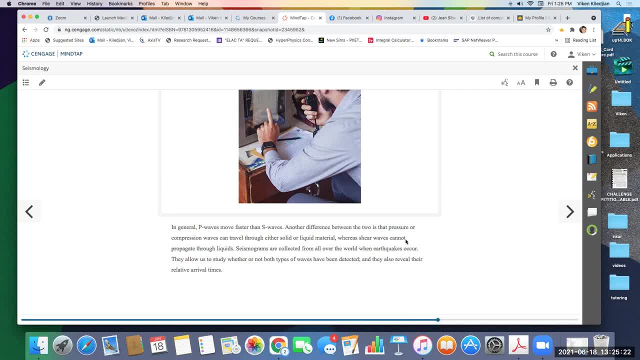 And then the S wave, whereas the shear waves cannot propagate through liquids. So remember it this way: S for solid, So S waves cannot travel through. solid Cannot, Okay, So they are secondary, That means they're slower. And they also cannot travel through. Hold on Shear waves cannot propagate through liquids. Oh, I think I said it wrong. No, hold on S is the secondary S waves means they can only travel through solids. Oh, I said it wrong. 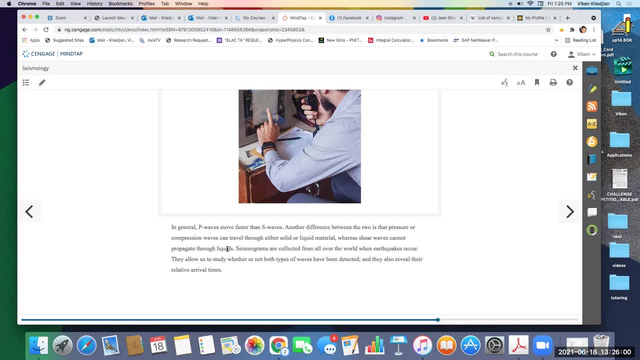 Yes, yes, So shear waves cannot propagate through liquids, which means they can only travel through solids. Yes, Now I said it correctly. So S wave is secondary and they can only travel through solids. Seismograms are collected from all over the world when earthquakes occur. 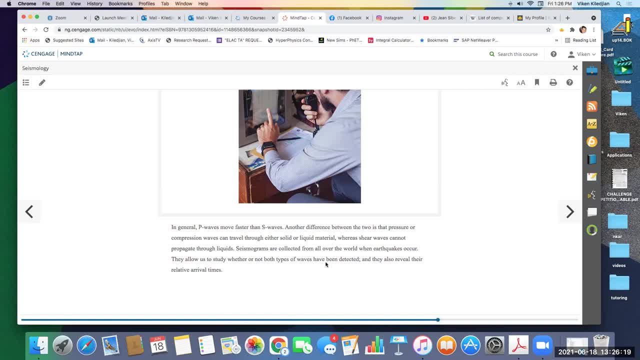 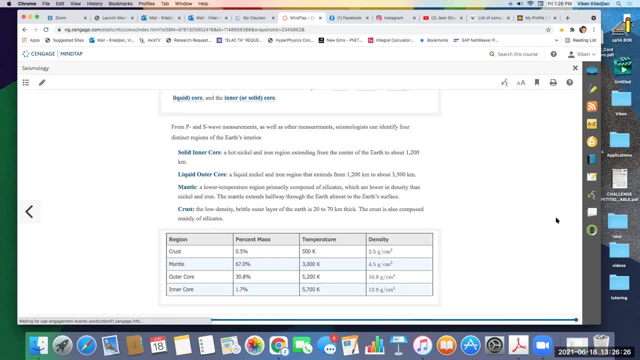 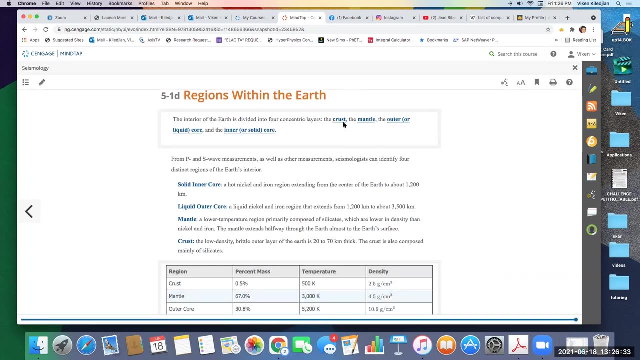 They allow us to study whether or not both types of waves have been detected and they also reveal their relative arrival times. So regions within the Earth, The interior of the Earth is divided into four concentric layers: The crust, the mantle, the outer, or liquid core and the inner, or solid core. 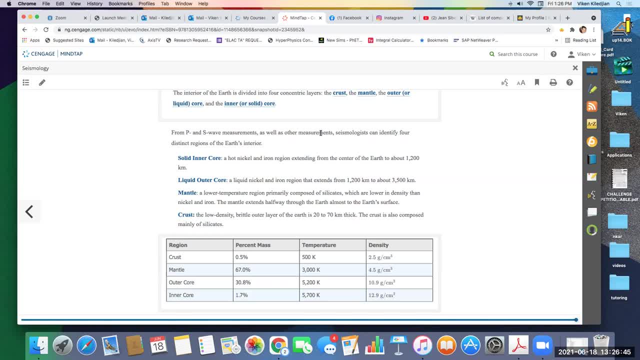 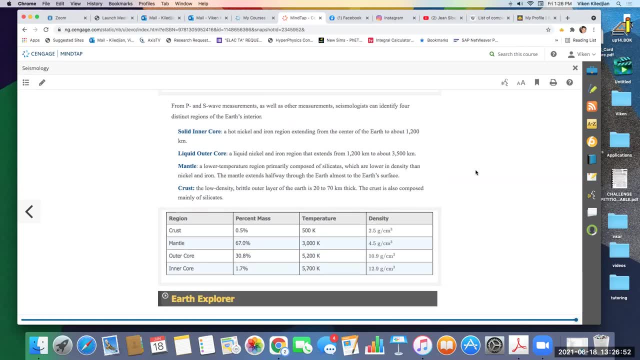 So from P and S wave measurements, as well as other measurements, seismologists can identify four distinct regions of the Earth's interior: Solid inner core, a hot nickel and iron region extending from the center of the Earth to about 1,200 kilometers. 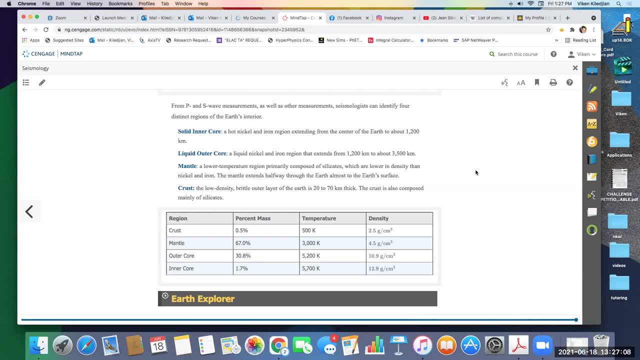 Liquid outer core: a liquid nickel and iron region that extends from 1,200 to 3,500.. Solid inner core: a hot nickel and iron region that extends from 1,200 to 3,500.. Solid inner core: a hot nickel and iron region that extends from 1,200 to 3,500. 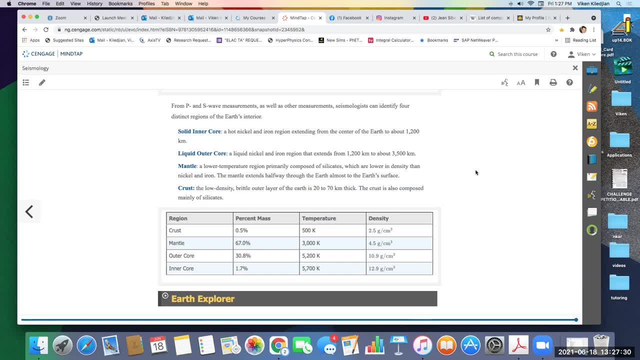 The core of the surface is at the center of the Earth and it's called the mantle region. This is the mantle region, the upper part of the mantle region. The upper part of the mantle region is a lower temperature region primarily composed of silicates. which are lower in density than nickel and iron. So silicate means anything that has silicon and oxide. Silicon and oxide- that's a silicate, and it's kind of like where we get our sand from. That is actually a silicate. 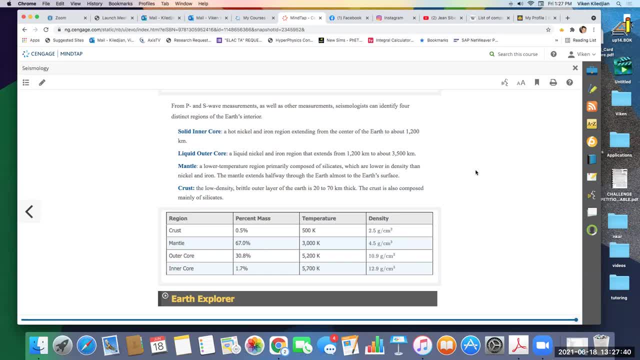 It's composed of silicon bonded with oxygen, And that's where our natural gas content comes from. So this is a silicate. So this is a silicon that's called the silicate. the mantle extends halfway through the earth, almost to the earth. 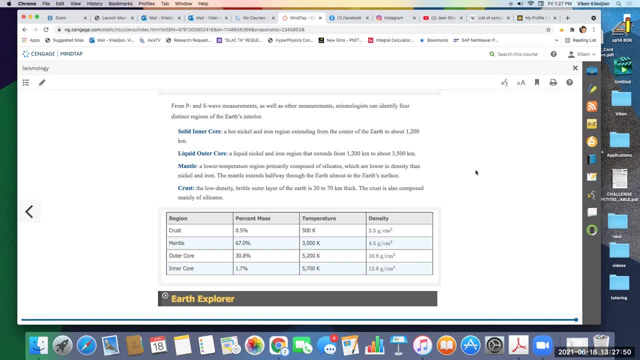 surface. the crust, the lower density, brittle outer layers of the earth is 20 to 70 kilometers thick. the crust is almost composed mainly of silicates and, of course, rock. so the crust. the percentage of the mass. so the crust: uh, that means the crust comprises 0.5 percent. 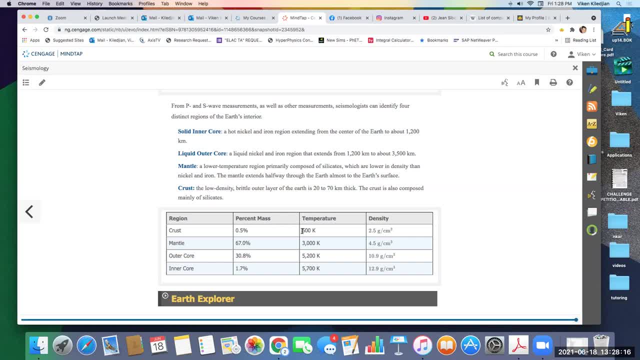 of the mass of the earth and its average temperature is 500 kelvin. that's still warmer than room temperature. room temperature is 300 kelvin. that's the temperature we live at. on the surface of the earth is about 300 kelvin, so that's 200 degrees above room temperature. so 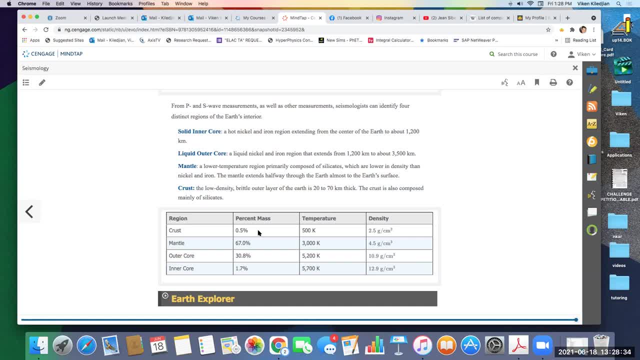 that's the temperature we live at means if you dig into the crust, your metals will already start melting. you can't dig too much because the temperature is going up by 200 kelvin. the average density of the crust is 2.5 gram per cubic centimeter. the mantle comprises 67 percent of the mass of the earth. 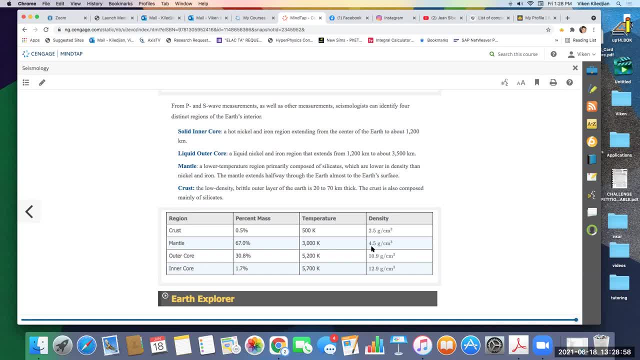 the average temperature 3000 kelvin, and then the density is starting to go up right: 4.5, the outer core 30.8. the temperature is going up, the density is going up. by the time you get to the inner core the density is 12.9. so if you kind of average all these densities then you get um, then 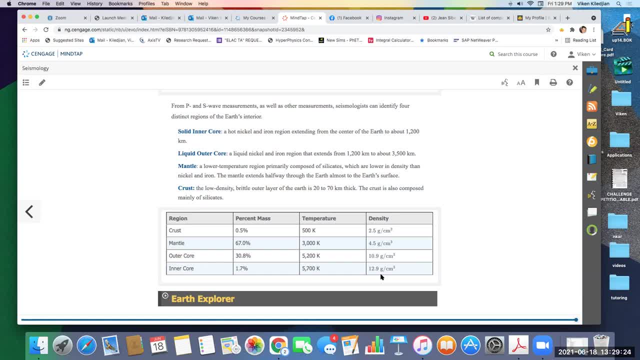 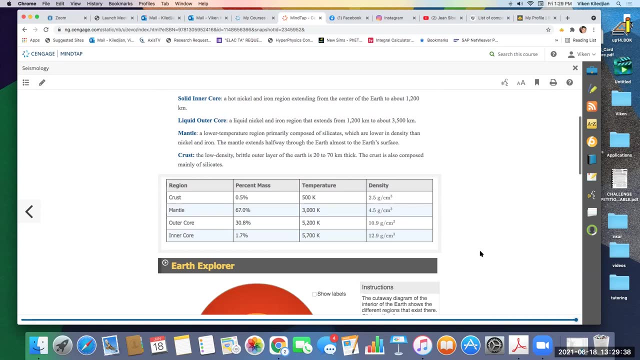 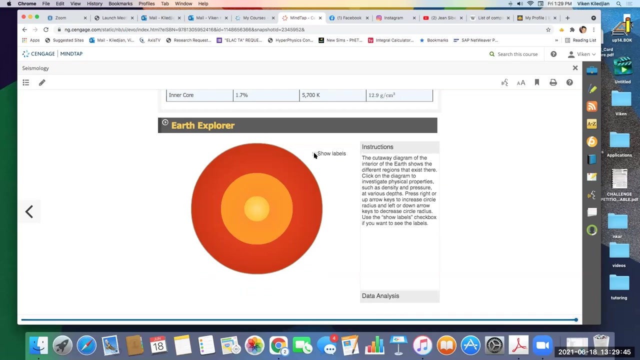 you get the total density of the earth. which was what did we say? it was 5.5. 5.5 is the average density of the earth. w we're gonna get the total density of the earth. oh, that's already better. so, earth explorer, uh, let's see here, let's show labels. yeah, so the inner core. 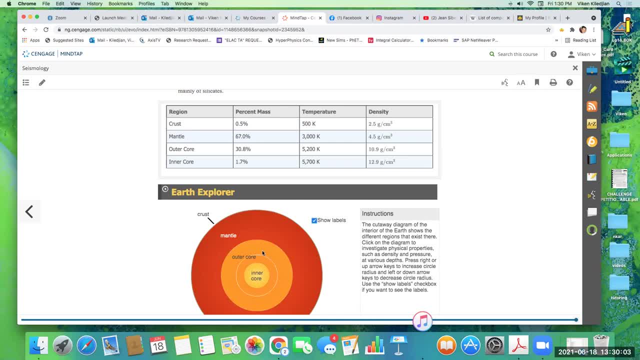 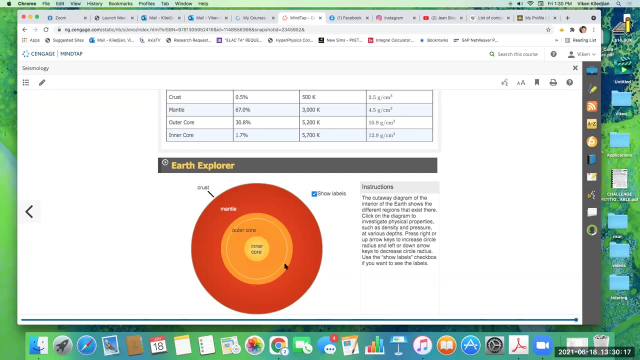 this is the solid portion, is the part the orange is the part that's liquid, okay, and then you got here it's solid. so it's like i kind of remember the movie the, when you go to the, the center of the earth, and there's sea there. 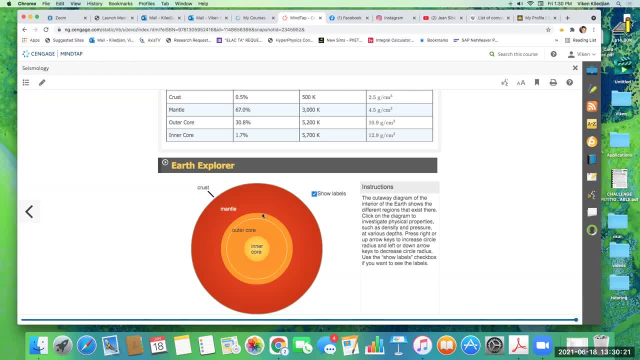 the journey to the center of the earth movie, right, in a sense that that that movie is kind of true. if you were to go all the way to the center of the earth right there, this part would be liquid and you could almost like, uh, get a boat and ride on that, of course, if you can withstand. 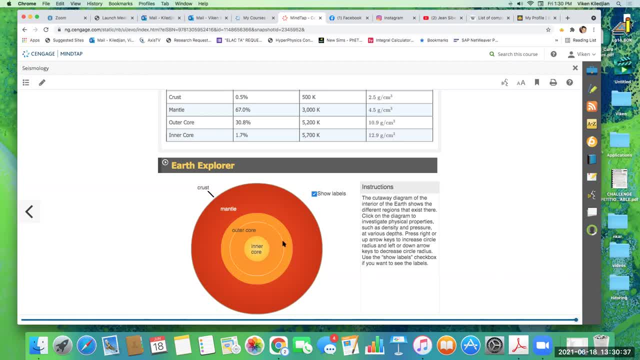 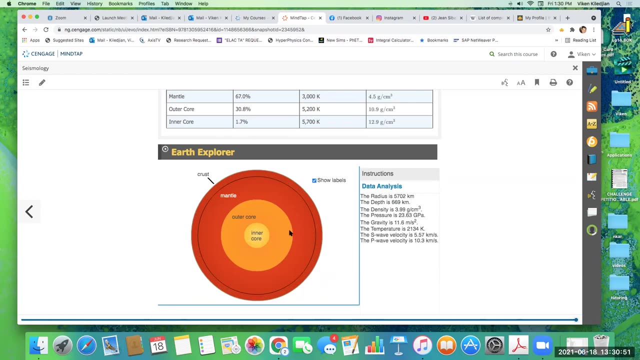 the temperatures. but it is, there is a water, there is a liquid there. so in the sense it's, it is kind of, um, not that wrong, uh. then you get here, oh okay, so it gives you the whole thing here. oh, so if i click on this, it will give me the all the. so if i go like that, 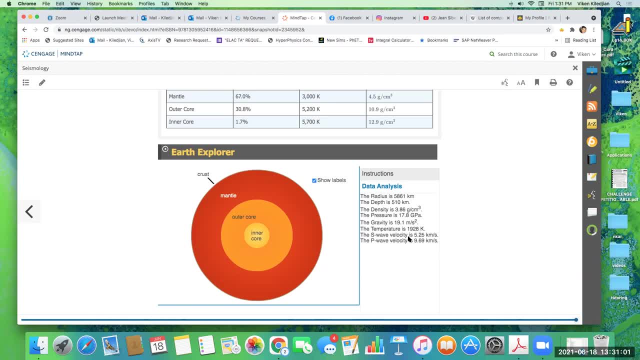 it gives you the whole thing about the temperature of each one, the s-wave velocity. you see, the s-wave velocity, uh, the p-wave velocity, so the s-wave velocity, or as you're going down, the velocities keep changing, you see. so you can kind of like click. 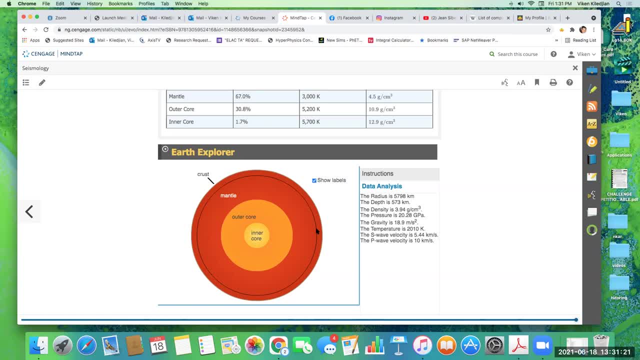 here, uh, the density is 3.94 at that point, the pressure is 20.28 gigapascals, gravity is 18.9. so the gravity at the surface of the earth is what nine point? it should be 9.8 at the surface of the earth. that's, uh, the acceleration due to gravity. now, as you're, 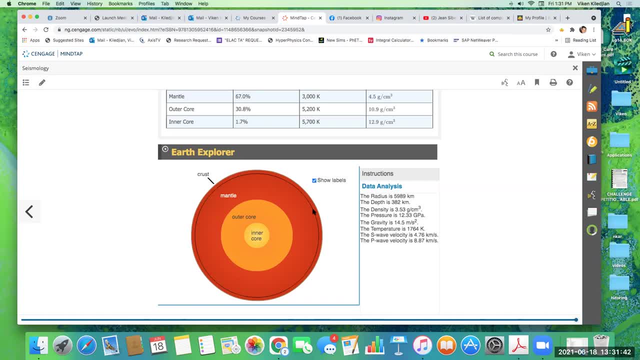 going down, the gravity is increasing, the temperature is increasing and notice the s-wave velocity and the p-wave velocity is also slowly increasing as i go down. so like that, then like that. well, the s-wave velocity is negative. that's weird. the p-wave velocity then 0.48. 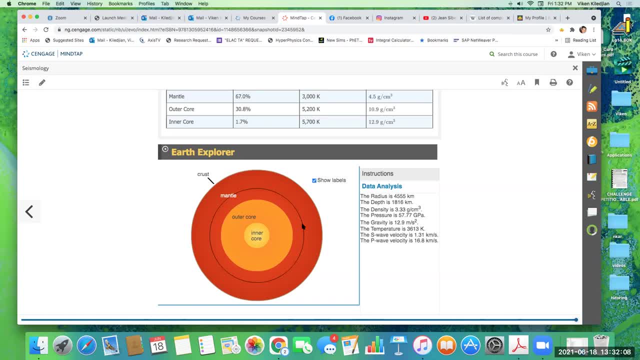 like that. so the p-waves are always faster and the temperature keeps increasing. temperature keeps increasing. now, if i go here, s-wave velocity is zero. what do you notice there? you see the gravity. at that point the gravity is nine point. so right there, you see, right, there's. 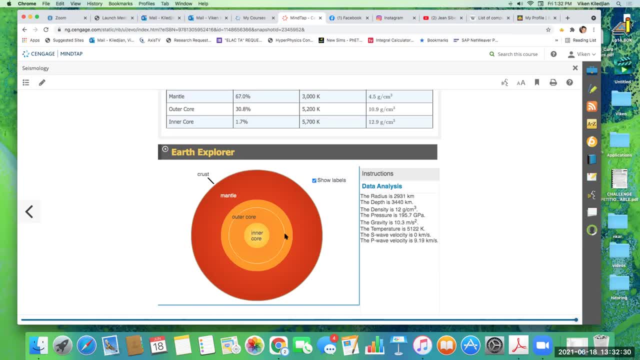 somewhere there, yeah, somewhere there- you would weigh the same thing that you do at the surface of the earth, because the gravity is back to 9.8, yeah, right around there. so if you were to go down, essentially into the center of the earth, your weight would increase, increase, increase until you reach that point. right at that point, then, at 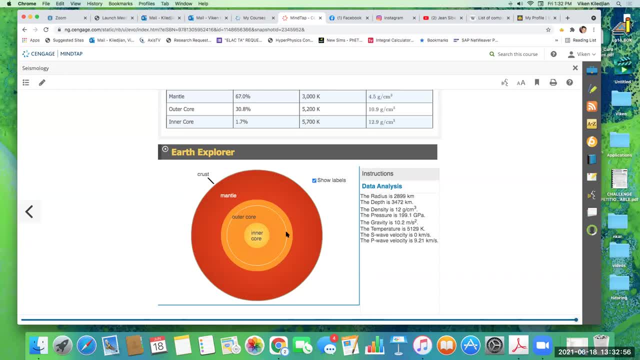 that point the gravity would be, uh, 9.8, so the gravity would be at the center of the earth. it's you would weigh the same thing that you do on Earth, But of course the temperature is very hot. Now, what do you notice about the S-wave? 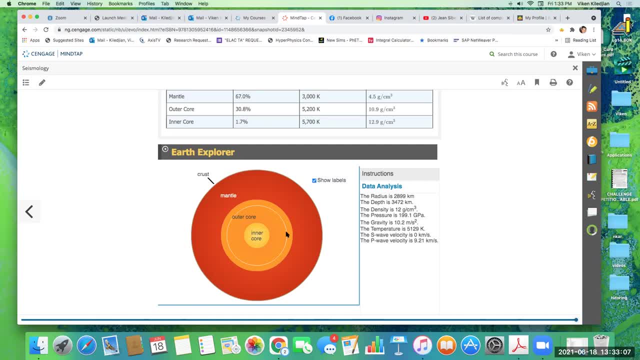 Remember we said S-wave can only travel through solids, So the velocity in the liquid core is zero, You see, But the P-wave is still traveling through the liquid portion. Then you go like that, You go like that, Okay, And then the S-wave is back on. 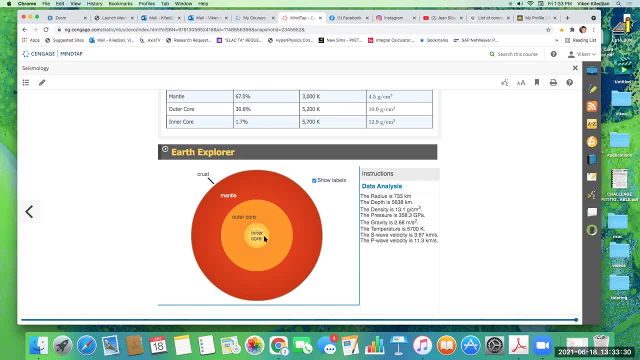 But the problem is, if he can't penetrate the liquid core, then what good is it that he can travel through the inner core? He won't even get there Right. So now the one thing you notice about the temperature is it's still going up. 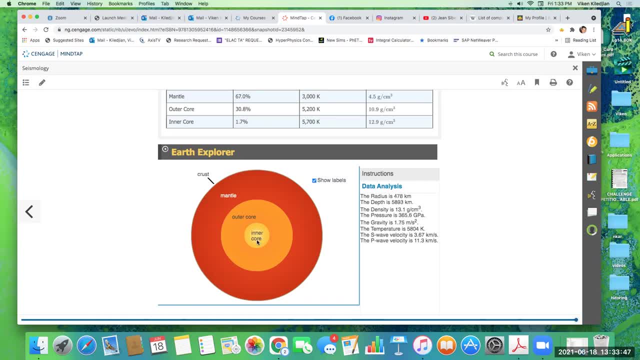 It's still going up And the density is going really high. So by the time you get to the center, the density is 13.1 gram per kilogram And the pressure is very, very high: 370 gigapascal. 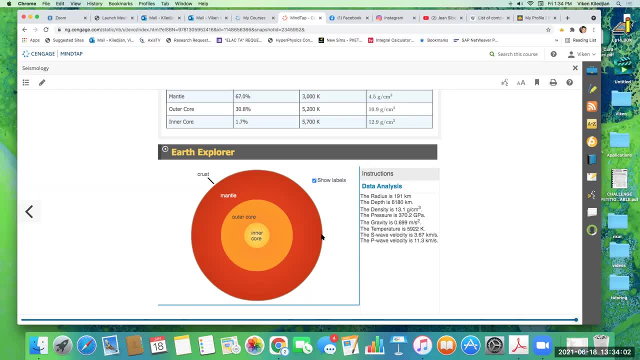 What's the pressure at the surface of the Earth? Okay, So right about, let's see here. Yeah, if I go to the surface, Yeah, about 1.31 gigapascal right there. That's the pressure. That's the pressure that we feel at atmospheric sea level pressure. 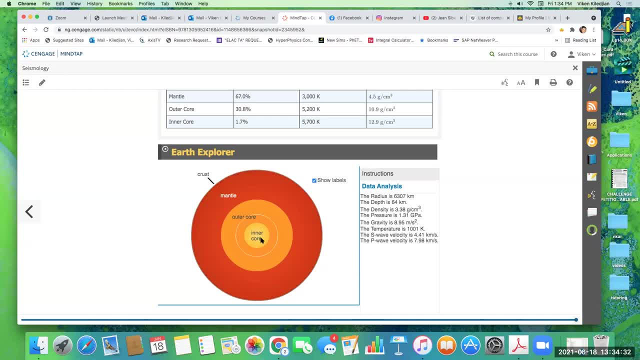 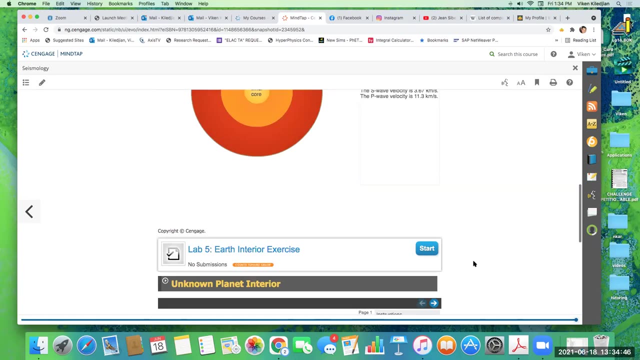 So of course, as you go down, the pressure is going to increase until you get to 365 times the pressure at sea level. So those are kind of interesting things you can see as you are pressing this Earth's interior exercise. Okay, 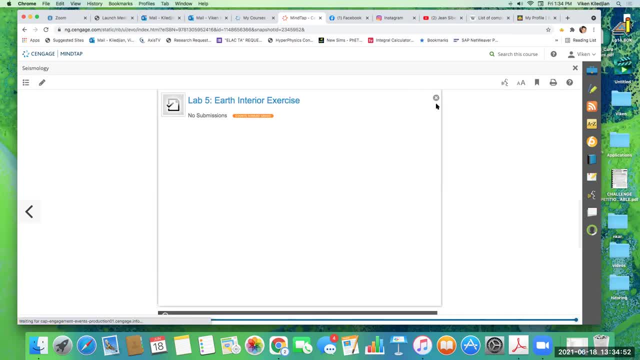 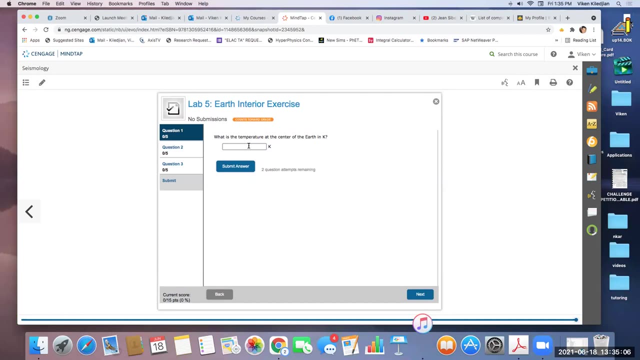 This is the first exercise. Okay, so this one. since there's only three questions, take a picture of each one. Take a picture of each of the questions and what answer you got. What is the temperature at the center of the Earth? 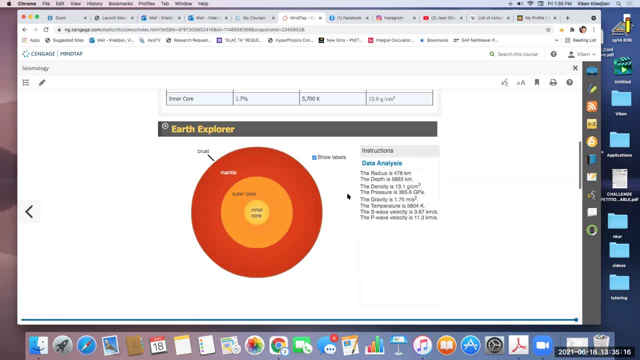 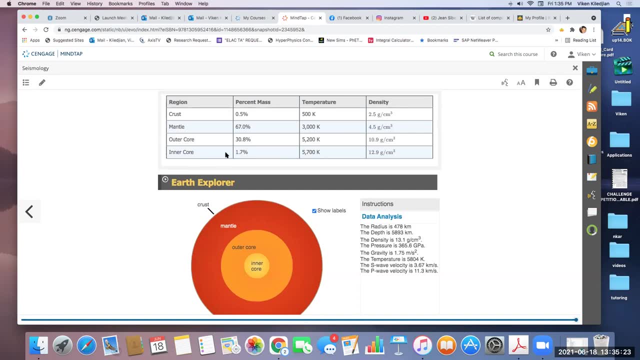 Okay, so what would that be? So then you would go: You can't really use this number, The inner core 5700.. You can't really use that because that's the average temperature of the inner core. You see, But it varies. 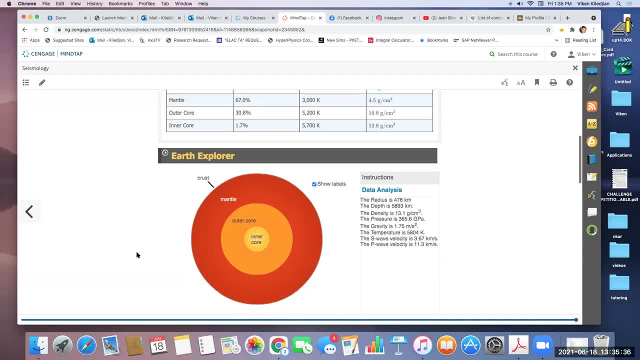 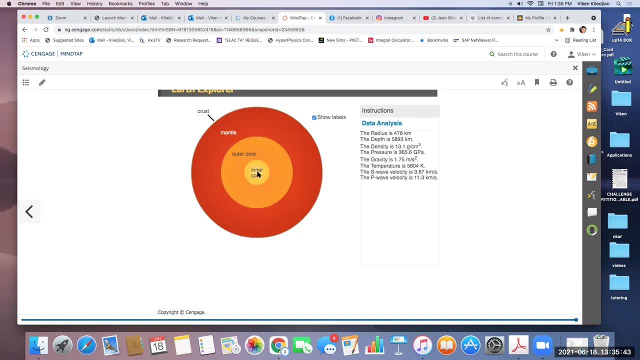 So if I were to find out the exact center of the Earth, then I would have to go click, So like go click Right there at the center And whatever answer that you get- 5987, right Does it show? 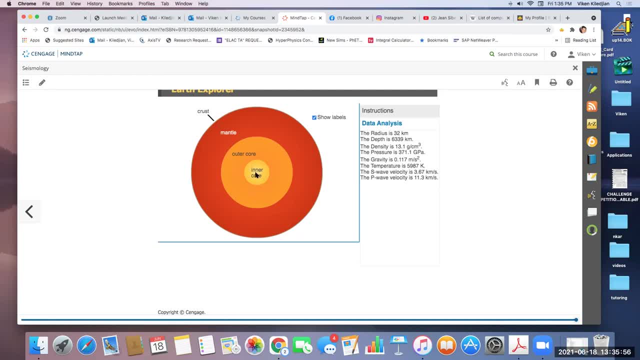 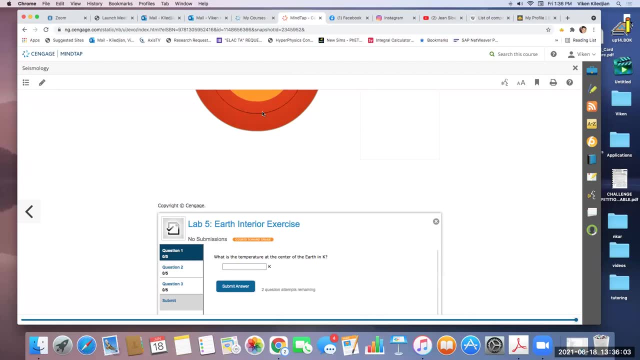 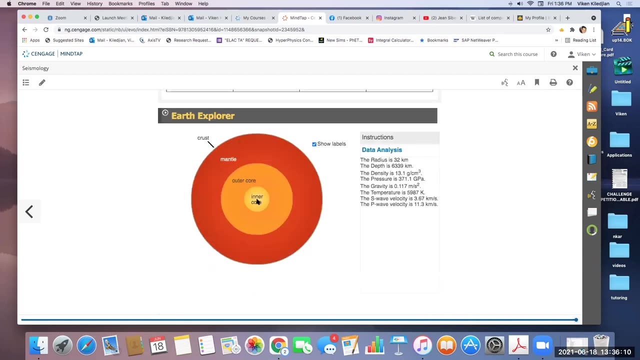 Does it show. So then you take, Take a picture of that. So if answering these questions requires you to go and do something here, then you also need to document that. So you got to go here and go and then click: Yeah, it looks like it's 5987, but you might- each person might- get something different. 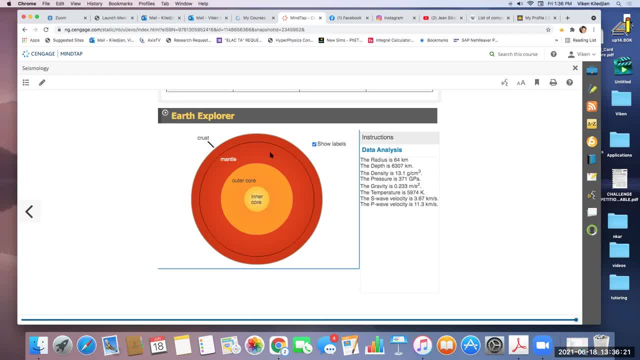 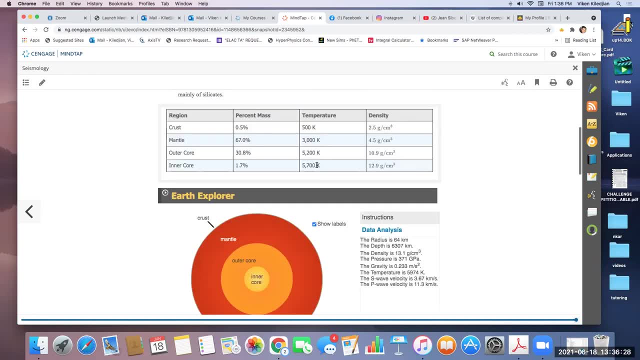 5974 I'm getting now, So take a picture of the- also this picture- And then show Showing the, the right side, 5974, notice that that's more than the average temperature of the inner core, because that's only the average, you see. 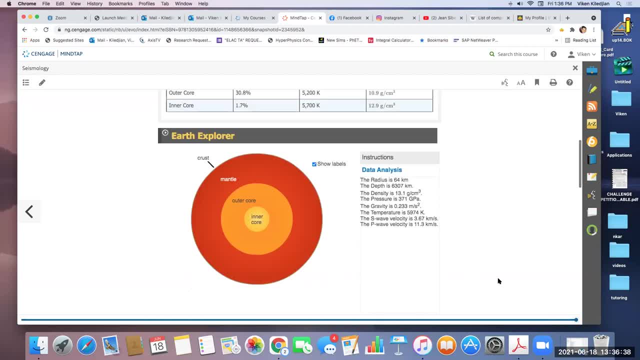 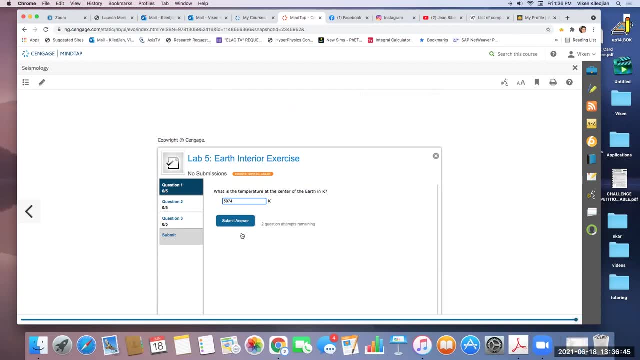 So you should get something higher than that. And then, once you put that answer here, let's say, if I were to put it, Okay, then you would take a picture of that. And then you go to question two: Approval: Approximately how thick is the mantle in kilometers? 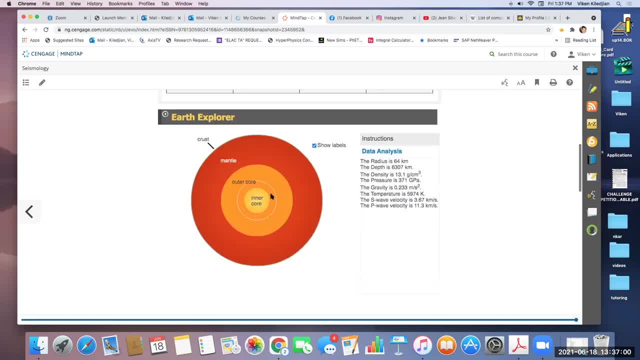 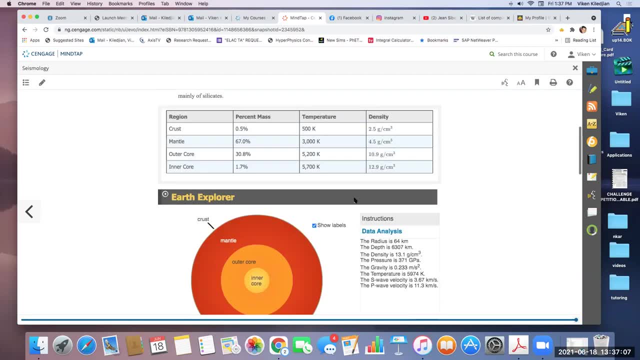 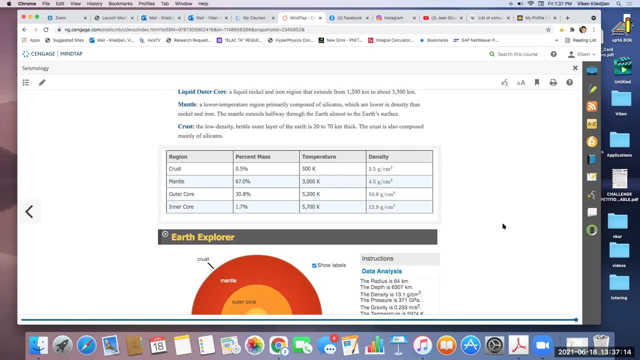 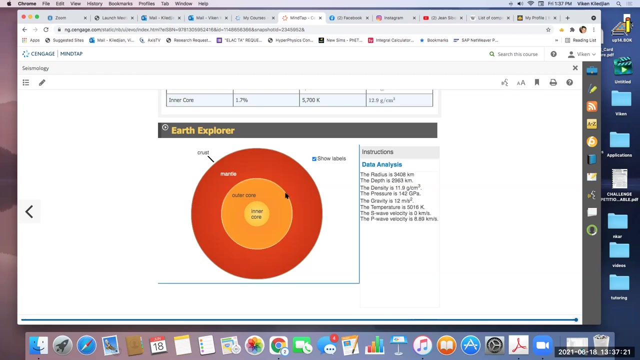 So that means they want to know from the mantle, from here all the way to here, What is that? So how would you do that, Can you? Well, the information here you can't use, Let's see. Maybe you can go take a picture of that like this, right? 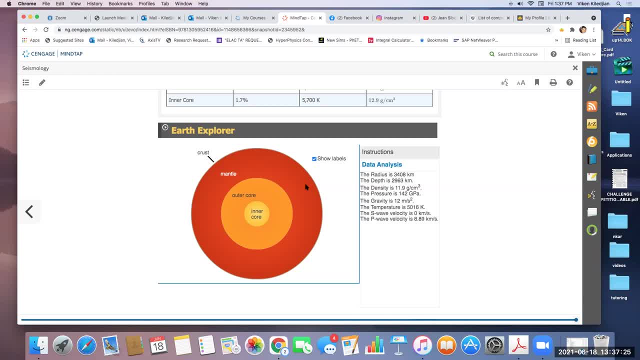 And then showing the, Your radius. let's see here, right there, and then go all the way to here, show the radius and then subtract them. you see, or you could use the depth. the depth is, the depth is measuring from the top to the where, where you click right. 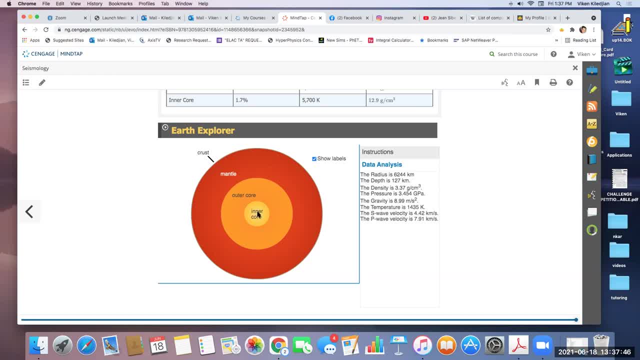 And the radius is measuring from the center to where you click. But if I want to know the thickness of something from here to here, right Then, well, you can do. if I want to know the thickness of something from here to here, you could either use the radius of that point and the radius of that point and subtract them, or you could use the depth and subtract them. 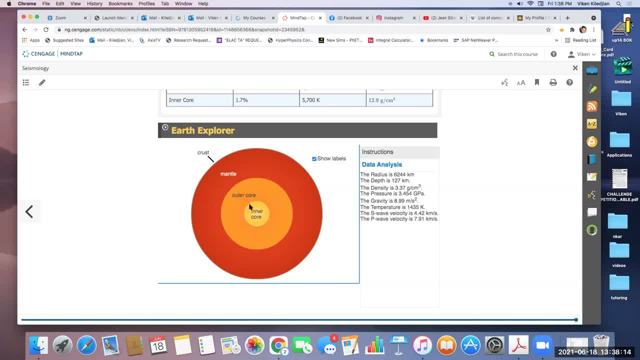 I think you should get the same thing. So then you have two pictures to take over there, one here and then one all the way out here. Try not to include the crust Like right there, maybe a little below the crust, Let's see. 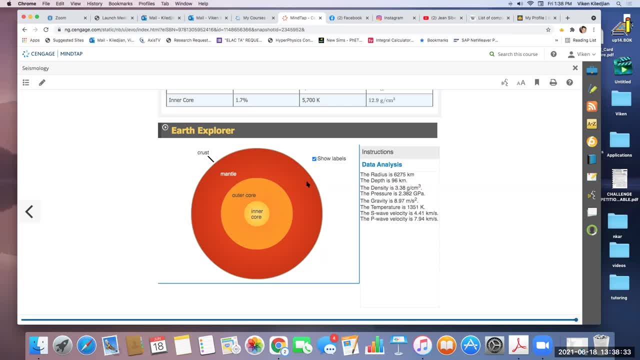 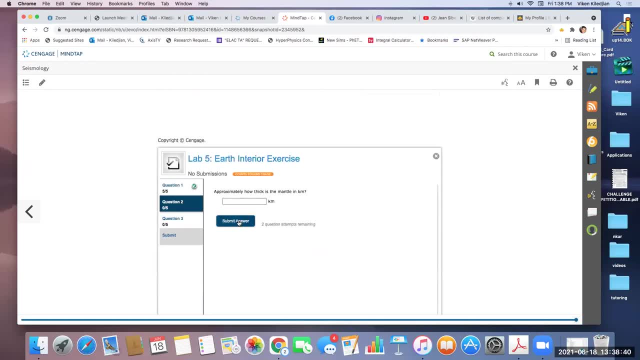 Yeah, So then you were to subtract those two. that would give you the mantle, And then you would put the answer here: submit. So how many pictures would that be? Two for these- showing the radius or the depth and then um, and then take the difference and put it here. 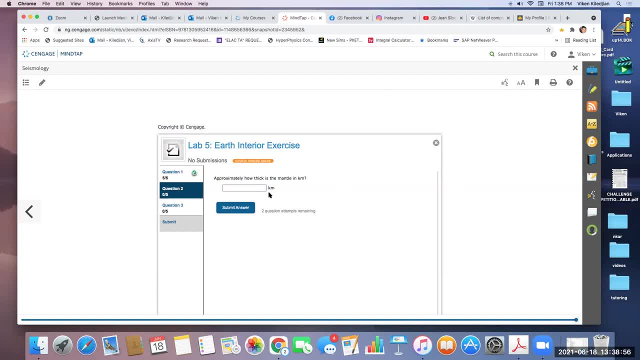 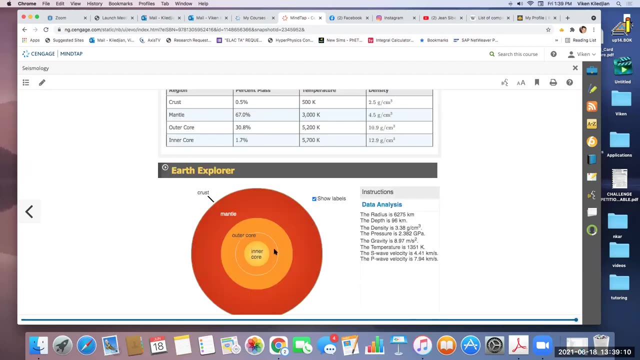 And then Click submit And then the answer. So basically one of this and the two of those, And then question three: approximately how much mass is in the liquid outer core? So how would you do that one Liquid outer core, Uh, that one. we just, we might just be able to use this one. 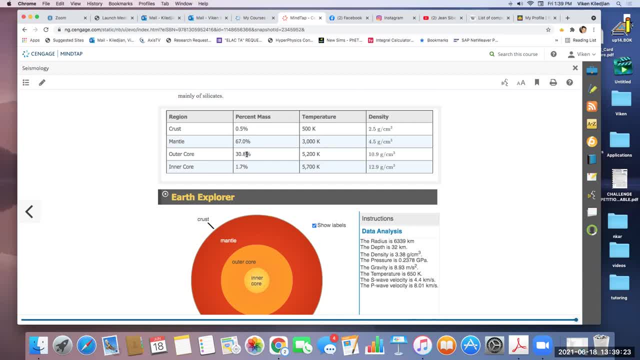 Uh, the liquid outer, the outer core. It says 30.8% of the mass of the earth. Uh, I think that's the best way to do that: Use this and then find online what the mass of the earth is. 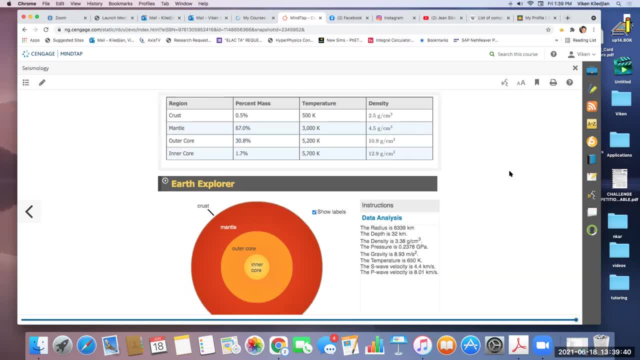 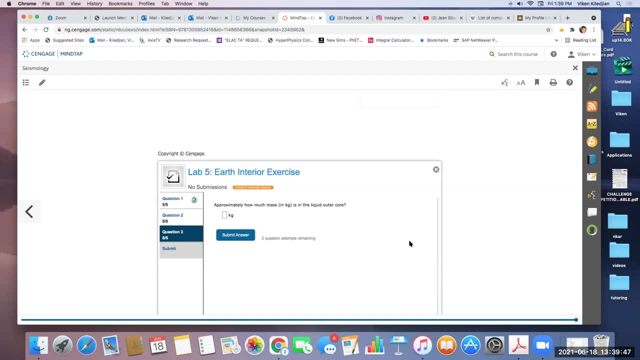 Um, so just do a Google search. So do a Google search for that one- what the total mass of the earth is- and then take a picture of your Google search, So the number that came out. So do a Google search: What is the mass of the earth? 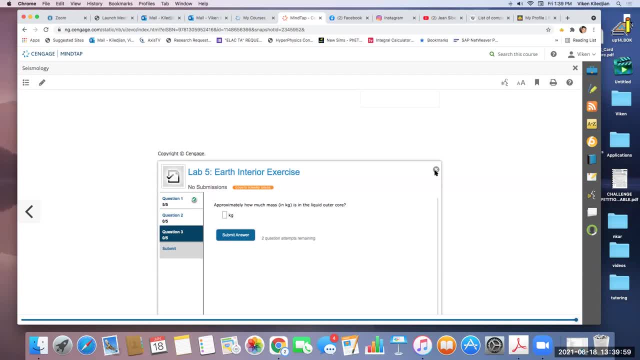 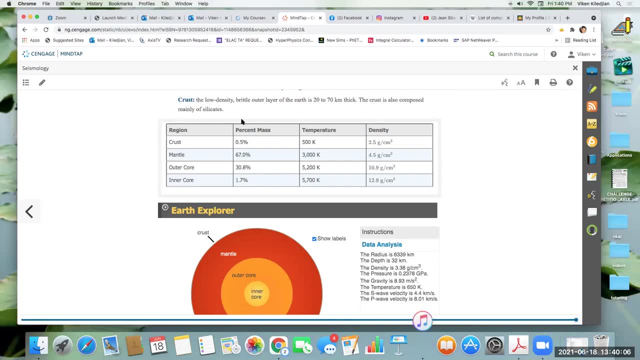 Take a picture of that, Then use this percentage. Uh, take a picture of this part, Like this Right, Showing that, um, the percent mass by breakdown You see. So then argue that if I want to find the mass of the outer core, I'm going to take 30.8%. 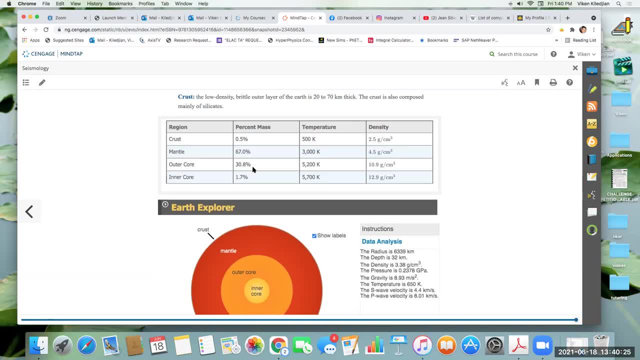 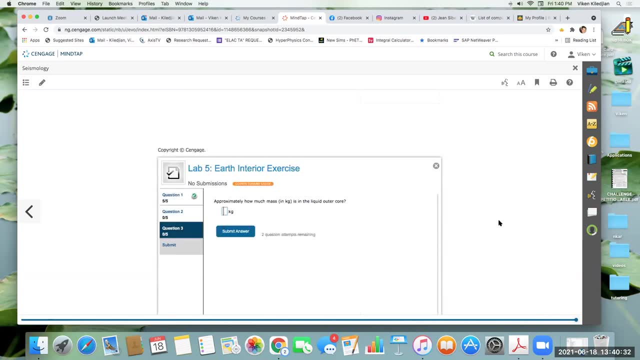 Uh, So I'm going to take 30.8% of whatever search you did- the mass of the earth on Google, then multiply them and then, uh, put the answer here. Okay, So for that one, show your work. I know it's a simple, short work to show, but just show the math. sort of imagine that someone else is reading it, an audience that's not me. 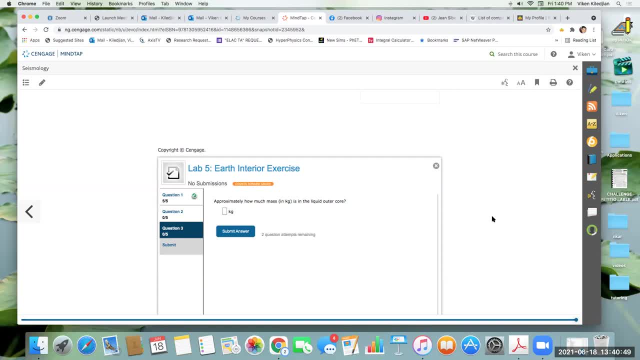 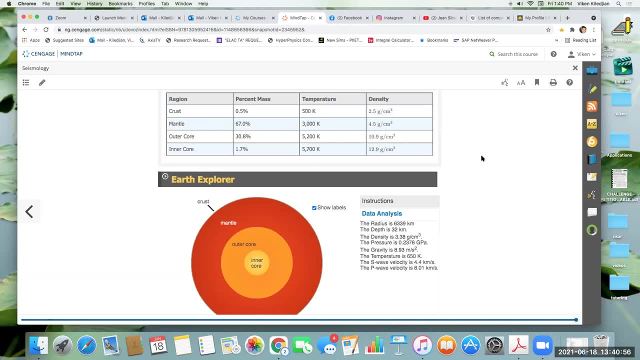 So you want to be as thorough as possible, showing how you are getting these things. Uh, I'm going to take this percent. show them the percentage. show what the mass of the earth is, then show how I'm getting the mass of the earth from that. 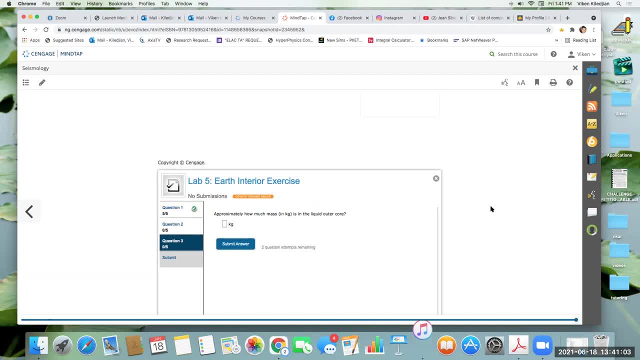 So do a- it's probably just a one-step thing where you could show how to get the mass of just the liquid core, then put it in here and then press submit, of course, and then show that your answer was correct. Okay. 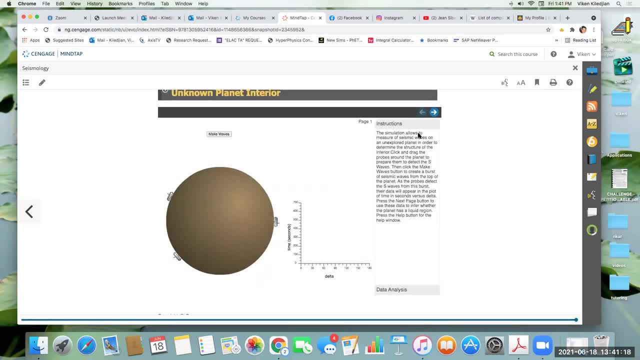 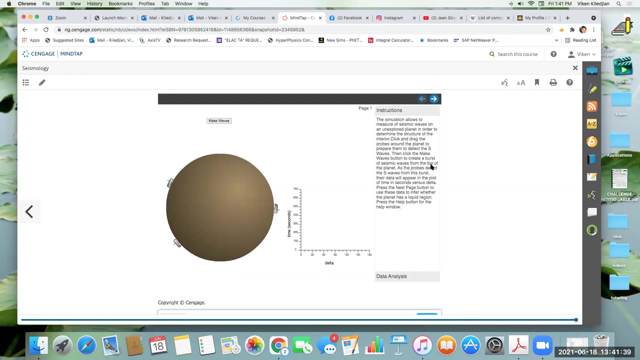 Then the next exercise. So the simulation allows the measure of seismic waves on an unexplored surface. So you start with an unexplored planet in order to determine the structure of the interior. So, uh, drag, so click and drag the probes around the planet to prepare them to detect the S-waves, then click the make waves button to create the burst of seismic waves from the top of the planet. 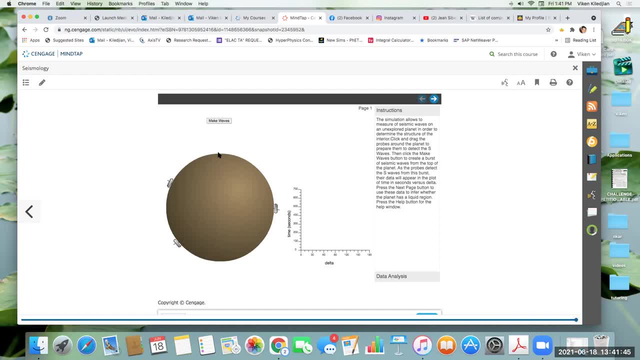 So what they're gonna do is simulate, let's say, there's a uh earthquake that happens here. as that earthquake happens, the the a dynamic is going on. Oh, this light, Yeah, caller's note: I provided this on Instagram. 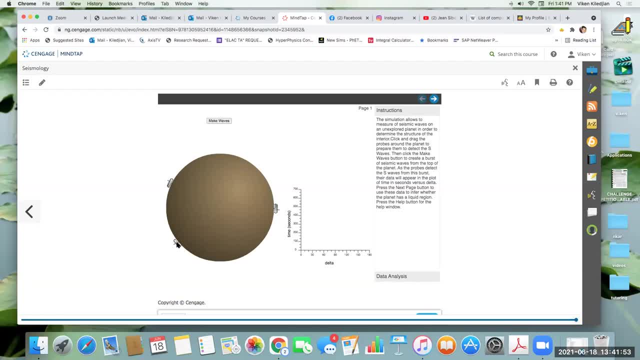 ty and P waves that go through, and then you have some random seismographs. So you see, this represents the angle. So if I put here, that means the seismograph is 180 degrees from where the earthquake is happening, you see, So if the earthquake is happening there, it's opposite. 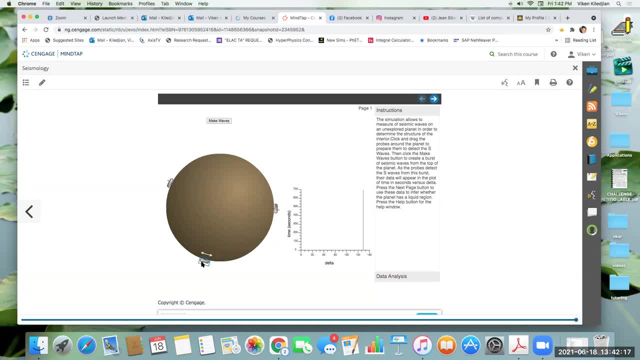 So it's 180 degrees. you see, If I put it here, it's 150 degrees. you see, Like that, So it's like this, like that, That's 150 degrees. So then I could take this, put it at a 60 degree. 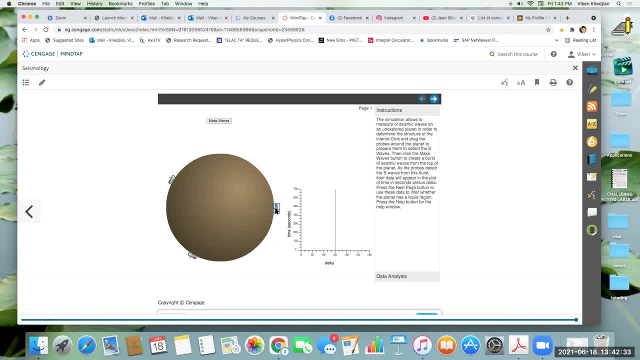 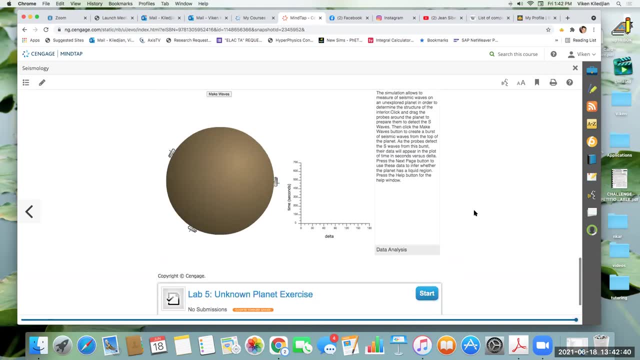 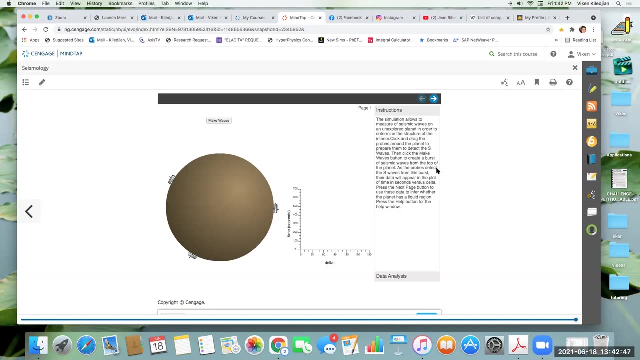 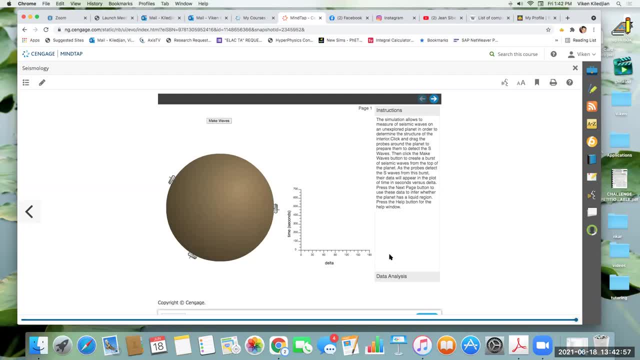 versus delta. The delta is the angle. Press the next page button to use this data to infer whether the planet has a liquid region. Press the help button for the help window. So make waves. So the only two of them detected. only two of them detected. 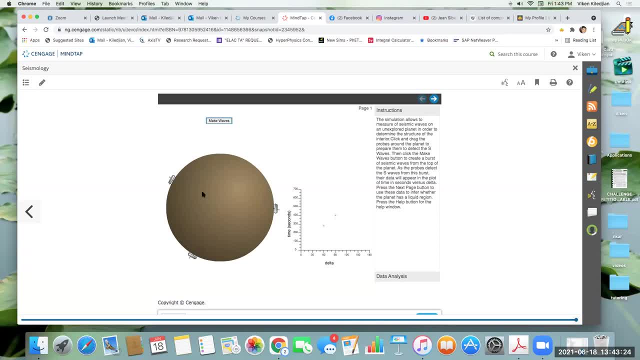 only two of them detected the S wave, So there must be. so now let's see here. Oh, okay, So now what we have to do is we have to match the data that we got. So you see, we got one data at the 60 degree mark. That means that means that means the 60 degree is this one? 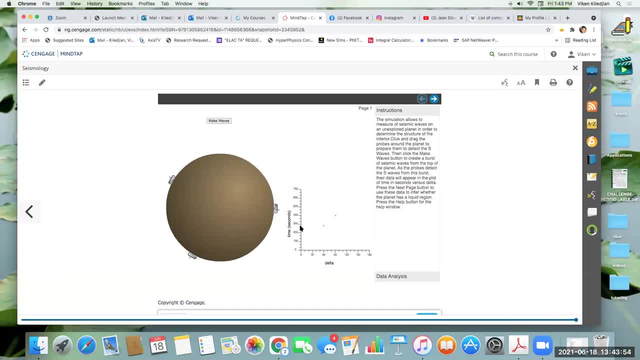 Yeah, Yeah, right here. This guy detected an S atom in about three, almost 300 seconds. you see, It took it 300 seconds, So what would that be About? five minutes to detect an a? that mean the S-wave. So that means the way it went like this: bent, bent around and then traveled. So since this is solid, 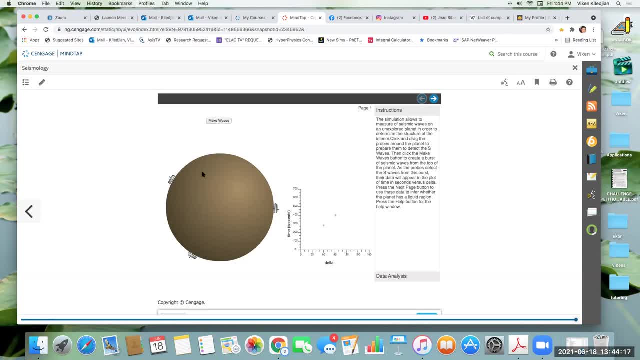 the S wave went from here, You could could travel like this and bend, bend and bend. Yeah, remember, the velocity keeps changing. so, because the velocity of the s wave is changing, it's bending, constantly, bending, bending, and then going there and it's taking it around, uh, five minutes, you see. 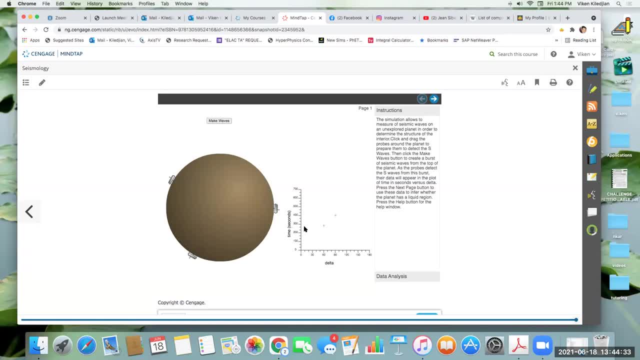 300 seconds is equivalent to five minutes. it's taking five minutes to get there. then this guy, the 90 minute guy, the 90 degree guy, is going like this and then bending, bending, bending, bending, and then it's going there and then it's taking it, uh, around 400 seconds. so that's about seven minutes. 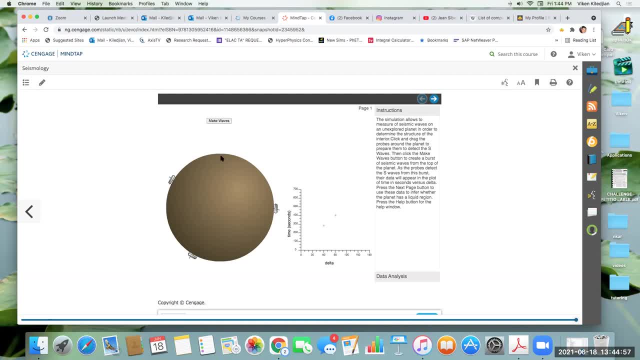 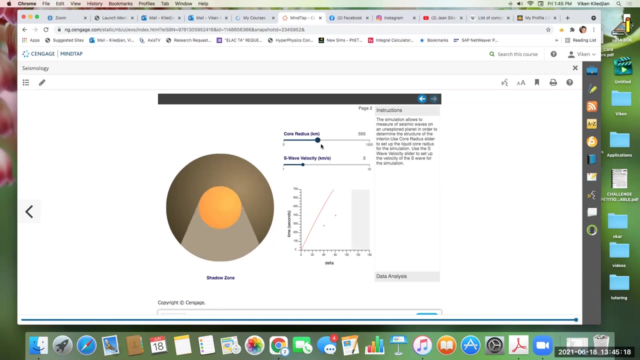 seven minutes for this detector to observe that earthquake. this guy is never observing it. nothing, no observation. so what does that mean? well, there must be a liquid, huge liquid core here you see. so let's see here, if i increase the liquid core also, i gotta play around with the s wave velocity. that the average s wave velocity, so the average. 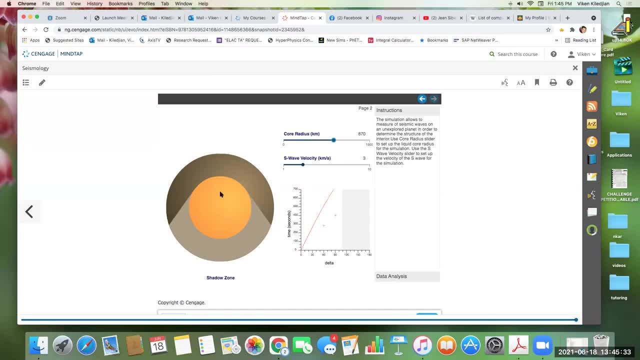 s wave velocity as it's going from here to here. you see, so we know that this guy observed it. so the liquid core can't be this big. you see what i mean? because then, if the liquid core was this big, neither this seismograph nor that seismograph can be this big. so the liquid core can't be this big. 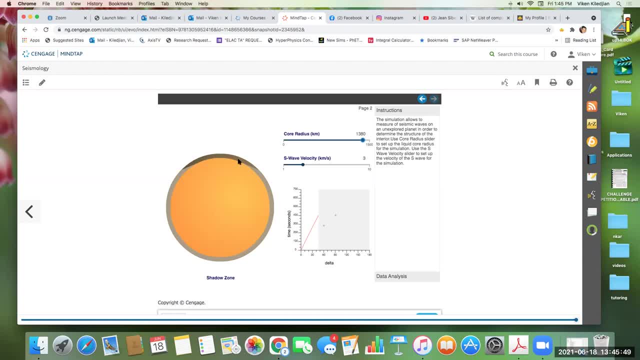 so the seismograph would have observed it, only these seismographs from here to here would have observed it. so the liquid core can't be that big. so it's probably like: this right can't be bigger than it, can't be too much bigger than that, because this guy observed it and then that guy observed it. 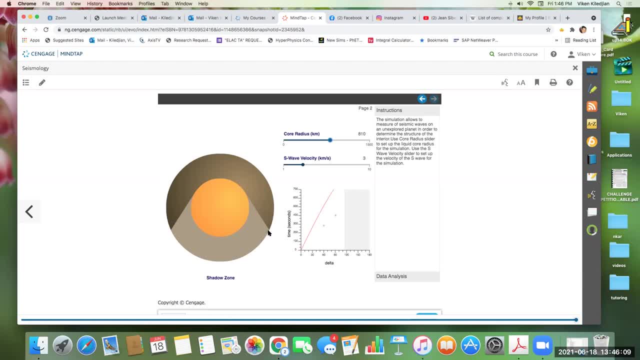 you see. so now, what this is telling you here is that any seismographs from here to here wouldn't be able to observe the s wave you see from here to here. so then the s wave velocity. now i gotta play around with it. does it fit that data? 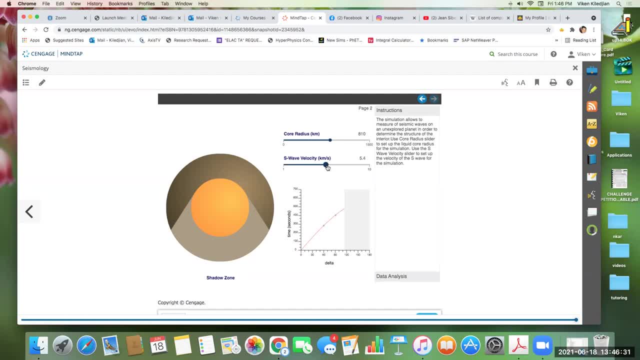 yeah, right there. so that means the average s wave velocity while it's traveling through this medium is, uh, the average s wave velocity is um 5.4 kilometers per second. the core radius: we can't really tell what it is, because if i make the core radius bigger, 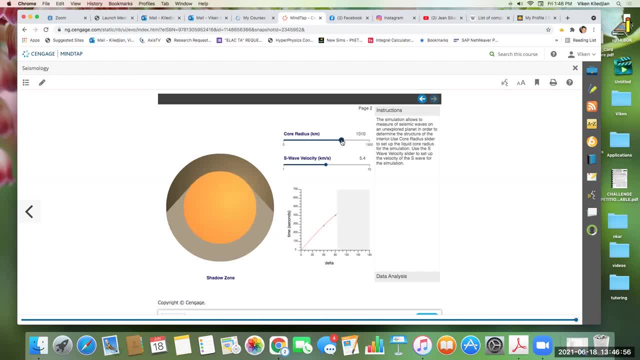 it still fits the data. so how big can it be? it can possibly be this big, you see, but that gives me a lot of room for error for the core radius right. so it could be this small or it could be this big, you see, but at least the s-ray. 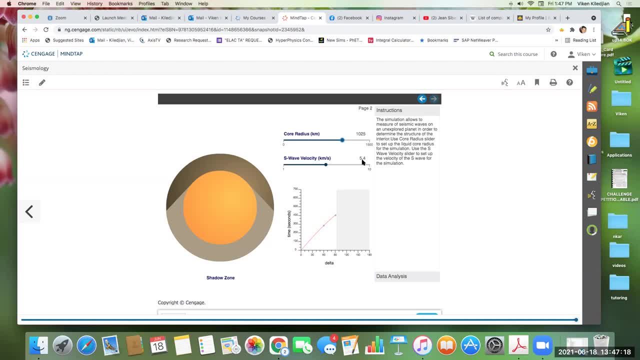 velocity. uh, i have, i have it down very sp, miraculous for sure. so i can say for sure: the s-ray velocity has an average velocity of 5.4, but the core radius can be as small as zero or as big as thousand-something. so where should i have put? 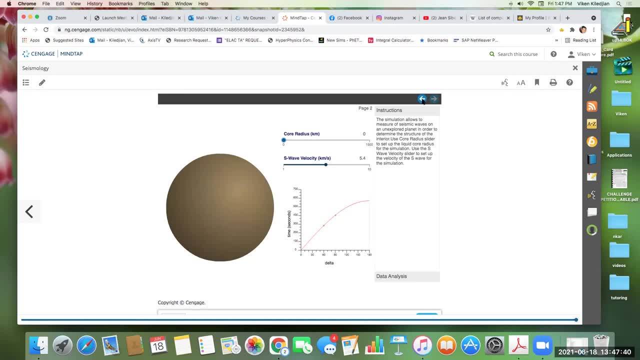 my third uh seismograph, then maybe i should have put it at more well. the best thing to do to the do is have more seismographs. of course, have one here, have one here, have one here and have one here, so on, right, but if i'm only have three seismographs around the earth, i think 180 degrees- 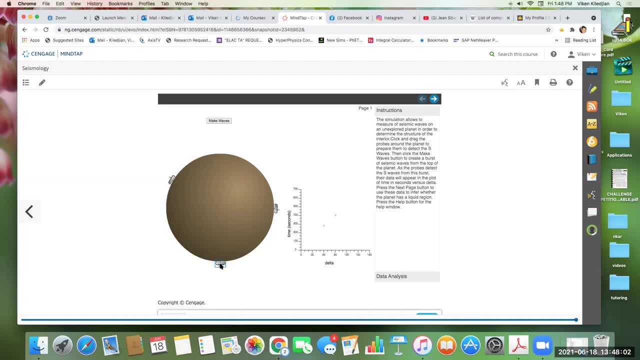 was not advantageous for me, because 184 doesn't give me too much information. probably i need one at 60, 90 and then maybe 150 would have been good. now let's repeat: okay, it's probably still not that well, the 60 guys getting it and the 90 guys getting it. 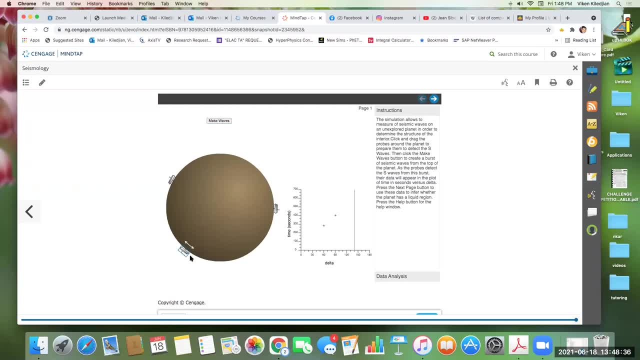 let's see here. maybe keep moving it, okay. ah, you see that now the third guy got it. this guy got it at a hundred and something degrees now, so maybe what i should do is keep moving it back down until i don't get it. oh, and go down a little bit more. 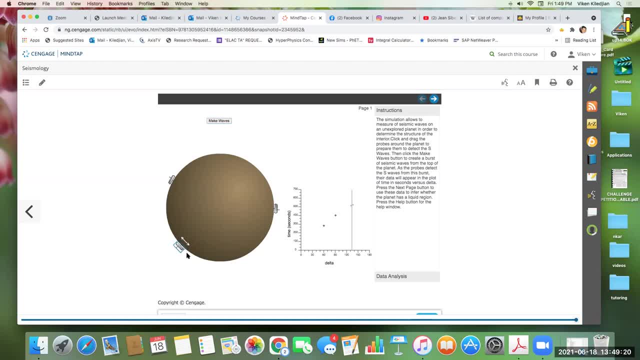 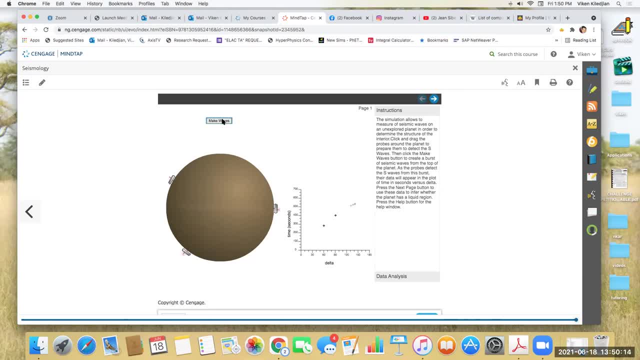 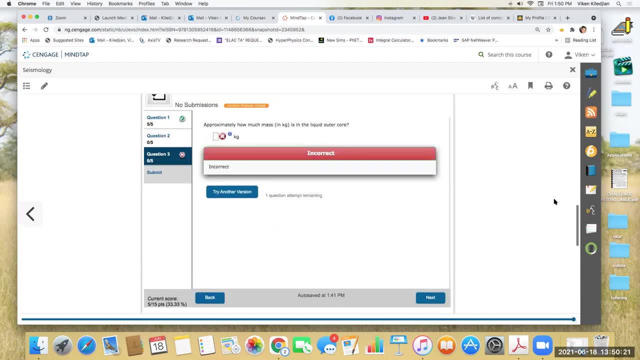 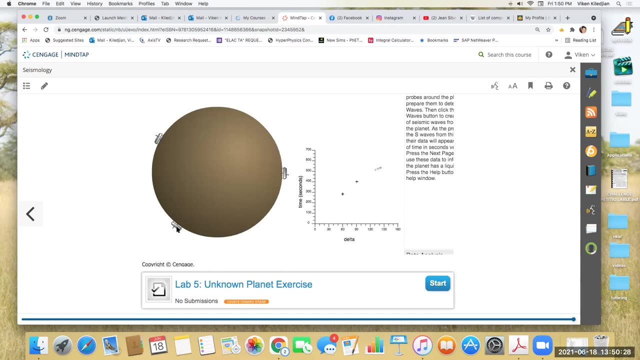 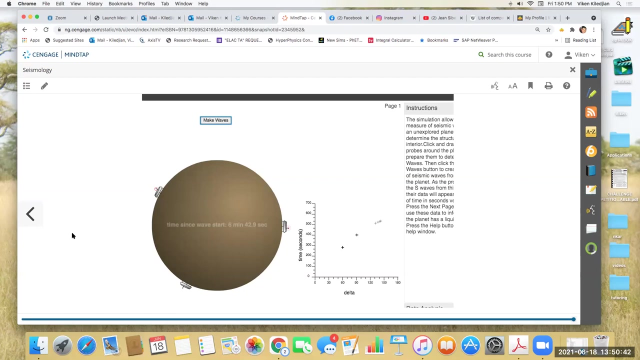 this is a good one. this is a good one. this is how we find out the size of the liquid core. oh, i got it, so zoom in on that. okay, maybe one more. okay, i think that was the very last edge. they got it okay. so then i'm gonna go. 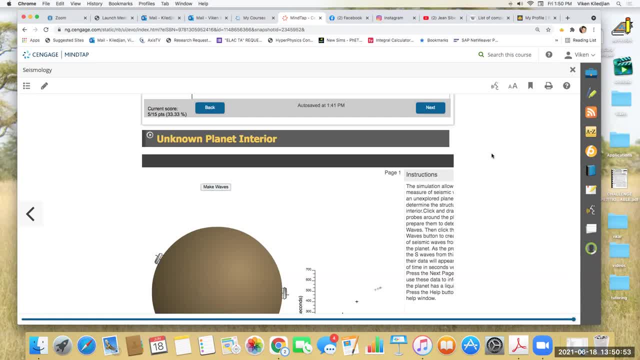 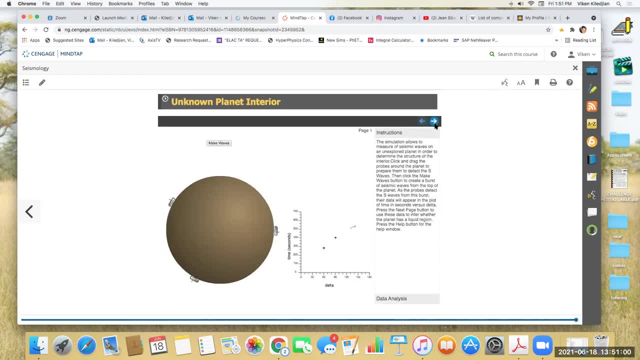 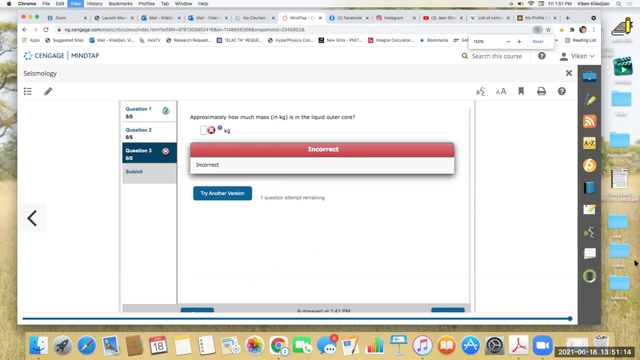 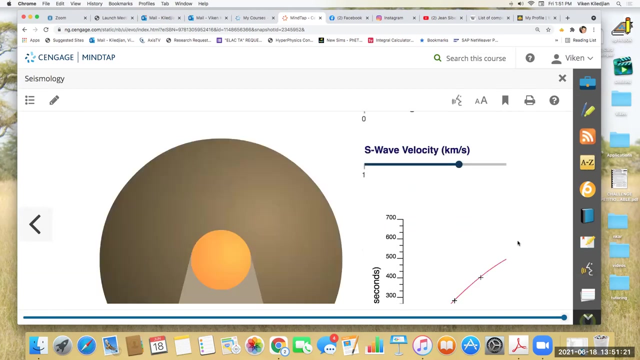 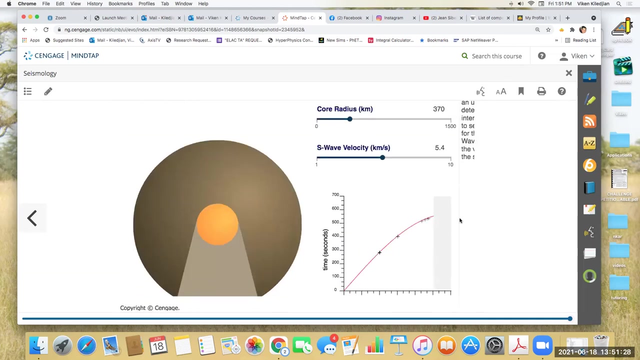 oh, oh, zoom out. okay with the velocity of 5.4. let me see, i'm still feeling all the day. now let's go the core radius. so now, now i'm gonna zoom in on the core radius, I'm going to zoom in, zoom out a bit. Okay. so now I can play around with the S wave velocity. 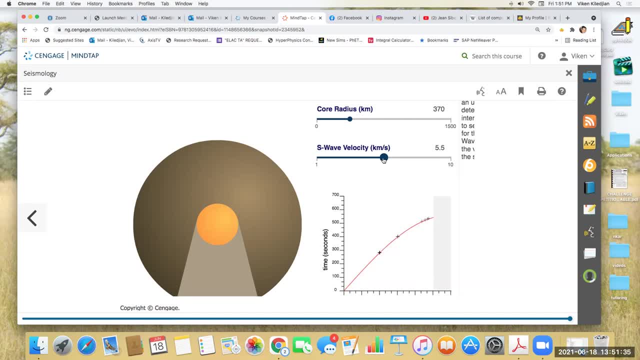 a little bit more, I also get a better measurement of the S wave now. See right, Okay, about 5.4 is still the average, but it looks like it should be 5.4, something 5.45 or something like that. Like I said, either one 5.4 or 5.5.. Now what's the size of the core? 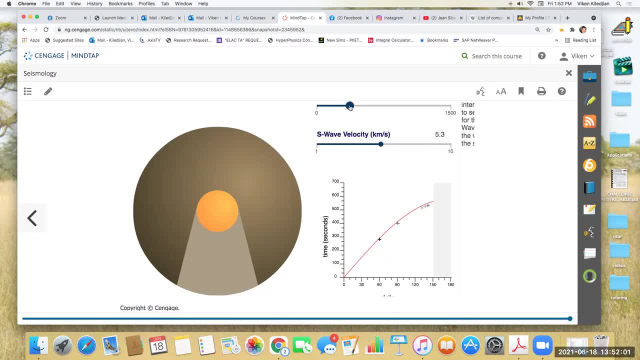 What I'm going to do is say, make the core go bigger until the last person, the last seismograph to get the S wave is that guy right there, You see. So that means any seismograph from here to here would not receive the earthquake from that portion. You see. So I think that's the. 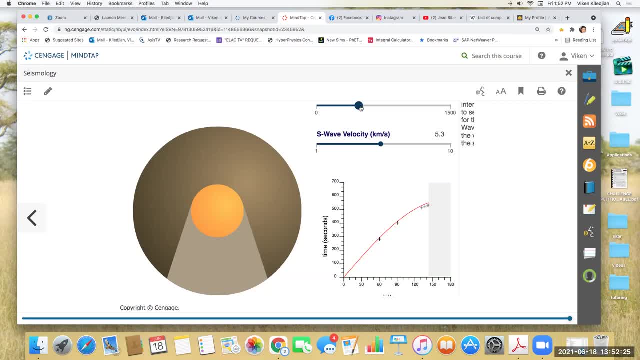 wait, what happened to the graph? Oh, I think when I hold on, Let's see 5.4.. I think this one is a better fit right there: 5.5.. So now, let's go right there, Okay, so now. 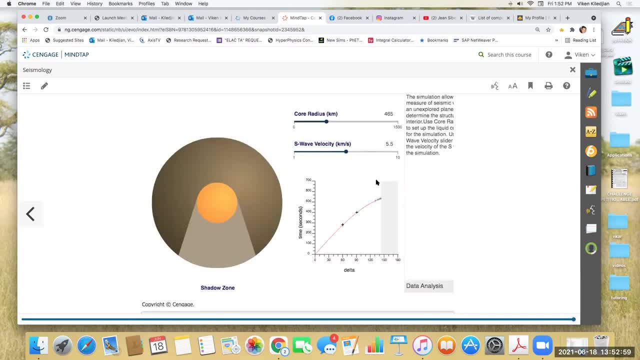 okay, so now you could take the picture of that, showing all the seismographs that you have right here, And it shows the angle of the first one is 60 degrees, 90 degrees and all the other ones you used Like that, like that, until you got the last. 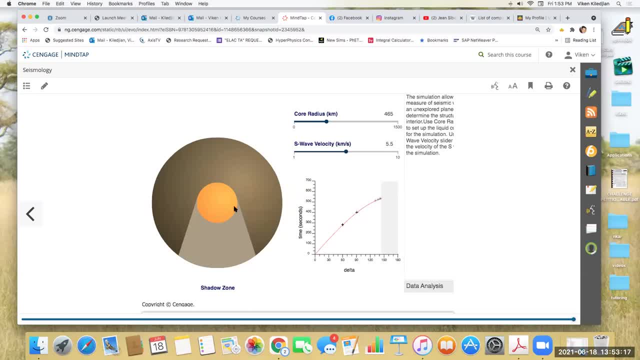 one is about 135 degrees And then it shows the core radius is 400, and that's the core, the liquid core. Now the solid core is going to be inside of it, but we're focusing. we're focusing on the liquid core, You see. So the solid, 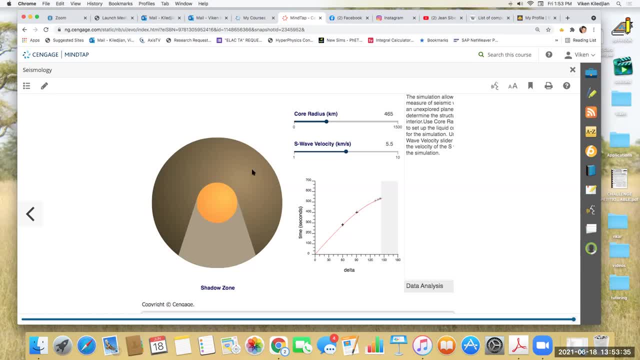 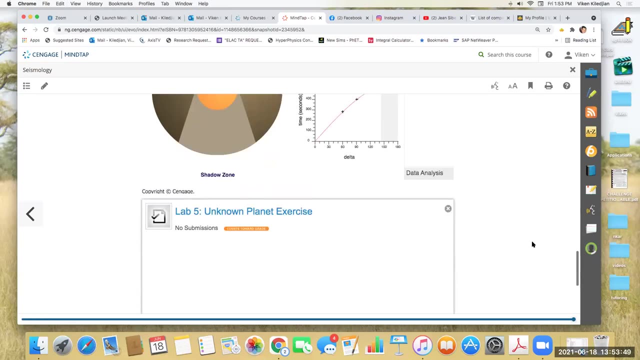 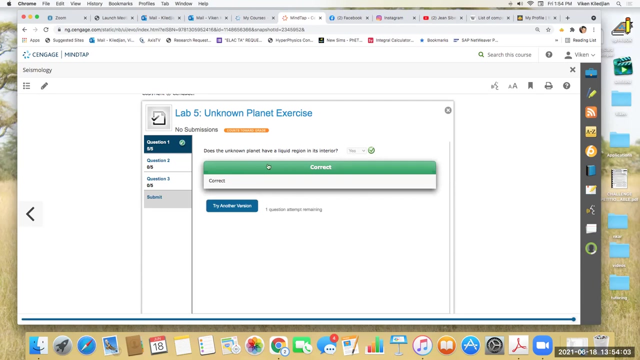 is going to be right there. So this one actually has a small liquid core, this planet, It's not that big. So does the unknown planet have a liquid region in its interior? You could say: yes, Correct, Okay, Now this one again. take a picture of each one. This one is just a yes or no, so nothing else to 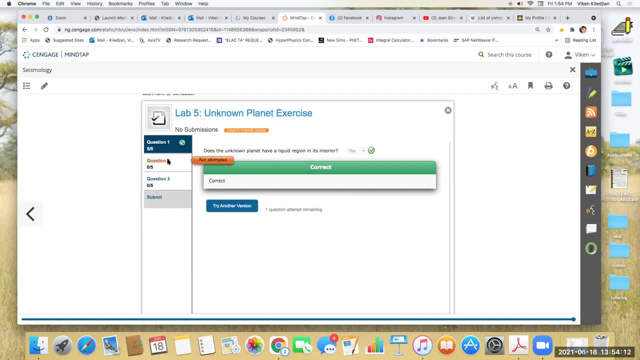 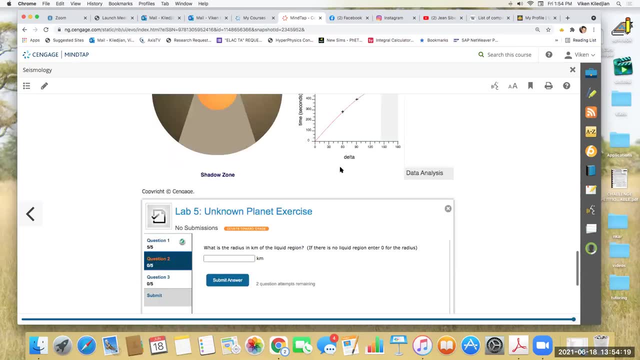 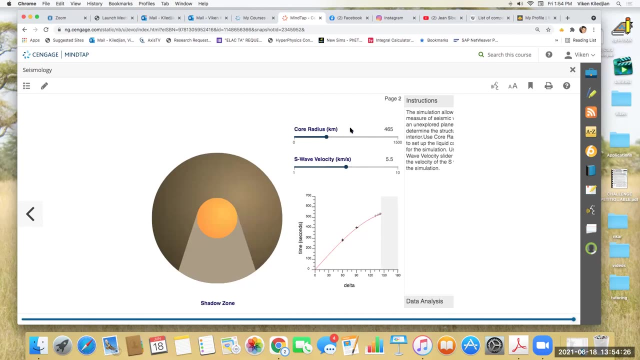 show for that. So yes, What is the radius in kilometers of the liquid region? So then you would- that's where this picture would come in. You would show this picture showing the S-wave velocity and showing the liquid core and then actually showing the size of the liquid core. 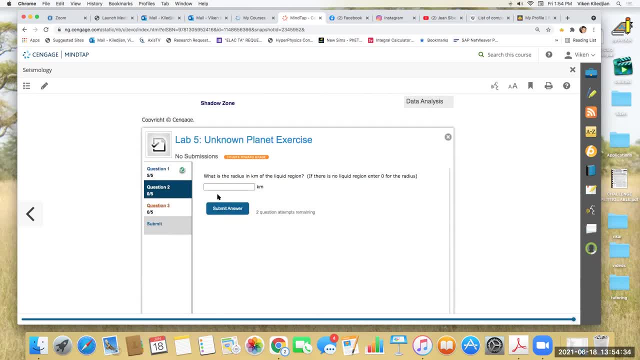 Really nice. Set up here And then submit your answer. Then the question three: what is the S-wave velocity in the planet's mantle? Well, it's all answered by that picture, You see. So then you would show a picture of each one and then go on to the next one. So let me show you a little video. 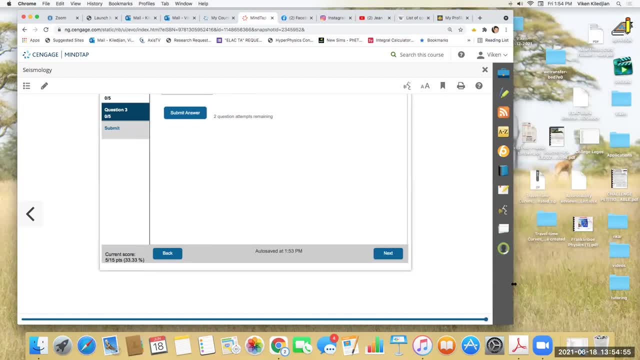 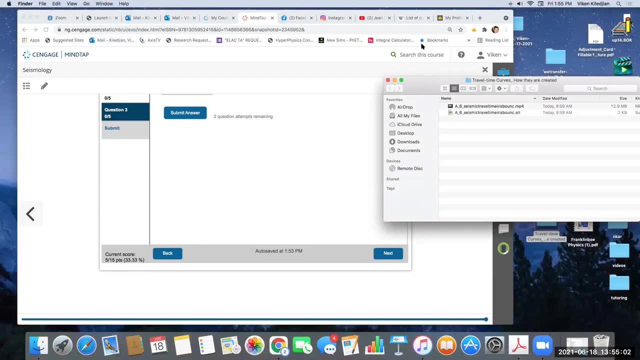 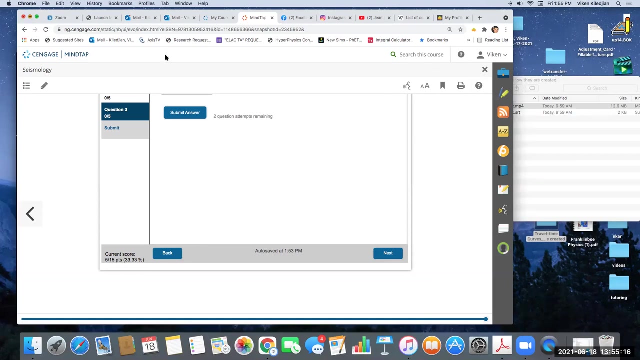 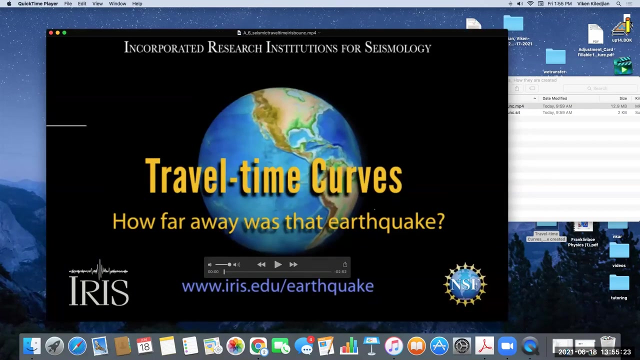 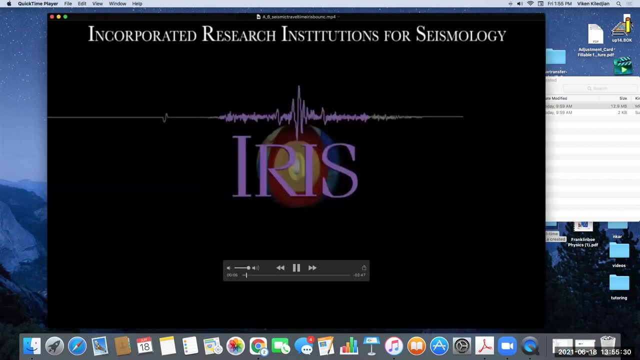 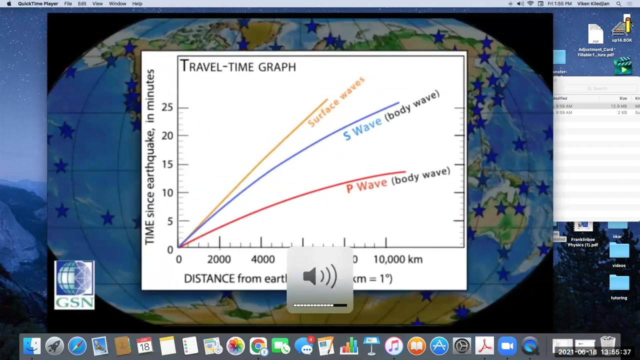 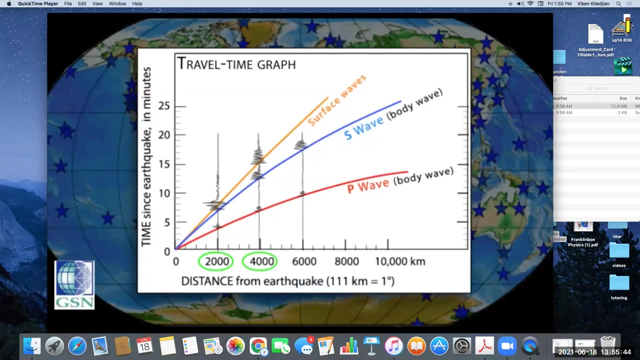 that I found about this, because this is really cool how this technology actually works. Short video This is. these are called travel time curves. 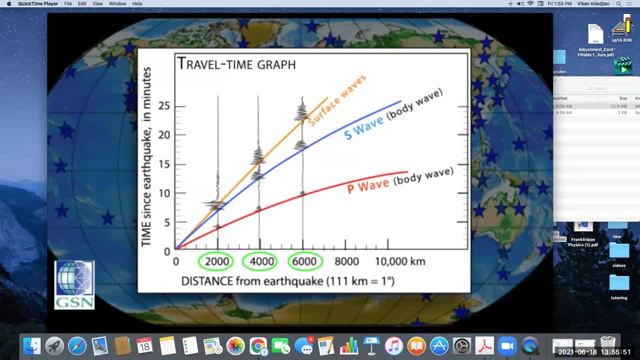 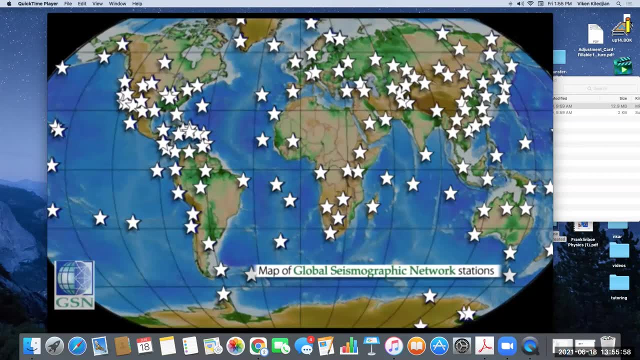 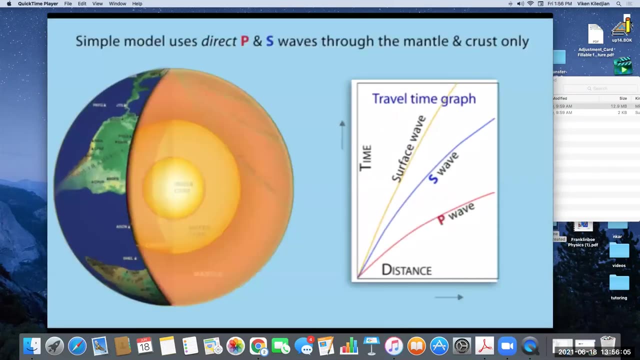 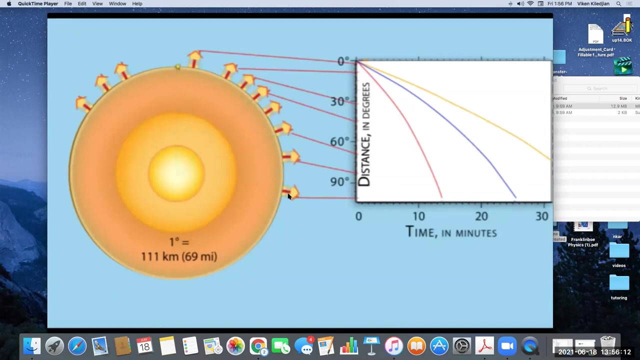 we'll use a simple graph of p? s and surface wave arrival times, while exaggerating the relative motion as the waves hit the buildings representing seismic stations. you can see here we show an earthquake near the top of the globe and graph the seismic wave arrival times to recording stations. 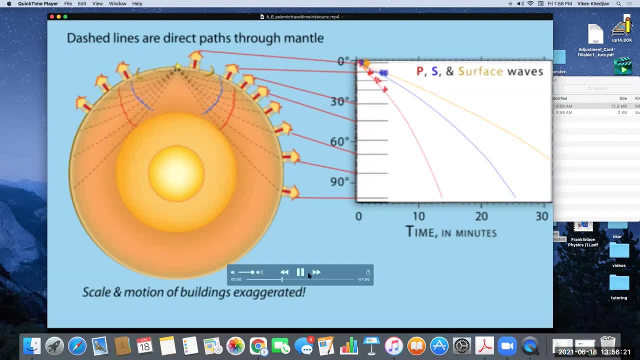 at increasing distances from the hypocenter, which is the location below the surface, so you can see her. they're doing a little bit more than what we did. they're focusing on the p wave, which is the red one. we didn't do that one, we just mainly focused on s wave. so, uh, they're focusing on the. 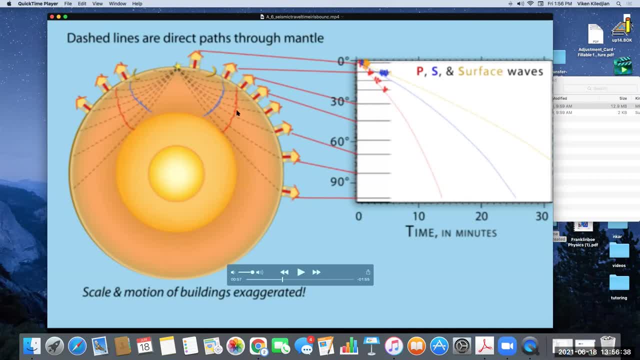 p wave and the s wave. so you see, the primary wave arrives first, then the s wave, and then they're also talking about surface waves, the waves that you get along the surface. you see, so those might arrive first, even the surface wave might arrive before the primary, just depends. but here it's. 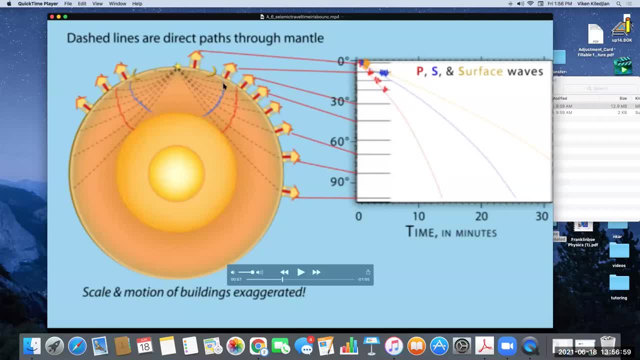 showing that the surface wave is the lagging behind the, the secondary and the primary see so lagging behind. so they, they're making three graphs, whereas we just made, uh, just, we focused just on the s wave. so we were in that lab, we were only focusing on trying to find the size of the liquid core, and that's all you need is the s ways for. 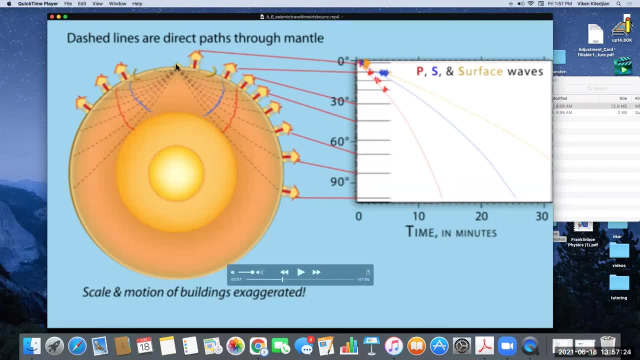 that. but if you want to find out where exactly the earthquake took place, you need to analyze all three of them: the surface, the s and the p right. okay, now let's go where the earthquake actually occurred. the y-axis shows distance from the earthquake and the x-axis shows the elapsed time since the event. 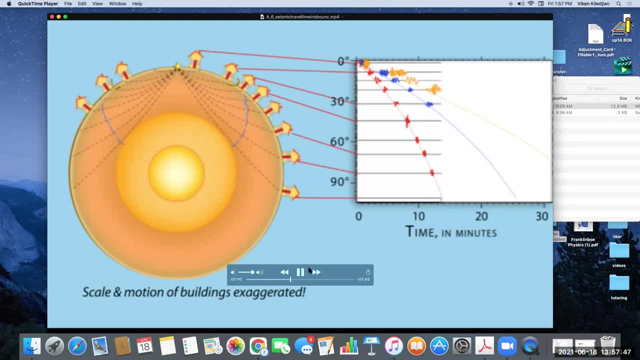 the seismograms record the arrivals of the compressional p, the shearing s and the rolling surface waves. these motions are also reflected in the motions of the buildings. seismic waves travel at different rates, so the farther a seismic wave is from an earthquake, the farther apart the p? s and surface wave arrival times will be. 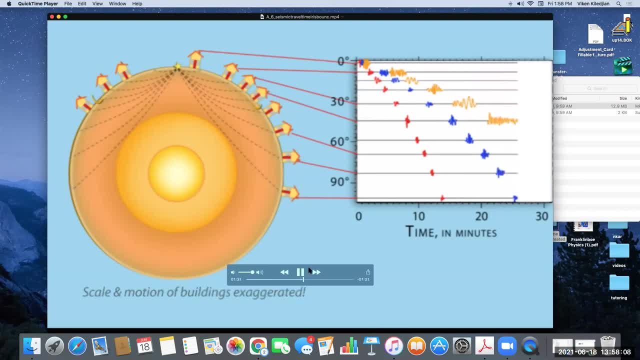 here we show only direct p and s wave paths through the mantle and crest. the final image of this animation will show more of the complexity within the earth as the waves are reflected, refracted and damp due to. so now look at how complex this is when you really want to analyze. 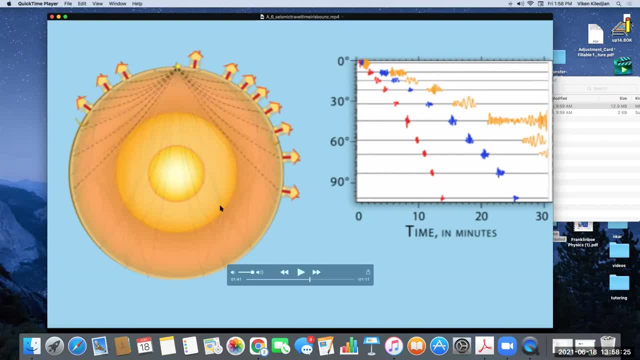 because the waves go, they bend inside the liquid core, then they bend out, coming here, then they might reflect back. if it's a p wave, uh, you might do. all of these p waves can travel the liquid core, so they might do all kinds of crazy things right, and then they, they reflect. 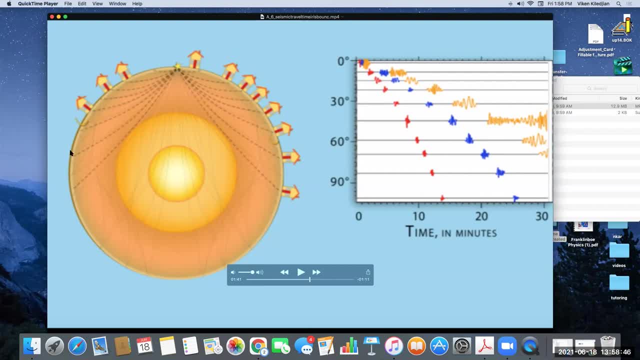 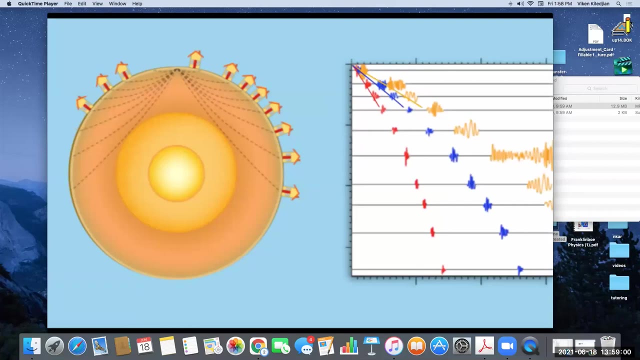 so you might get a seismic station here reading it. then it goes back and then another station here reads it, you'll see. so all kinds of complexities occur, the changes at depth connecting the waves through the effect of seismograms. the impact of seismograms creates the travel time curves that can be used. 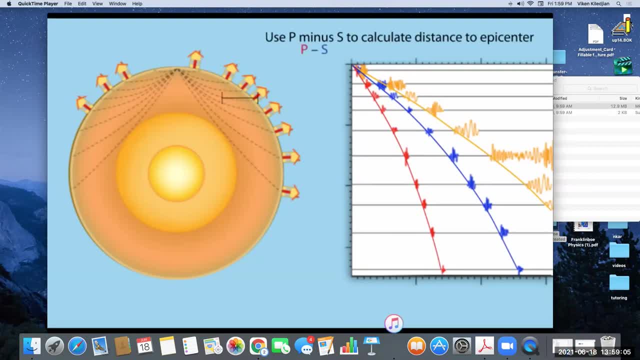 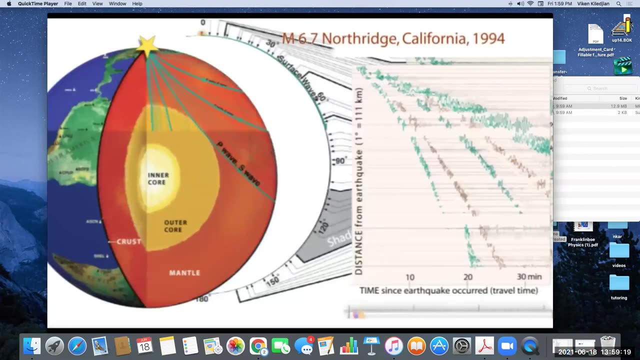 to locate earthquakes simply stated. the time difference between the arrival of the p wave and the arrival of the s wave can be used to measure the distance from the seismometer to the epicenter. this iris poster of the 1994 northridge california earthquake reveals more. 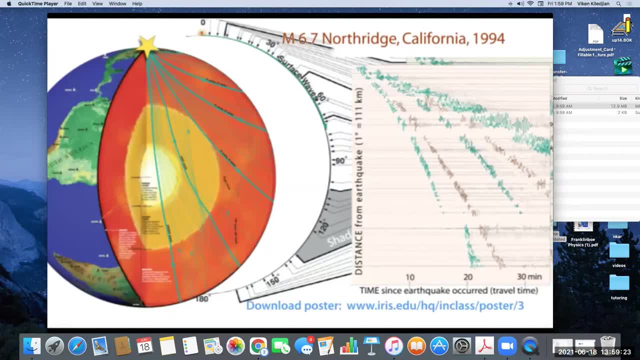 of the complexity beyond just p? s and surface waves. that earthquake killed 51 people, caused over 20 billion dollars in damage. the first wave of the seismograms from the seismometer is an example of the seismograms that can be used to locate earthquakes. 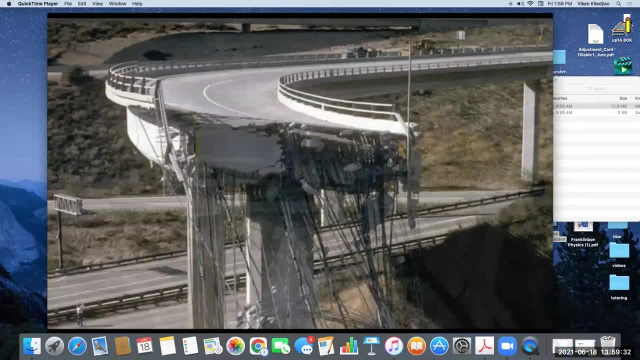 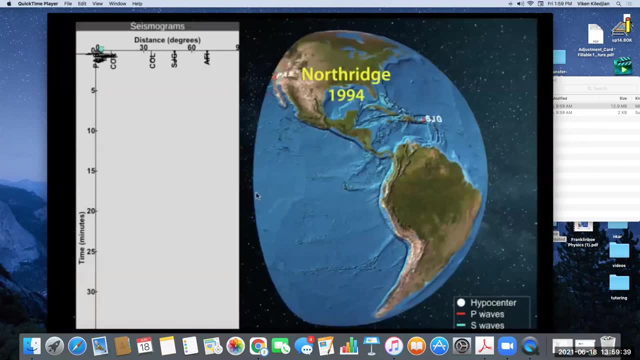 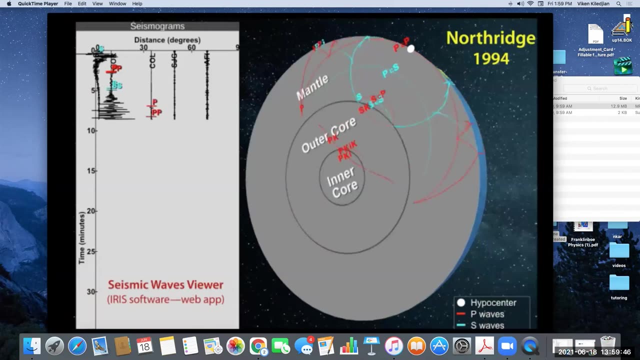 and raised the Santa Susana Mountains north of Los Angeles by 70 centimeters or 28 inches. It also created seismic waves that ricocheted throughout the Earth's interior and were recorded at geophysical observatories around the world. The paths of some of those seismic waves and the ground motion that they caused are shown on the globe. 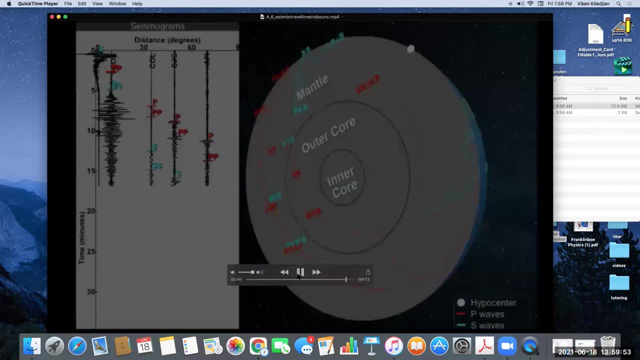 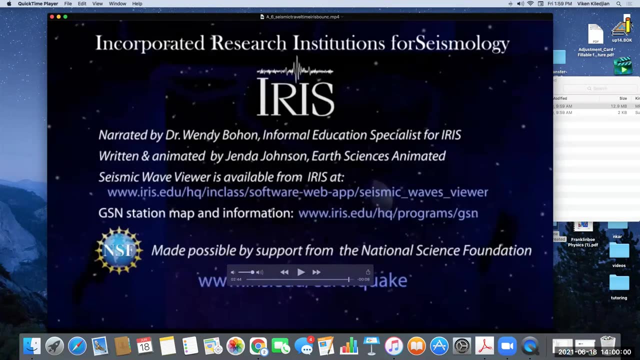 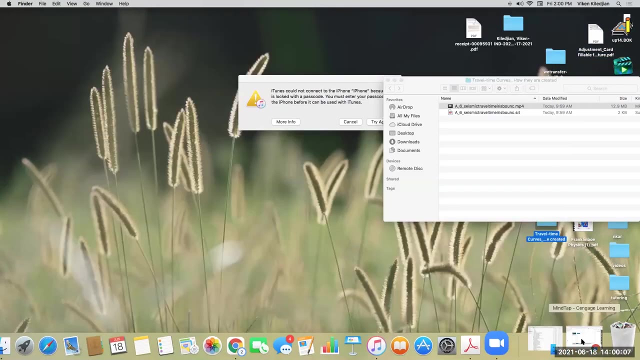 This is the Northridge earthquake that I happened to live through- Just a nightmare. So they're showing how the waves spread out for the specifically for the Northridge earthquake. So it's a nice video, that kind of similar to what we are doing here. 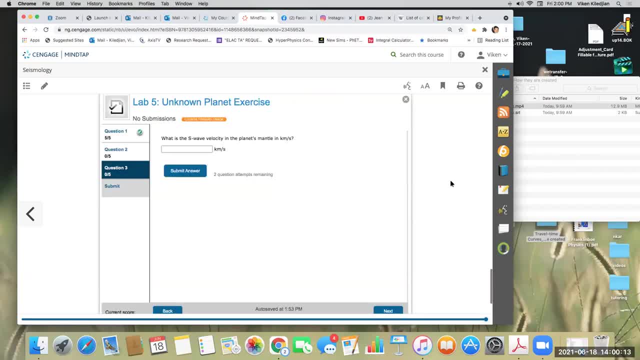 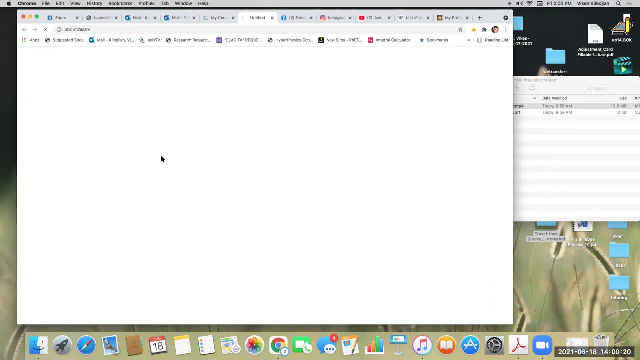 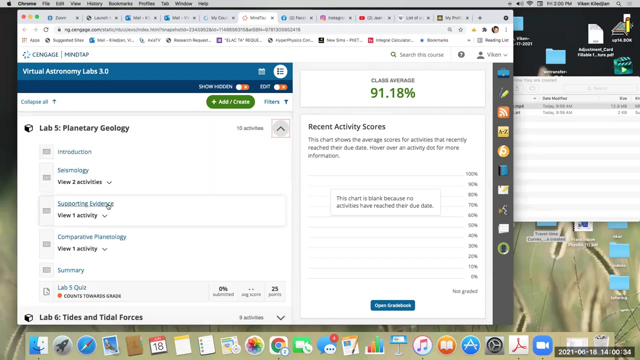 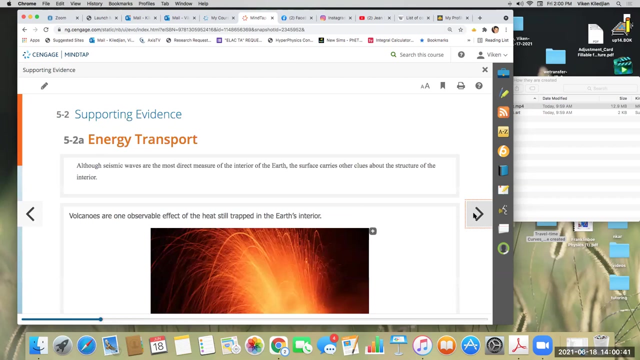 Okay. so now I think that's it for that. So we can now go to the. Okay, let's go to planetary geology. So we did the. Now let's go to supporting evidence. So all the seismic waves are the most direct measure of the interior of the Earth. 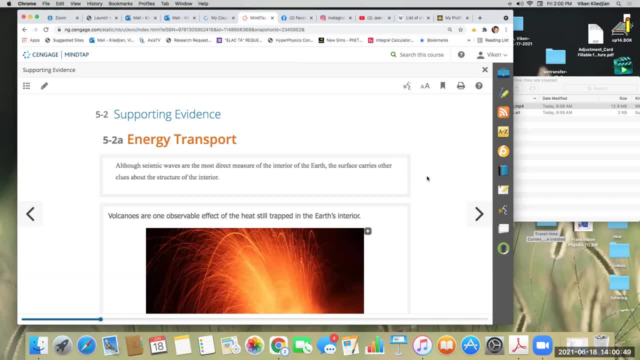 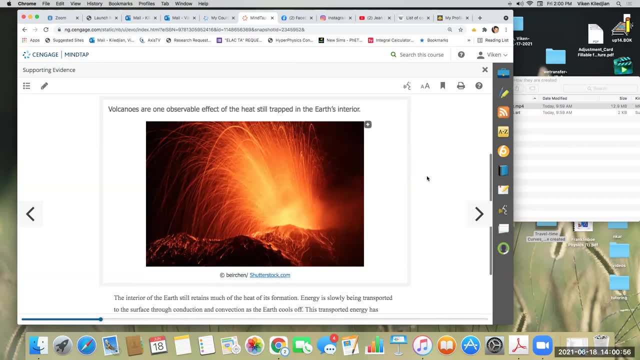 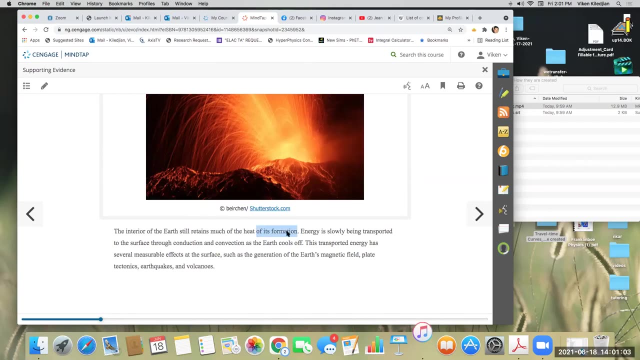 The surface carries other clues about the structure of the interior. Volcanoes are one observable effect of the heat still trapped in the Earth. The interior of the Earth still retains much of the heat of its formation, Energy slowly being transported to the surface through conduction and convection as the Earth cools off. 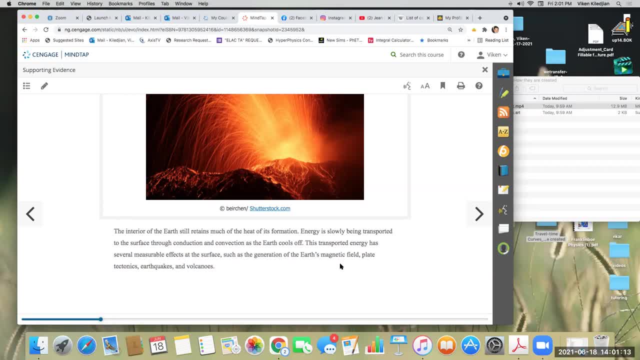 This transported energy has several measurable effects at the surface, such as the generation of the Earth's magnetic field, plate tectonics, earthquakes and volcanoes. In other words, it's saying all of these phenomena, the heat that we have, plate tectonics, earthquakes, volcanoes and magnetic field. 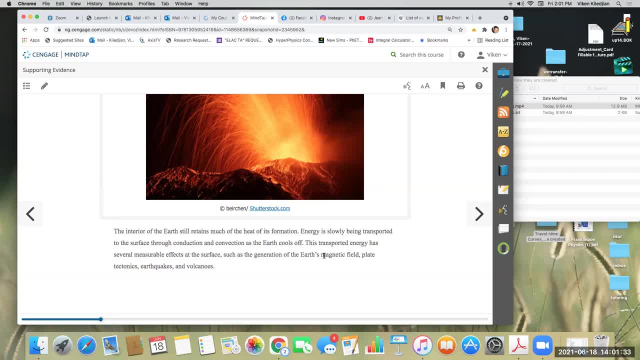 is a leftover of the original energy that the Earth had when it collapsed and formed into a planet, So that heat that originally the Earth was very hot, hotter than it is now- that heat that it still has- is causing all of these phenomena. Convection in the outer core is responsible for the Earth's magnetic field. 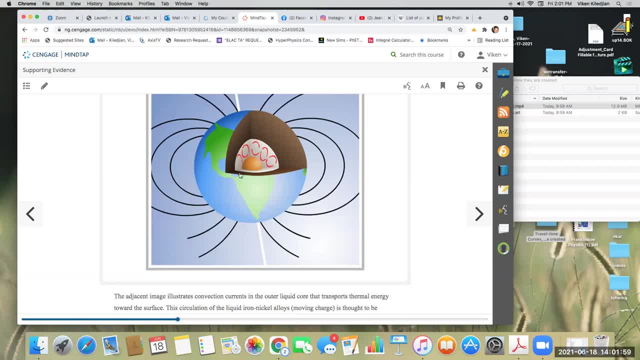 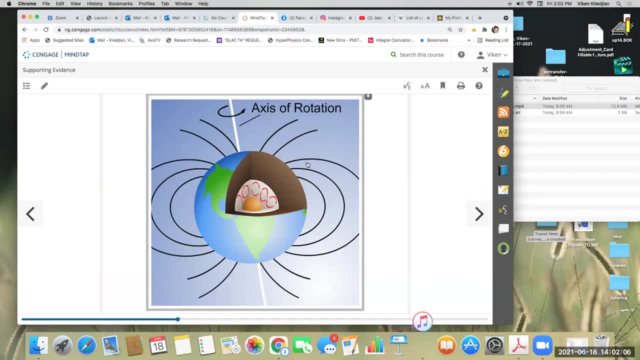 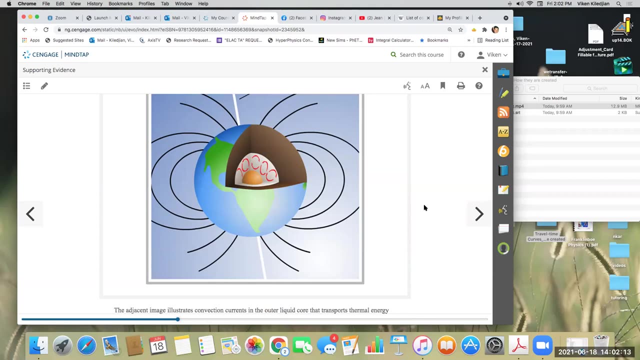 You see, so, as these convection currents are happening in the outer core of the Earth, in the liquid outer core that we were just talking about, they cause the magnetic field of the Earth And that really helps us because it helps protect us from the dangerous solar winds. 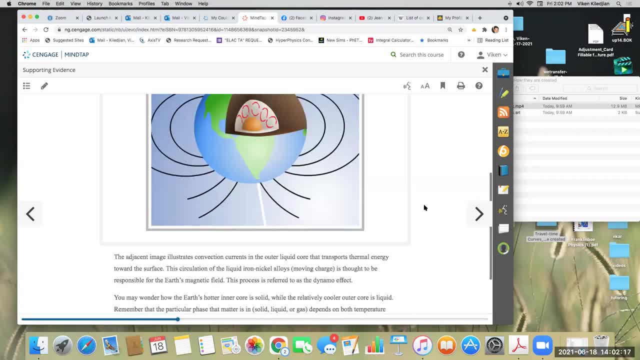 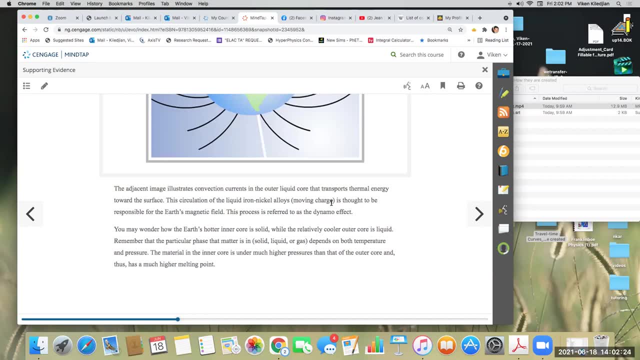 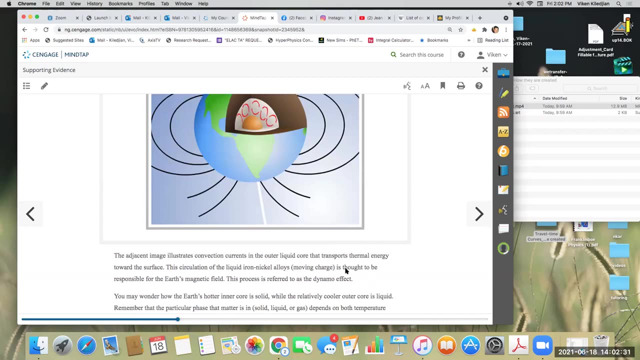 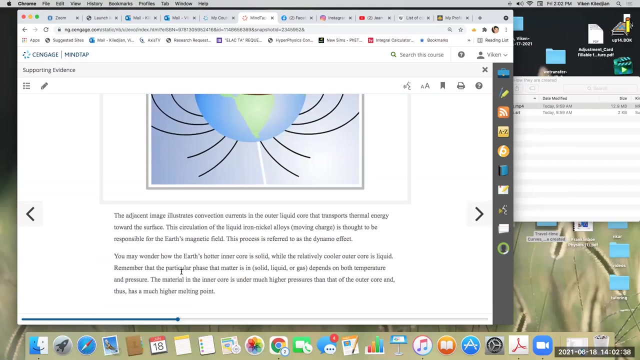 solar particles that are coming toward us. So the adjacent image illustrates convection currents in the outer liquid core that transports thermal energy towards the surface. This circulation of liquid iron-nickel alloys is thought to be responsible for the Earth's magnetic field. This process is referred to as the dynamo effect. 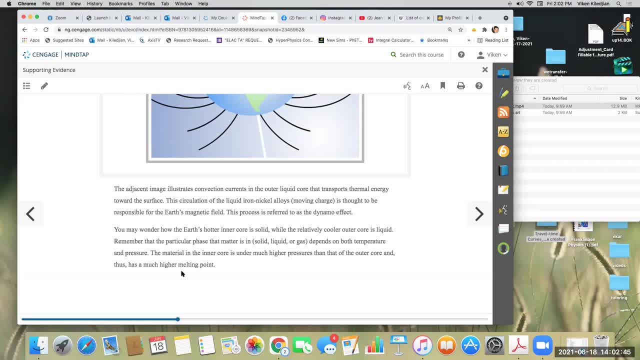 You may wonder how the Earth's hot inner core is solid while the relatively cooler outer core is liquid. Remember that the particular phase that matter is in depends both on its temperature and pressure. The material in the inner core is much higher pressure than that of the outer core. 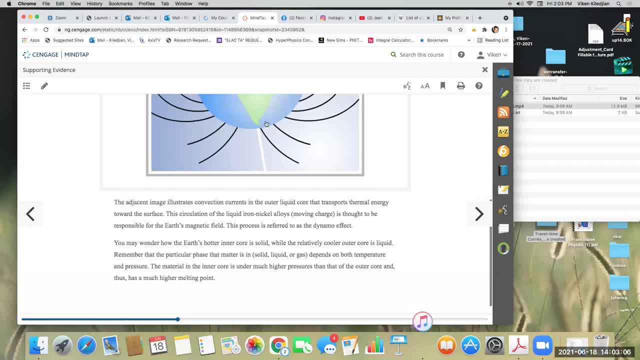 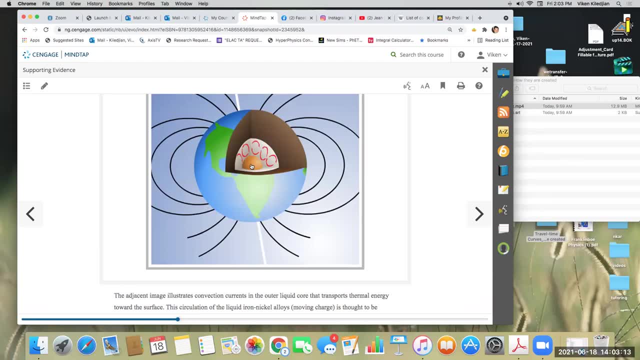 and thus has a much higher melting point. So the liquid core, which is the solid core, which is inside of the liquid core, you would think would be even more melted because it's hotter, But because of the higher pressure it changes back to solid because its melting point rises. 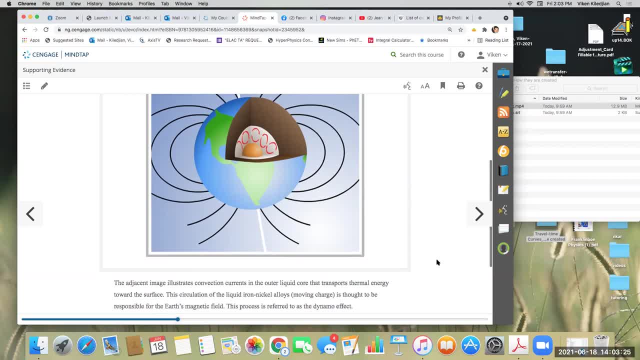 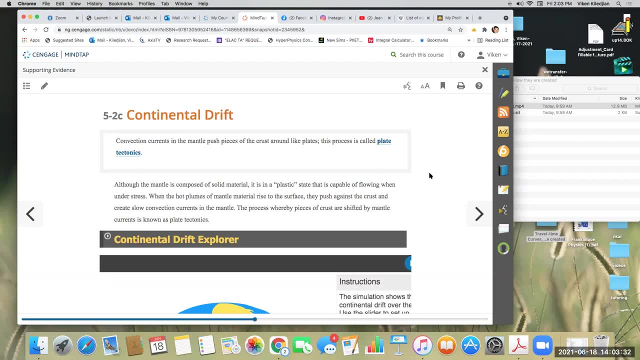 You see. So that's what turns it back to a solid Continental drift, also known as plate tectonics. Convection currents in the mantle push pieces of the crust around like plates. This process is called plate tectonics. 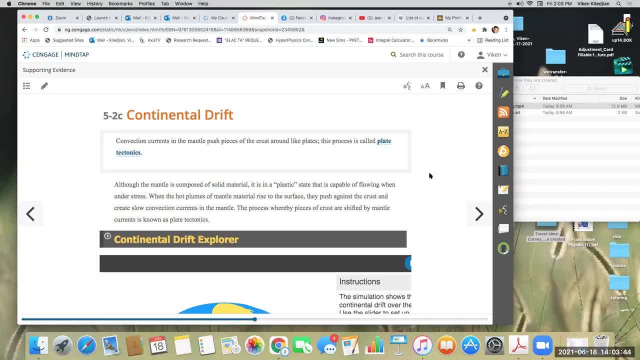 Although the mantle is composed of solid material, it is in a plastic state that is capable of flowing when under stress. Um, So, although it says the mantle is composed of solid, but it is in a plastic state that is capable of flowing, So we say that it is solid, but it is a flowing type of solid. 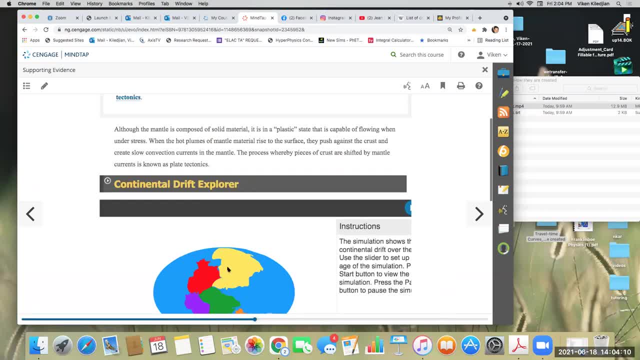 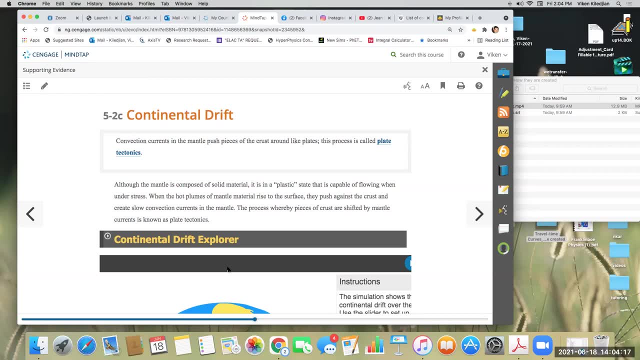 That's the mantle, And that's what we see when the mantle spews out of volcanoes. We're seeing this lava flow right. Even though it's flowing, we still call it a solid, The lava that's coming out of the volcano. 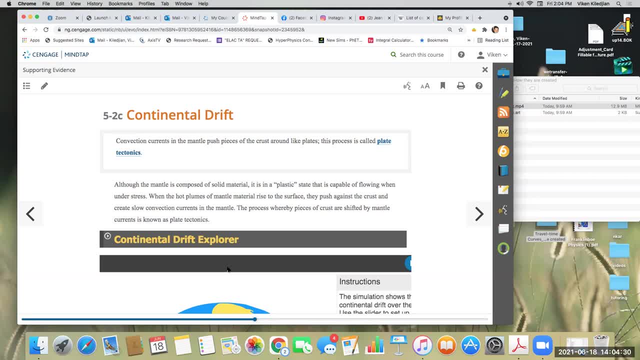 And as soon as it gets cold it just solidifies And we see the true solid nature of the lava. When the hot plumes of mantle material rise to the surface, they push against the crust and create slow convection currents. The process whereby pieces of crust are shifted by mantle currents is known as plate tectonics. 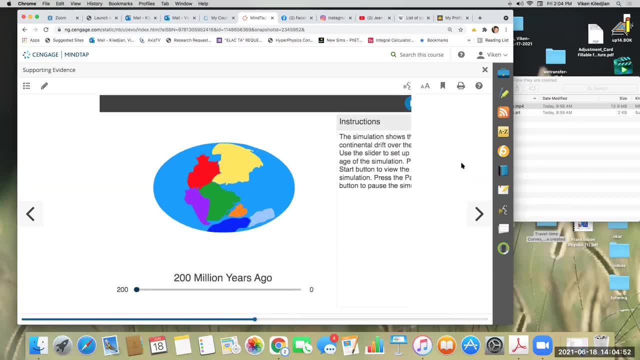 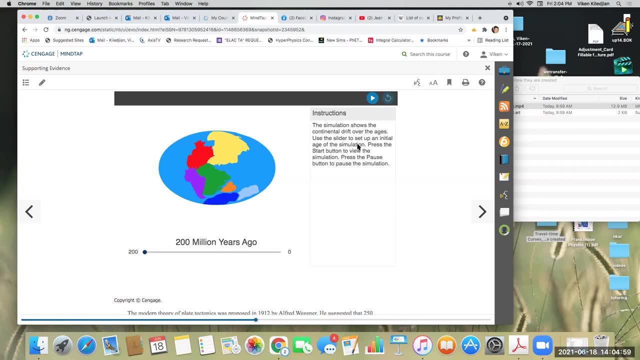 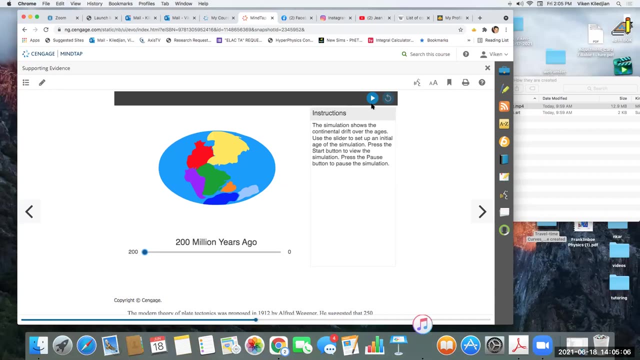 So this simulation- Let's go a little bit- Shows the continental drift over the ages. Use the slider to set up an initial age of the simulation. Press the start button to view the simulation. So you can kind of see here, Oops. 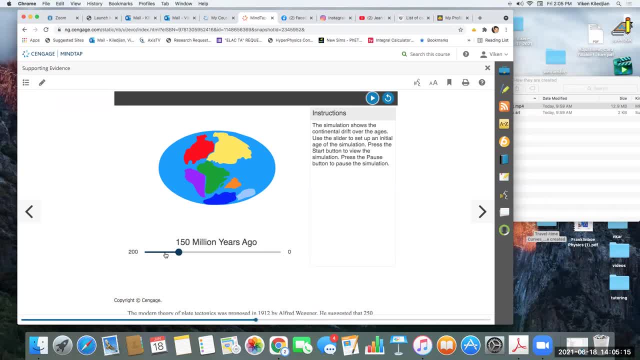 You can stop it at any point. So you see, originally you have Everything is kind of like almost together. That's called Pangea, When all the continents were together. Then the continents broke apart. So you can see now Africa and South America were together with North America and Asia. 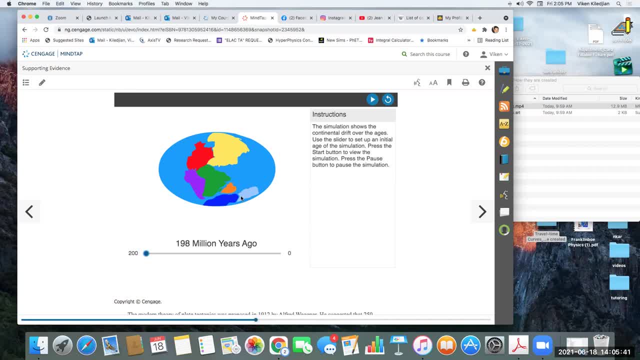 And then this is what became modern day India And Antarctica and Australia. So then, when I drag it, This is 20 million years ago. Then when I go like this: Already South America has split from North America And the splitting of through Africa is starting to occur. 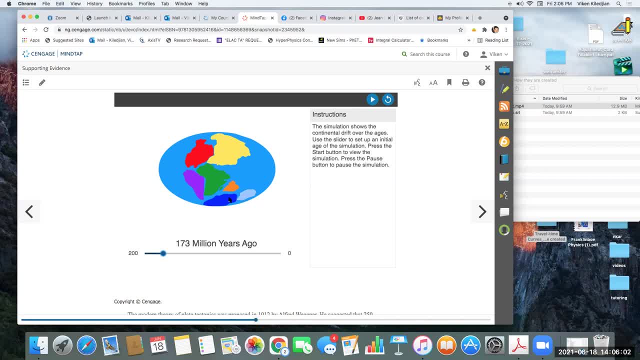 And the Australia is beginning to split from Antarctica. So now, Okay, Now you see this one, The split has really happened here. South America and Africa- This is still kind of together, But India is way apart from Africa. Ooh, 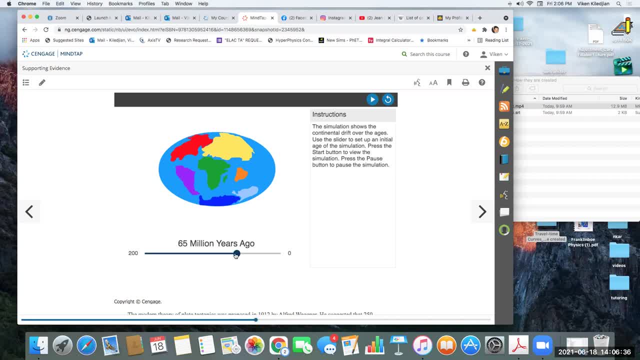 I like that. All of a sudden, the shift of direction. See this one, This one was going that way, Then it all of a sudden turned this way. Then Alaska is separating, Separated- Oh, now notice what's happening here. This one, 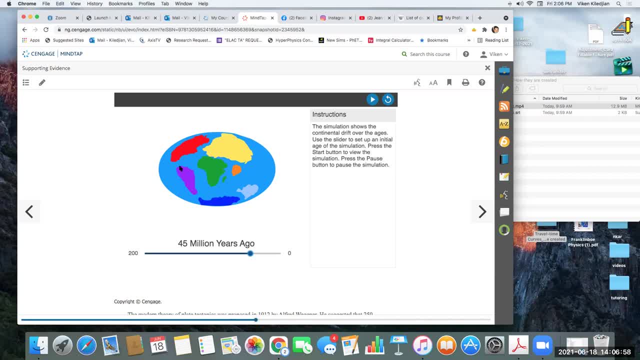 Central America is beginning to form, See right here. So right now this is like North and Central Right Together And this is South America. So now Central America is starting to form And India is starting to get pushed towards the Asia. 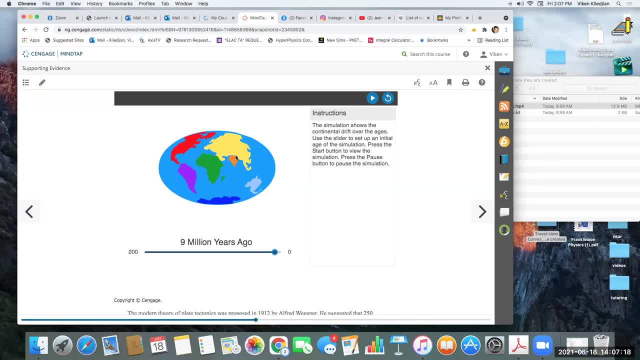 That's where you get these big mountain ranges: The San Andreas, Not San Andreas, Mount Everest, Right Right here, Mount Everest. This guy is pushing up against that And pushing it upwards And forming mountain ranges, And then Central America is going to eventually close with South America. 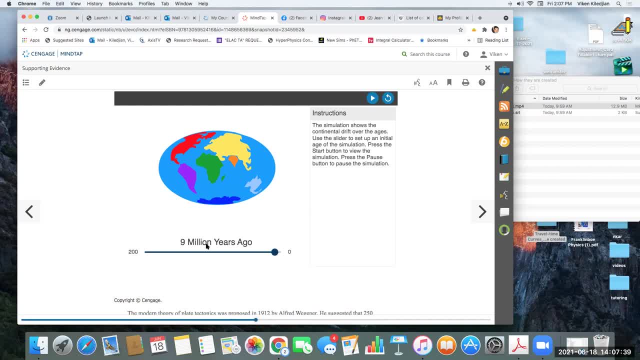 This is 9 million years ago And finally 3 million years ago And then present. So you see, now you've got the whole North America, Central America, South America, Africa. So So interesting how that happened, You know. 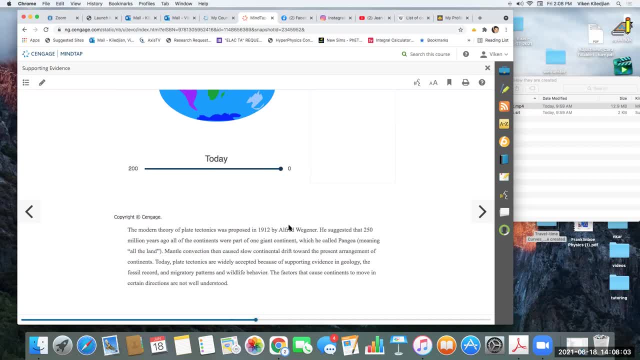 So this was proposed by 1912 by Alfred Wegener. He suggested that 250 million years ago all of the continents were part of one giant continent, which he called Pangea, Meaning all the land. Mantle convection then caused slow continental drift. 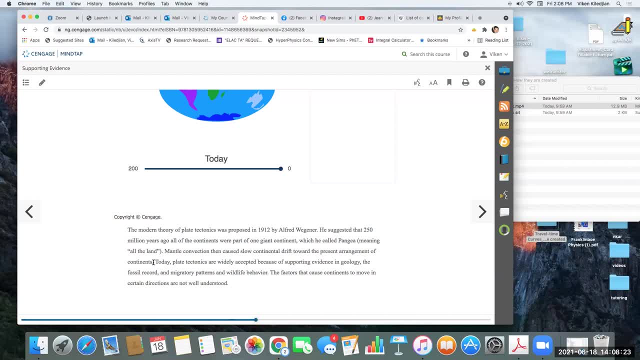 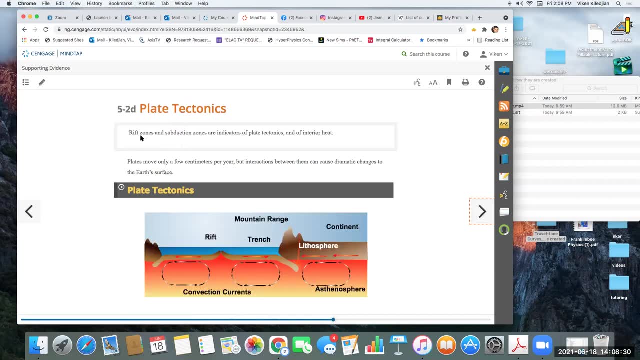 That present arrangement of Until, the present arrangement of continents, Plate tectonics, Rift zones and subduction zones are indicators of plate tectonics And of interior heat. So you see, here This is a rift, Meaning two plates are getting separated. 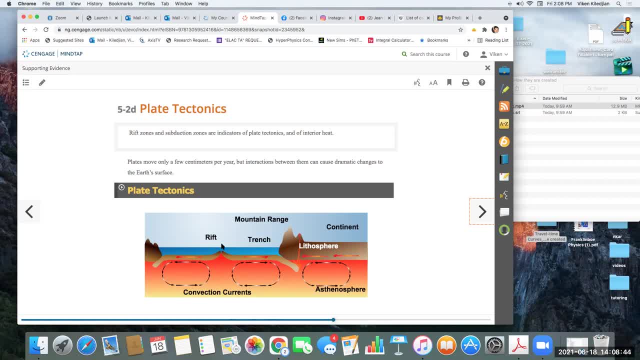 So when the convection under the earth pushes this up, These two plates start moving this way And the rift is created here, And then this plate comes And then subducts under this one, Under the, So this plate comes And goes under. 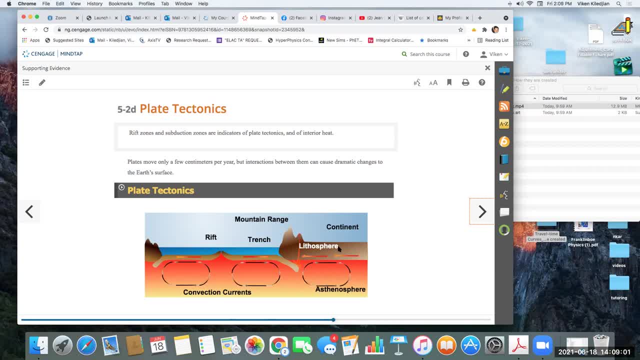 Subducts under the other of the continental plate And then hot material rises into volcanoes. You see, Right here As this, As this material, As this plate is going under, This hot material here is going upwelling And then you expect there to be volcanoes where one plate is going underneath the other one. 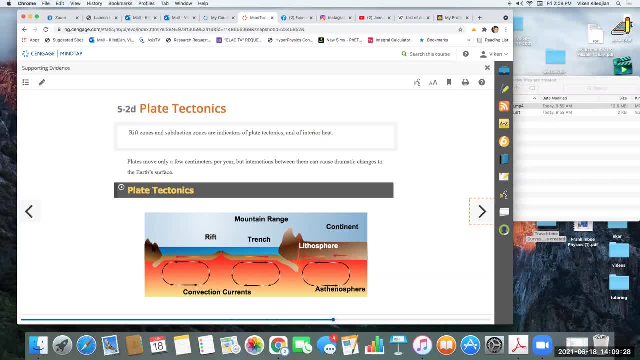 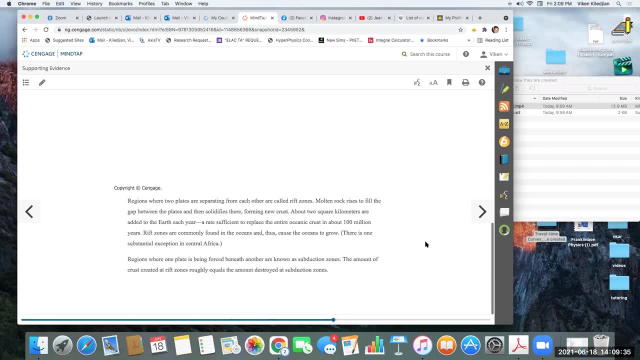 And then same thing here on the other side. You see. So rift regions, where two plates are separating, are called rift zones. Molten rock rises to fill the gap And then solidifies, But two square kilometers are added to the earth each year. A rare A rate sufficient to replace the entire oceanic crust in about a hundred million years. That means our earth keeps replenishing its crust Every hundred million years, Right, So that's very interesting. So therefore, you don't expect to find too many old rocks older than a hundred million years. If you were to go search under the ocean rocks Because it's renewing itself. It's kind of almost like our skin, which renews itself every day. We shed it And then it renews itself eventually over time. So rift zones are commonly found in the oceans. 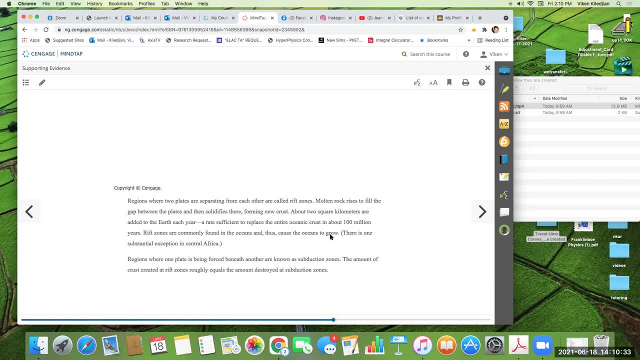 And thus cause the oceans to grow. There is one substantial exception in Central Africa. Regions where one plate is being forced beneath another are known as subduction zones. The amount of crust created at rift zones roughly equals the amount of destroyed at subduction zones. 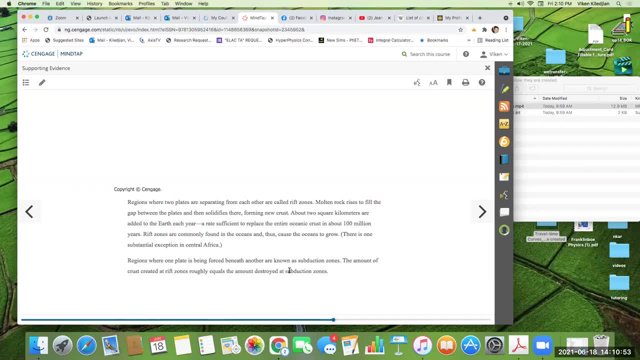 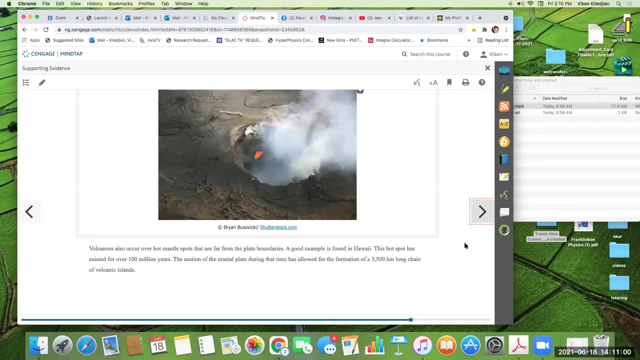 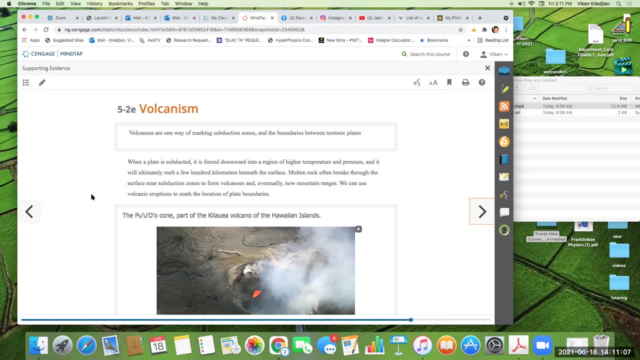 So you're creating at rift zones And then you're destroying them underneath when you're getting to the subduction zone. Volcanoes are one way of marking subduction zone and the boundaries between tectonic plates. The Pu'u O'Kon, part of the Kilauea volcano of the Hawaiian Islands. 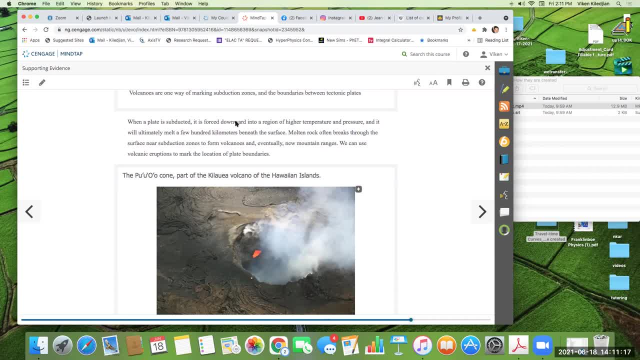 When a plate is subducted, it is forced downward into a region of higher temperature and pressure, And it will ultimately melt a few hundred kilometers beneath the surface. You see that. You see what's happening. So the plate is being subducted, melting. 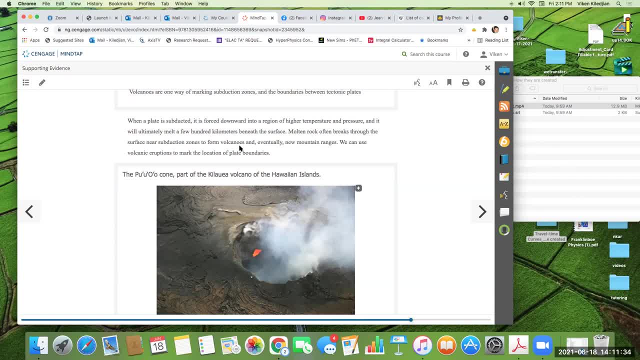 And then it says: the molten rock often breaks through the surface near subduction zones to form volcanoes and eventually new mountain ranges. You see, So when that plate melts, it starts to rise. It starts to rise due to the convection currents. 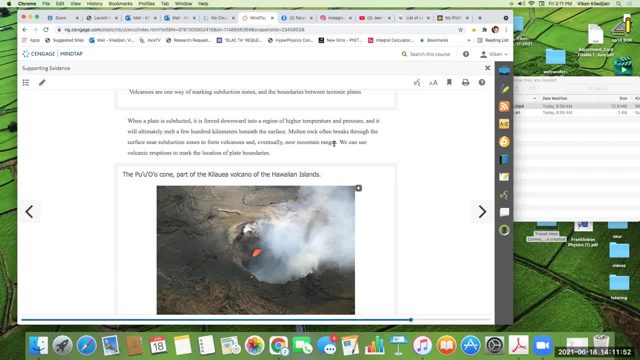 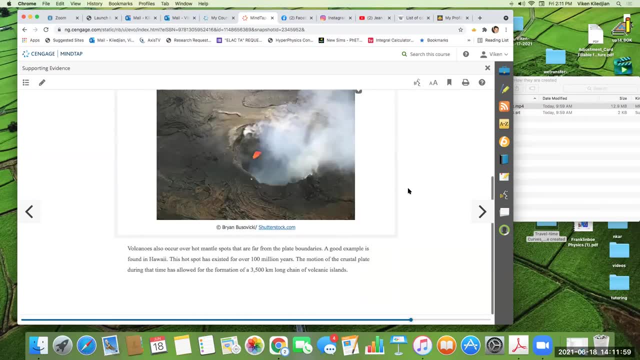 And it gets pushed up And then you create mountains and volcanoes. So volcanoes also occur over hot mental spots that are far from the plate boundaries. A good example is found in Hawaii. This hot spot has existed for over 100 million years. 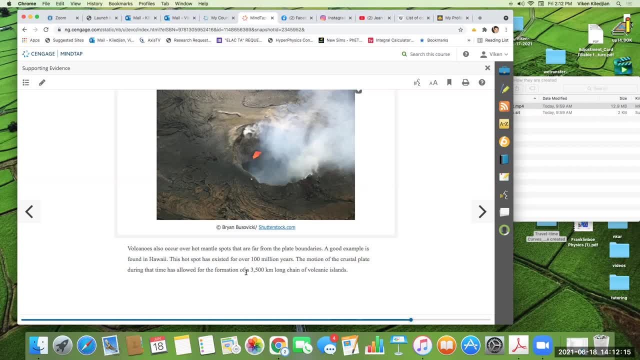 The motion of the crustal plate during that time has allowed for the formation of 3,500 kilometers long chain of volcanic islands. So, basically, as the crust is moving, there's a hot spot beneath it which is welling up And creating the Hawaiian chain of islands. 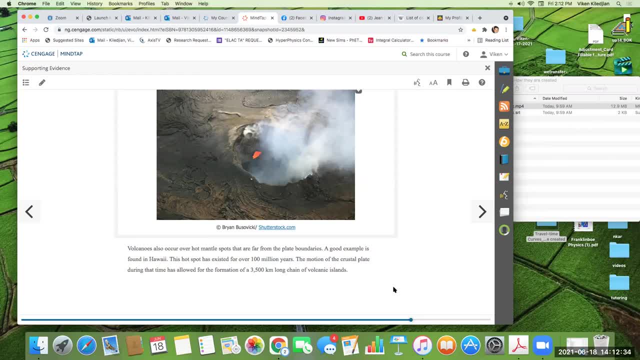 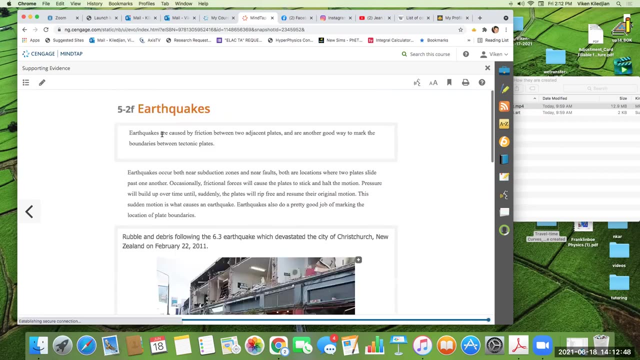 That's how we get Hawaii. So there is no subduction zone taking place in Hawaii. It's just that there's a hot spot underneath it And the plate is passing by it. Earthquakes are caused by friction between two adjacent plates and are a good way to mark the boundaries between tectonic plates. 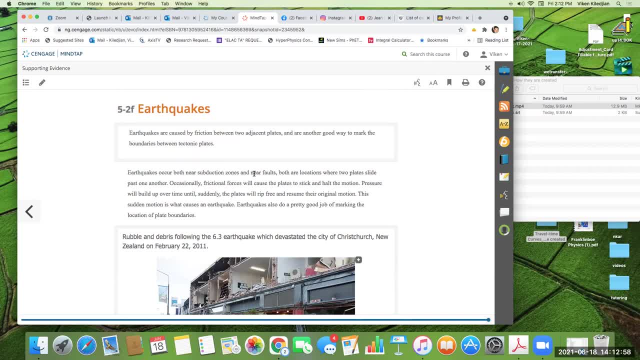 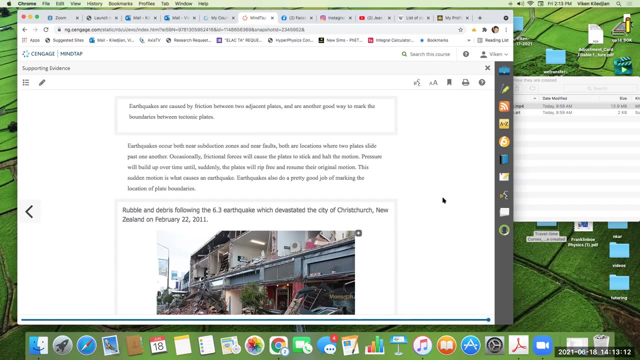 Earthquakes can occur both near subduction zones, near faults. Both are locations where two plates slide past one another. Occasionally, frictional forces will cause the plates to stick and halt. the motion. Pressure will build up over time until suddenly the plates will rip free and resume their original motion. 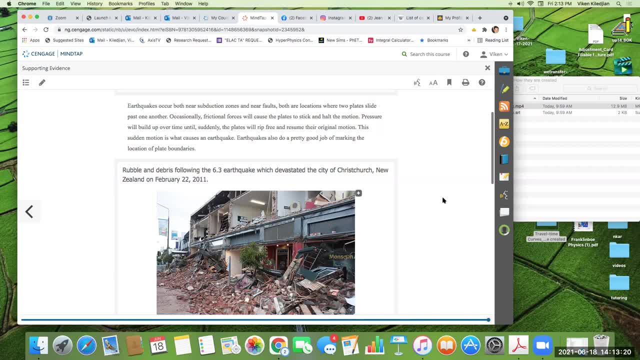 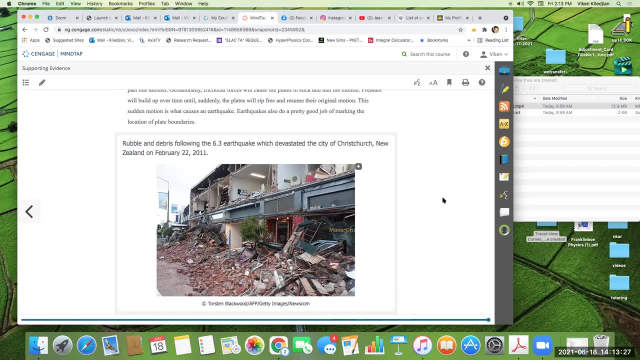 This sudden motion is what causes an earthquake, So it says here. Rubble and debris followed the 6.3 earthquake which devastated the city of Christchurch, New Zealand, on February 22, 2011.. Pretty scary man when you look at the pictures. 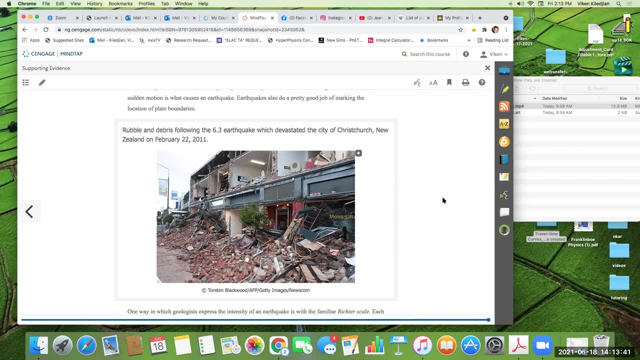 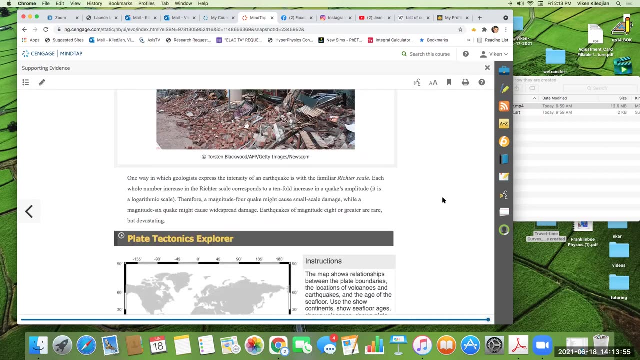 And that's only a 6.3. And you expect a bigger one to hit LA. So one way in which we can do this, So one way in which geologists express the intensity of an earthquake, is with the familiar Richter scale. 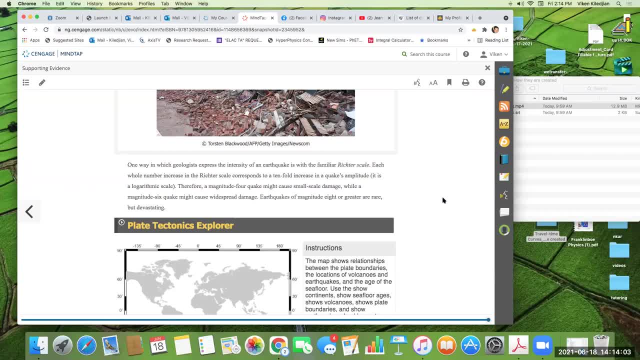 Each whole number increased in Richter scale corresponds to a tenfold increase in the quake's amplitude. It is a logarithmic scale. Therefore a magnitude 4 quake might cause small-scale damage, while a magnitude 6 quake might cause widespread damage. 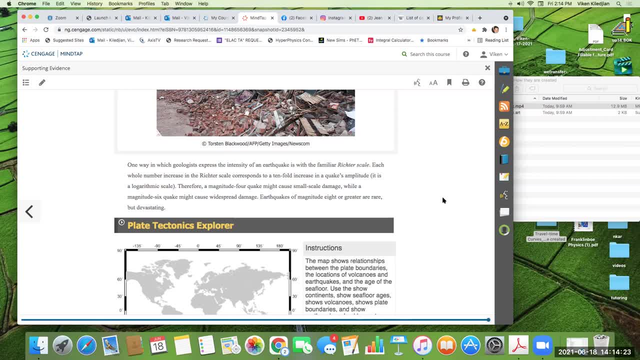 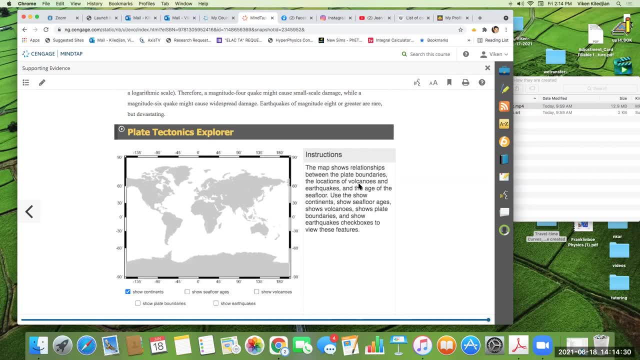 Earthquakes of magnitude 8 or greater are rare but devastating. The map below shows relationships between plate boundaries and locations of volcanoes and earthquakes and the age of the seafloor. Use the show continents, show seafloor ages, show volcanoes and show plate boundaries. 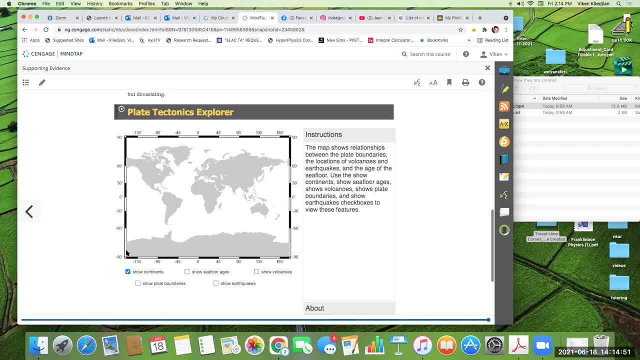 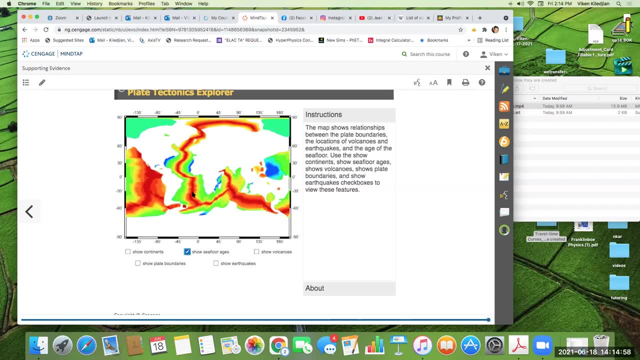 And show earthquake checkbox to view these features. So if I uncheck this it doesn't show boundaries, But I could show the seafloor ages. You see, this is the newer age. This is the big rift zone in the Pacific Ocean. 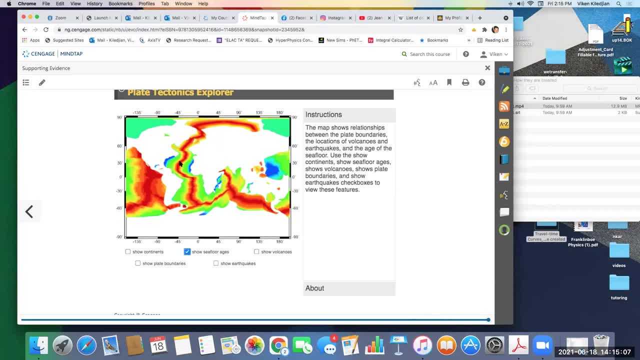 So see, red means newer plates, newer boundaries, And then this is the. these are newer boundaries too. Well, this is, Like I said, the Meridian, and the Blue is the rift zone in the Pacific Ocean. So this is the seafloor ages, and the seafloor ages are 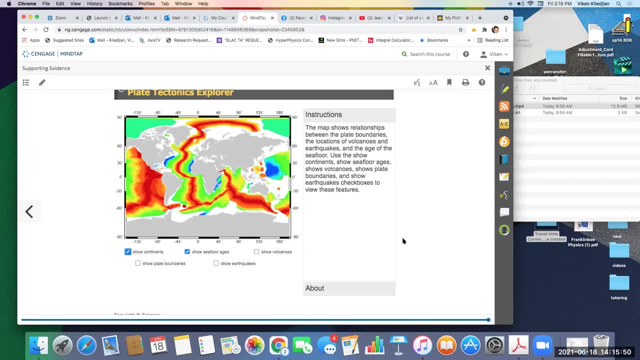 You can see the crux of the of the. You can see the crux right there. That's it oldest. so now show volcanoes. so if i undo the, okay, so then you can see here. you see where the volcanoes are. that tells you something about what's happening there. you see, right there. 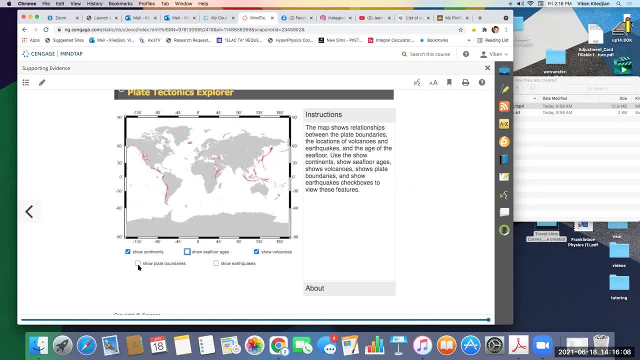 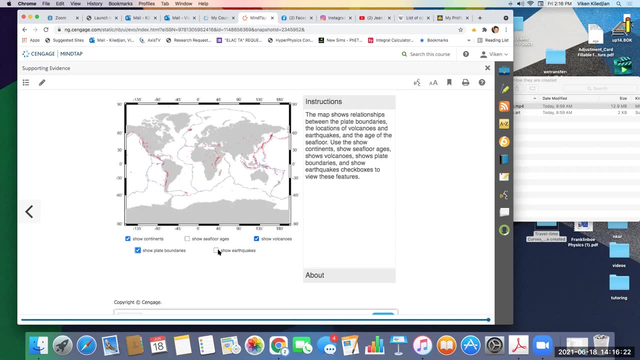 right there, that's where the volcanoes are. show plate boundaries. ah, you see, there you can see what is happening here. um, right there, a bunch of volcanoes here, so show earthquakes. oh wow, so bunch of earthquakes here along the western coast, so we would expect earthquakes where plate boundaries are, so start. 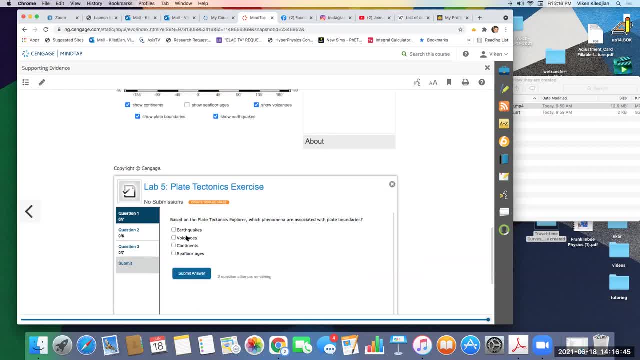 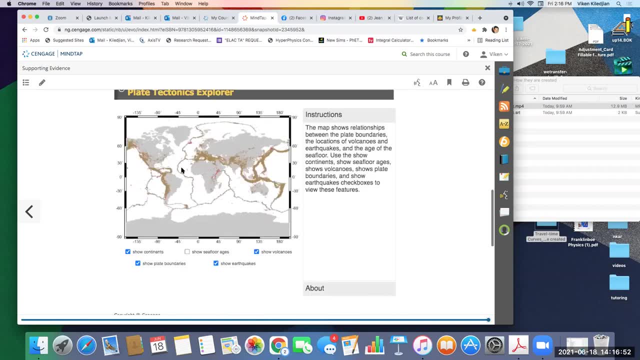 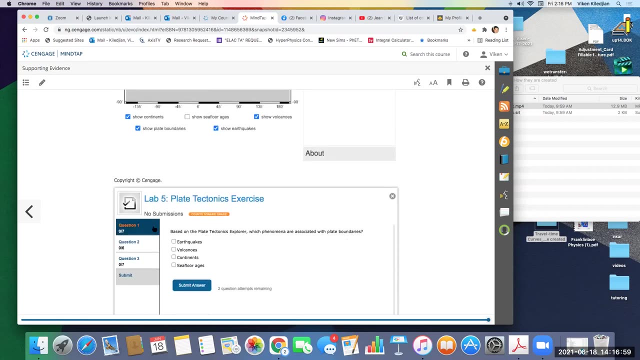 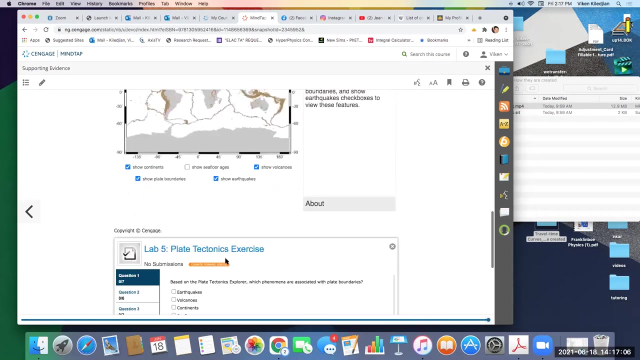 with this one. so, again, this one, based on the plate tectonics explorer, which is this one: uh, which phenomena are associated with plate boundaries? so, uh, you can, then, uh, you can, tend to take a picture here to support your answer, which on the which phenomena are associated with plate boundaries. so what you would do? 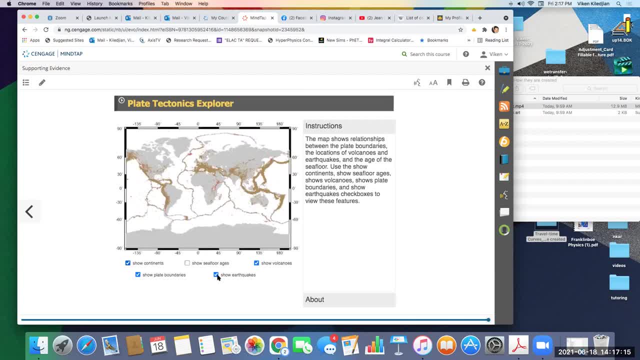 is: keep the continents and then one at a time. you would go like this: right, maybe even get rid of the continents and then just go: okay, show plate boundaries and then show sea floor agents. so try to see: is there a correlation between sea floor ages and where the boundary of the plate is like this? so take a. 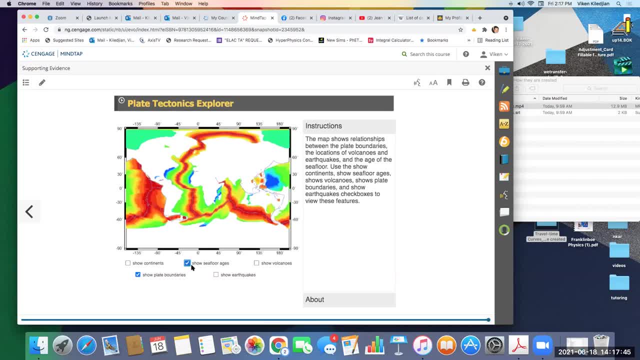 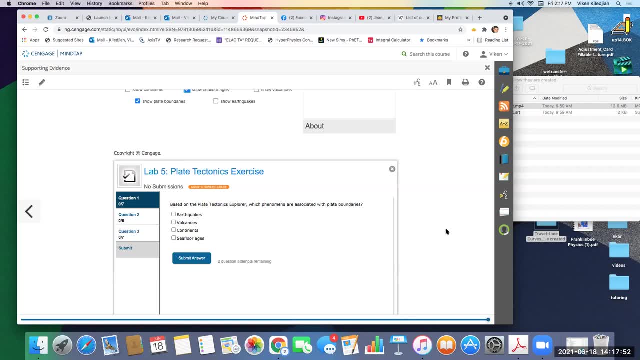 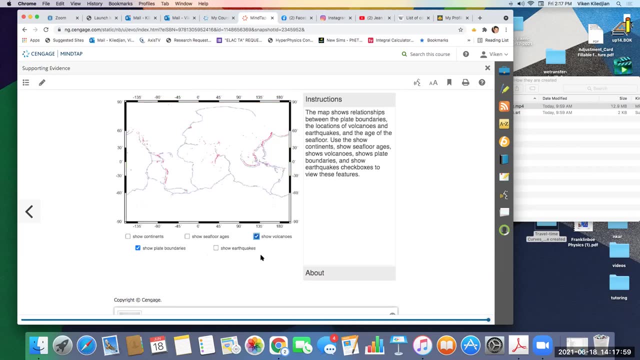 picture of this. then just with these two, check so see if there's a relationship. and then, if there's a relationship, then put sea floor ages right, then take a, uncheck this and then show volcanoes right. so you don't- you probably don't- need the continents, it kind of gets in the way. so you're. 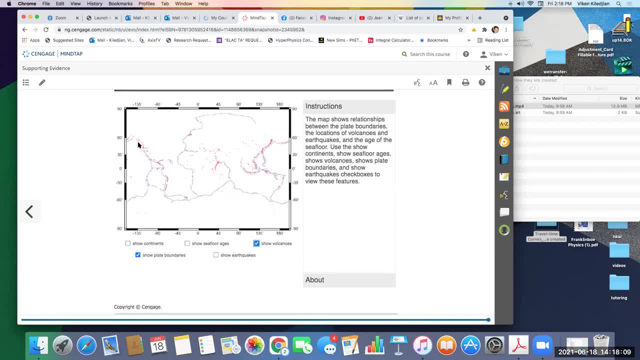 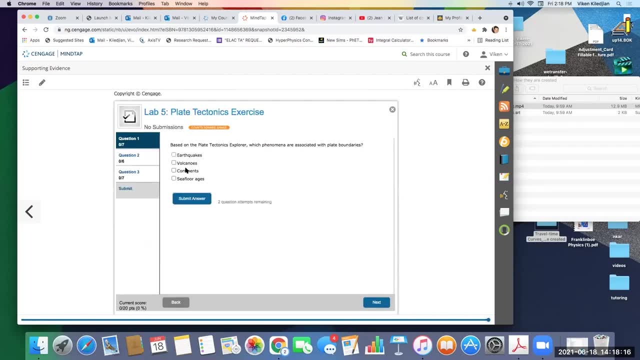 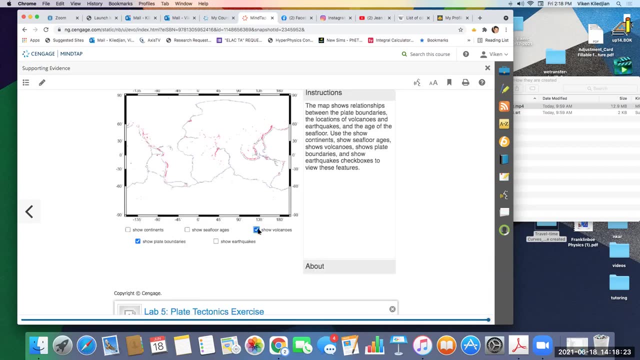 just comparing where the volcanoes are to the plate boundaries. is there a relationship? so now take a picture of that and then, if it, if there's a relationship, then you put volcanoes and then which phenomena are associated with plate boundaries. okay, then you do continents. are continents associated with plate boundaries? so take a picture. 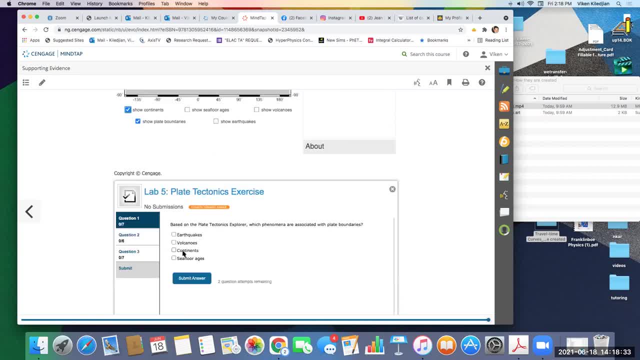 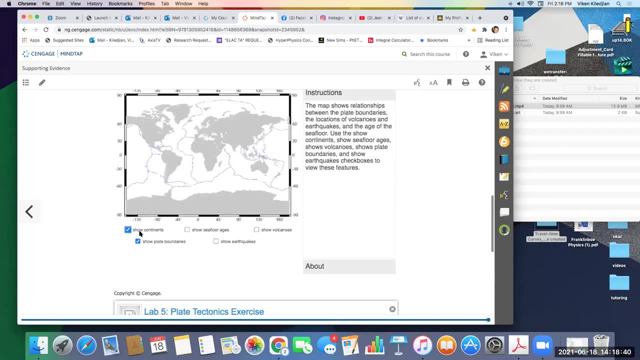 like that and then answer if the that's related. so then you put a check and then the same thing: what's the other one earthquakes. so this is always checked for each picture, but we're only changing one thing at a time. that's why we're taking four pictures, because you don't want to have like this and confuse. 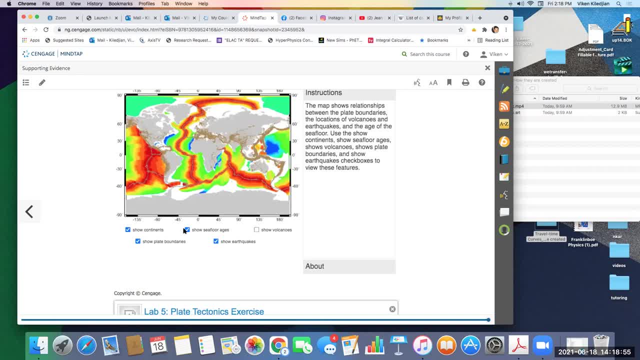 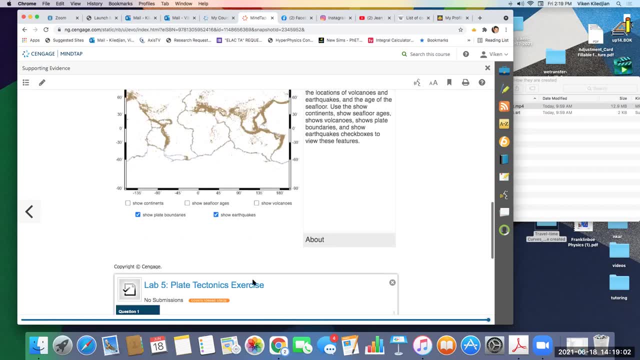 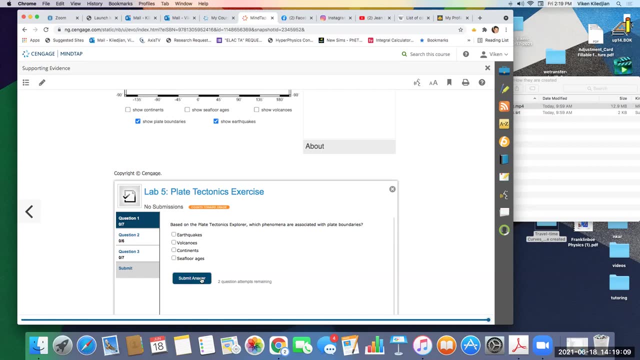 everything you see. you want to have only one thing checked at a time. so now to see: is there a relationship? then you go over here, so that's probably. you're taking one, two, three, four pictures and then you're checking whichever one. they're related, you're scaling submit and 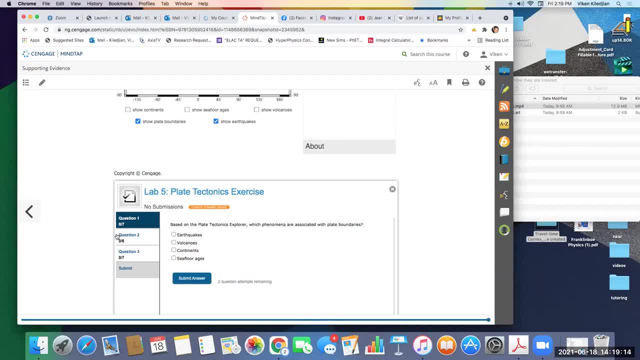 then taking a picture of your answer, whether you are correct or not. okay, i've seen on the plate tectonics explorer. two plates meet on the western border of south america. which plate is being subducted? the plate on the east side of the boundary or the plate on? 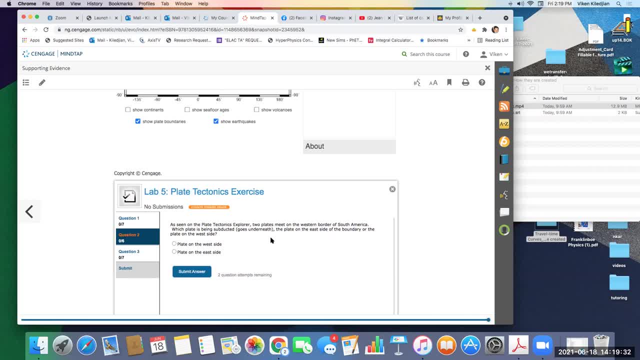 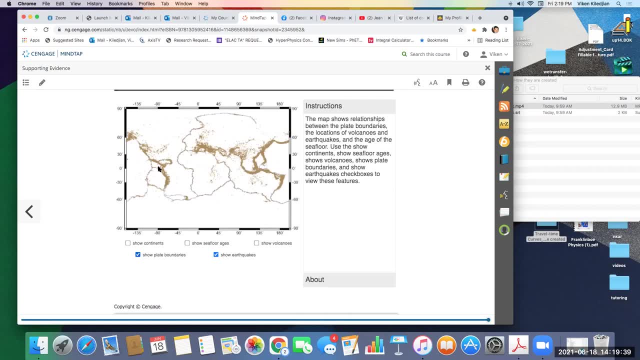 the west side. um, that one you could. actually, you don't need to take another picture because you've already got four pictures: one with plate boundary and earthquake showing. then you have another one with plate boundary and volcanoes showing. so now you're focusing in on the, on the. i think the 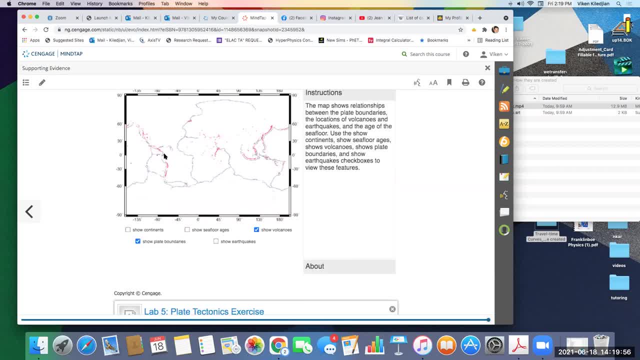 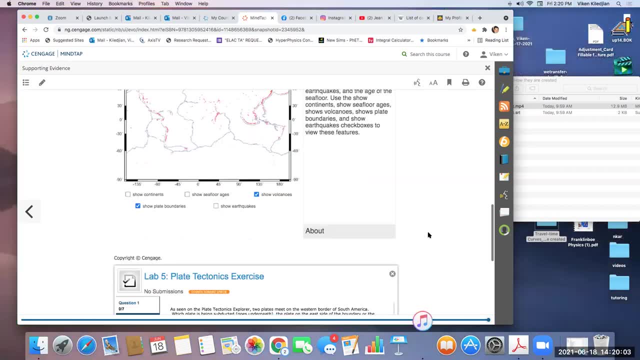 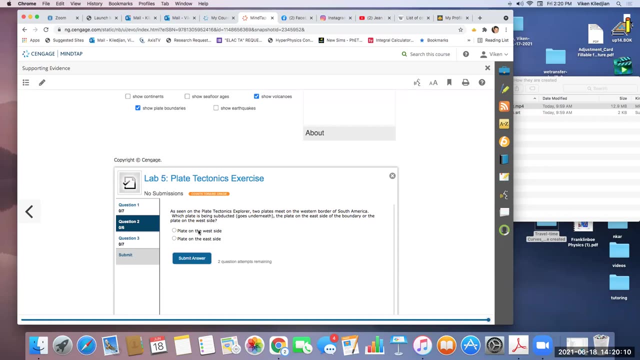 western border of south america, which is right, right here, then decide: is this plate going underneath that plate or that plate going underneath this plate? uh, right, and then. so, based off of that picture, essentially you're basing it. so you uh then make a decision which plate it is, with a plate on the west side or the east side. okay, then question three: japan. 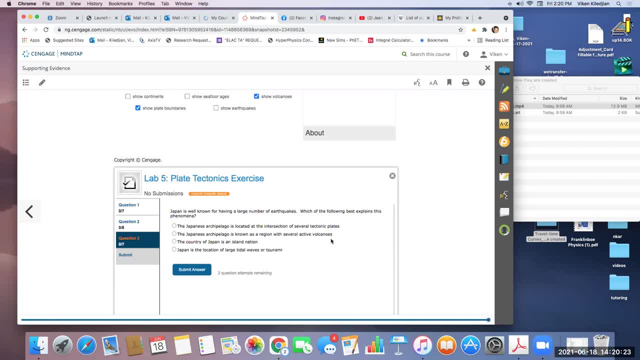 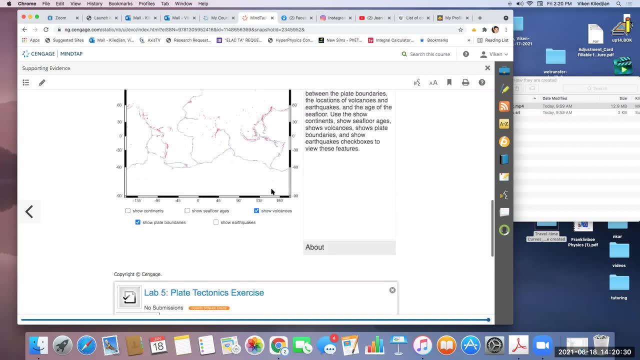 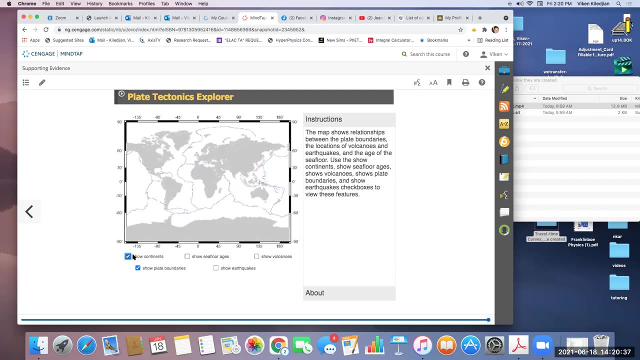 is well known for having a large number of earthquakes. which other family best explains this phenomenon? so again, i believe you can base that on the one, several of the pictures before. so you already have a picture of show plates and the continents. you might want to zoom in on those. 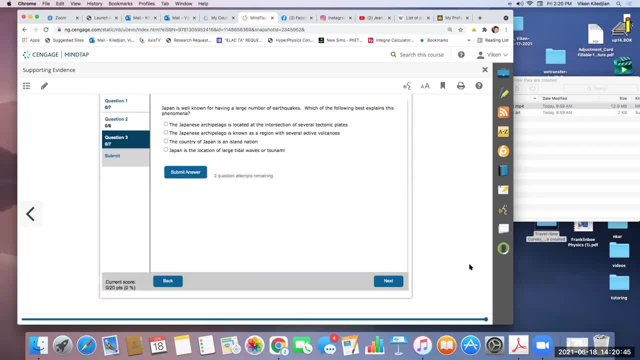 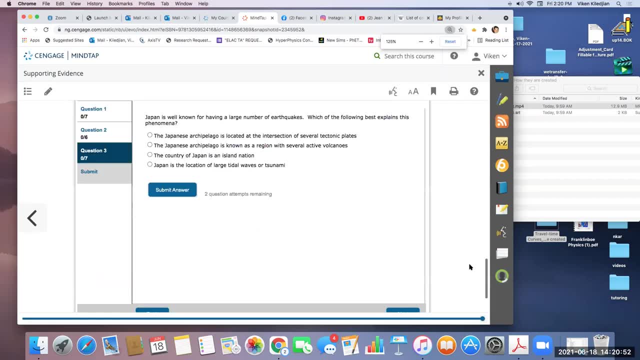 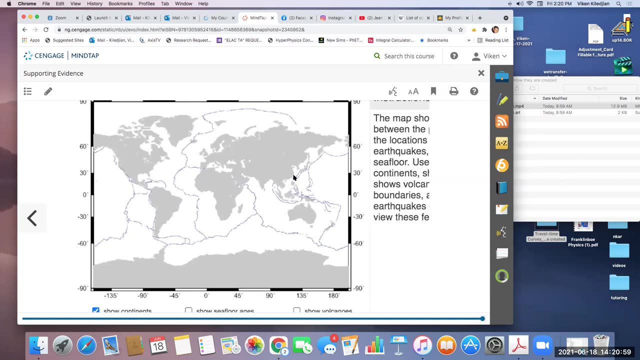 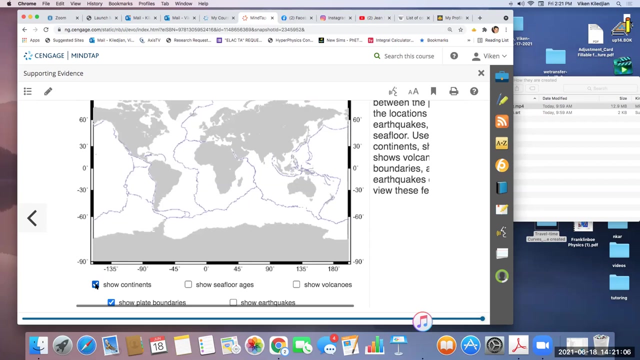 pictures because it's a little bit unclear. so when you're taking the pictures, taking the big zoom a little bit bigger, where's japan? i think it's this one, right like there. so now this shows this, just shows plate boundary and show continents. then the other one will show plate boundary and show earthquakes. 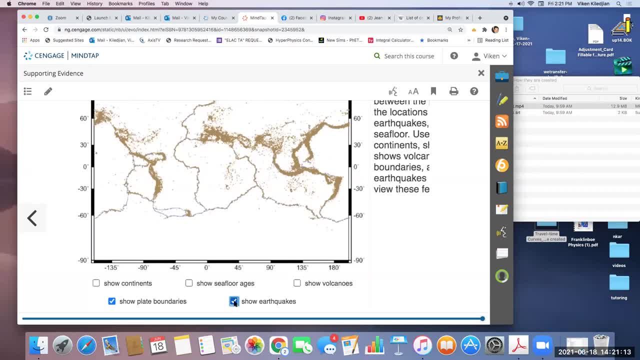 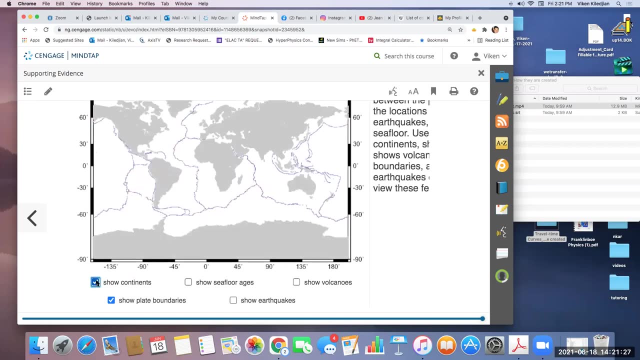 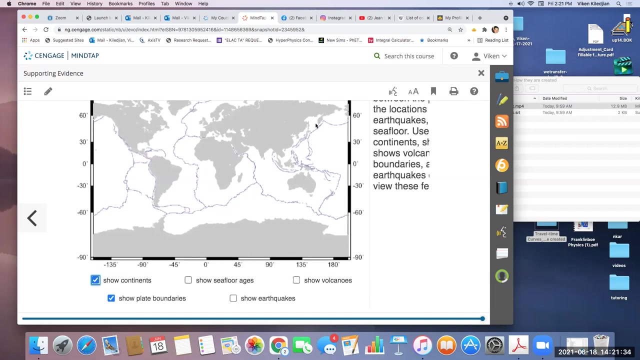 you see, then compare them and then, um, let's see if we show them together. yeah, i see that japan will actually be hidden behind this, you know? uh, so yeah, japan, is this one right here? i'm pretty sure i don't think it's that one. yeah, it's this one. 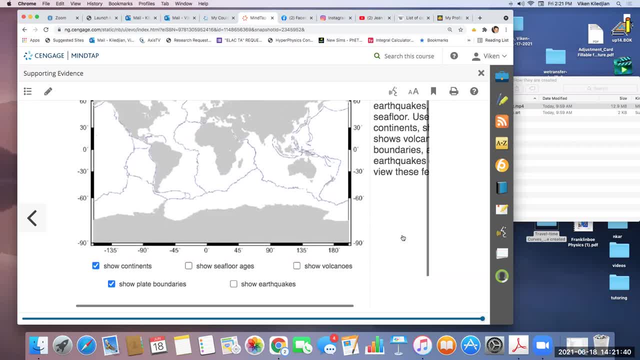 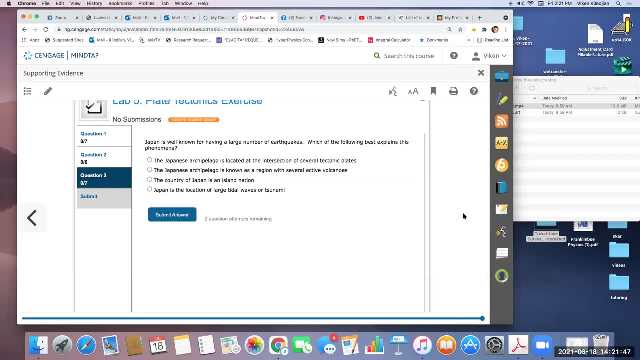 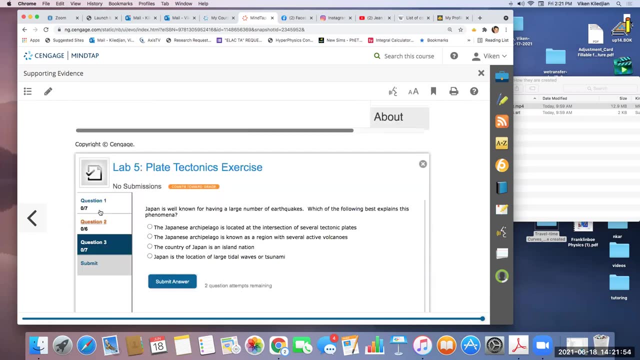 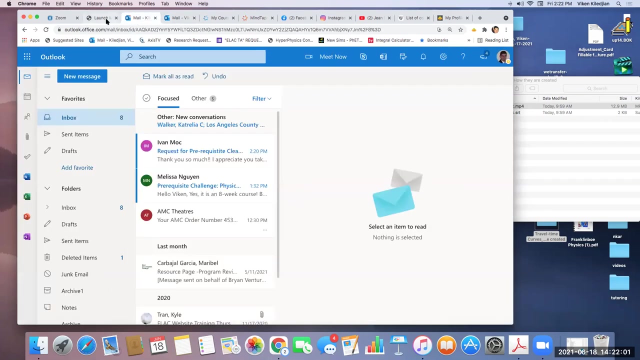 um, so then, uh, based on those pictures, you can decide which of the answers and then show the picture here. so basically, that's going to be four pictures just from the first question, and then from there you should be able to then three pictures for each question, and i think we're left with the last portion. uh, let's see where was i? 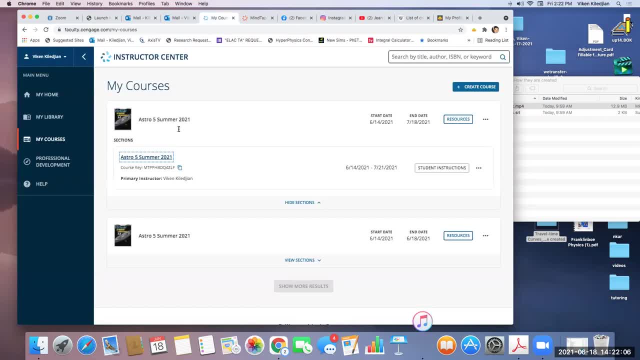 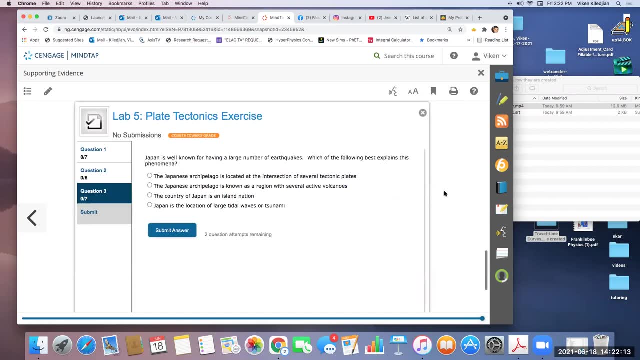 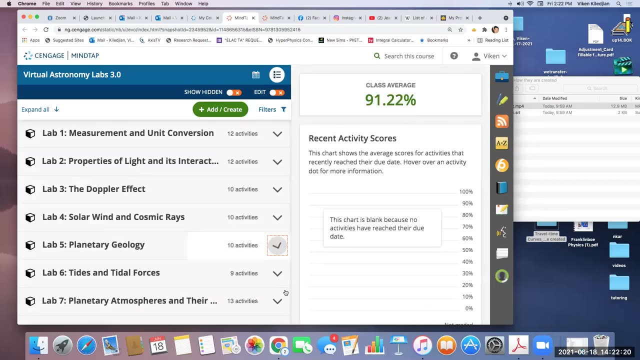 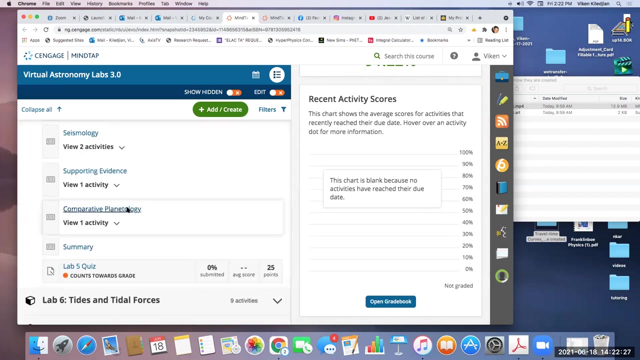 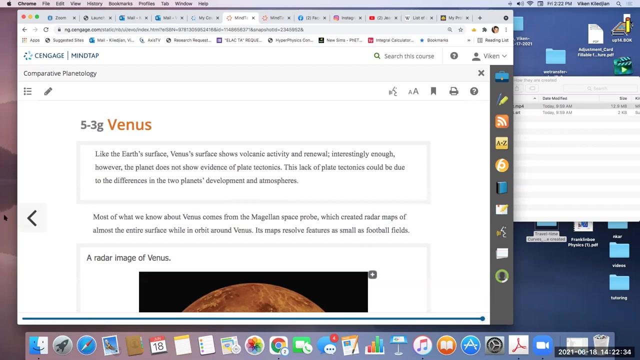 i think we are done with that part, aren't we? yeah, there's no arrow here, so then we're gonna go to back to the planet geology. the last activity here, comparative planetology. oh uh, the next one is uh, uh, uh, uh, uh, uh, uh. let me go to, uh, the first page. 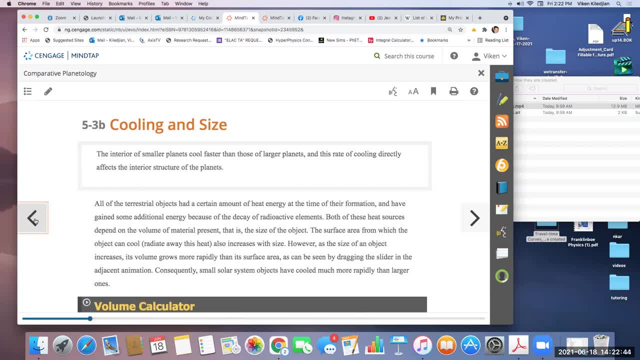 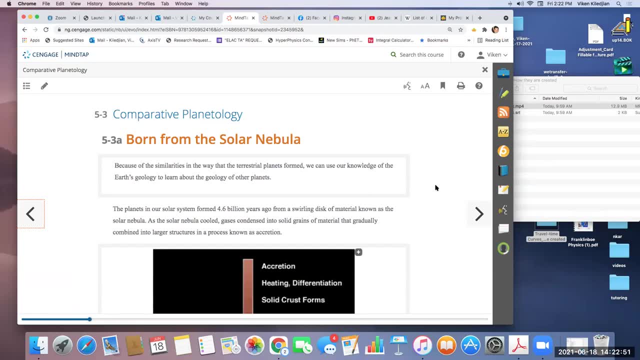 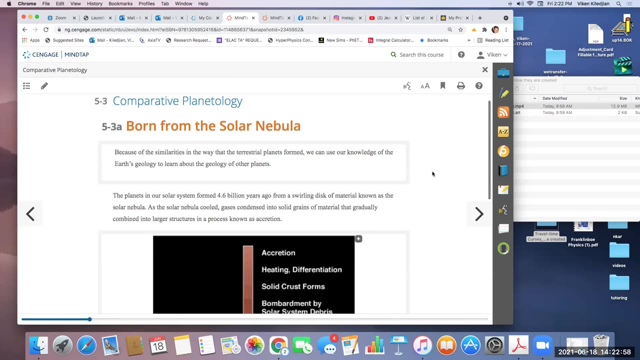 so they're going to compare the planets to each other. because of the similarities in the way that terrestrial planets formed, we can use our knowledge of the earth geology to learn about the geology of other planets. the planets in our solar system form 4.6 billion years of earth. to learn about the geology of other planets. 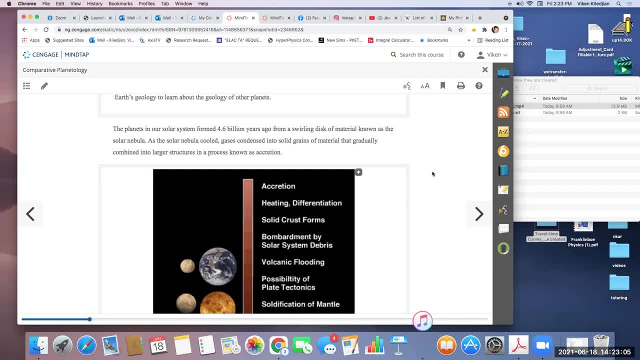 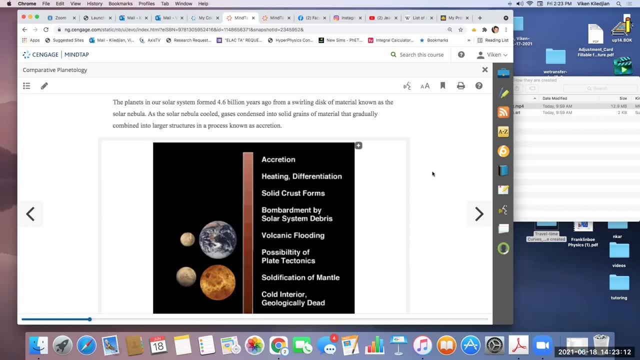 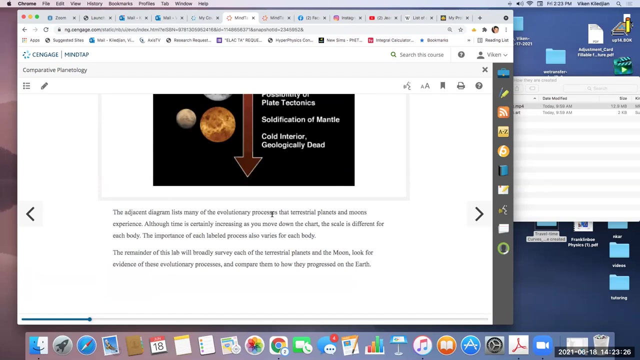 ago from a swirling disk of material known as the solar nebula. As the solar nebula cooled, gases condensed into solid grains of material that gradually combined into larger structures in a process known as accretion. So adjacent diagram: this: many of the evolutionary processes that terrestrial planets and 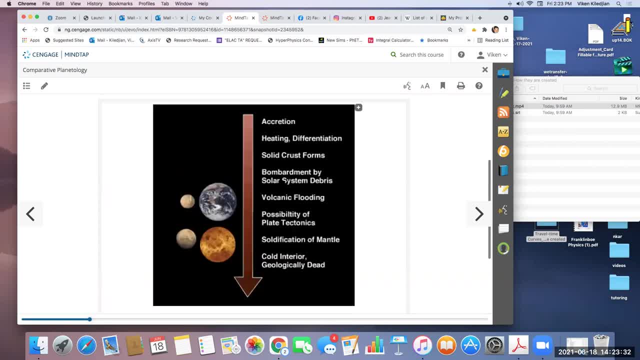 moons experience. So these ones here, Solid crust forms, heating and differentiation. Remember, differentiation means the denser material sinks. then crust forms bombardment by the solar debris, volcanic flooding, some possibility of plate tectonics, solidification of the mantle and then 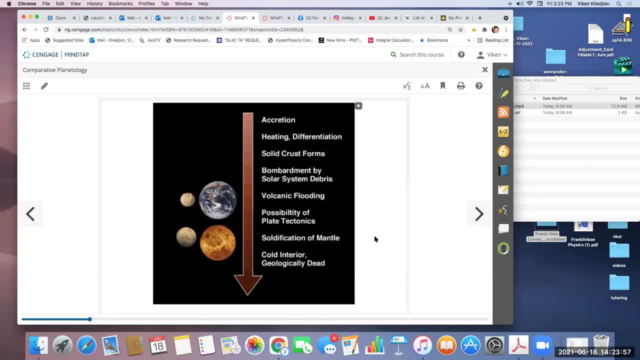 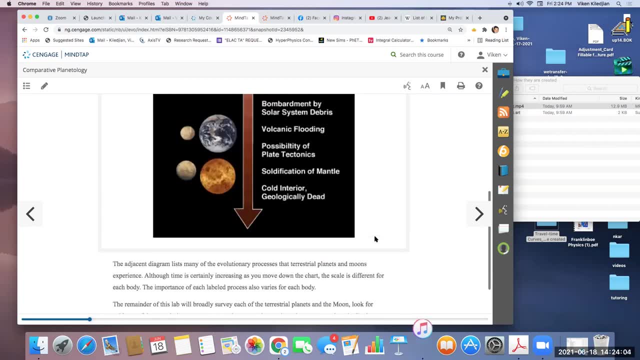 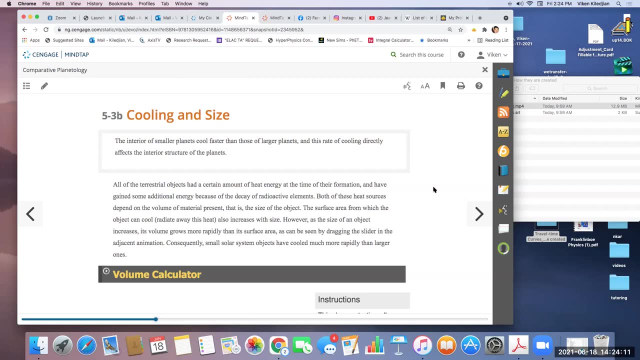 cold interior, geologically dead Cooling. The interior of a small planet cools faster than those of larger planets And this rate of cooling directly affects the interior structure of the planet. So smaller planets, it's saying, cool faster. The interior of a small, 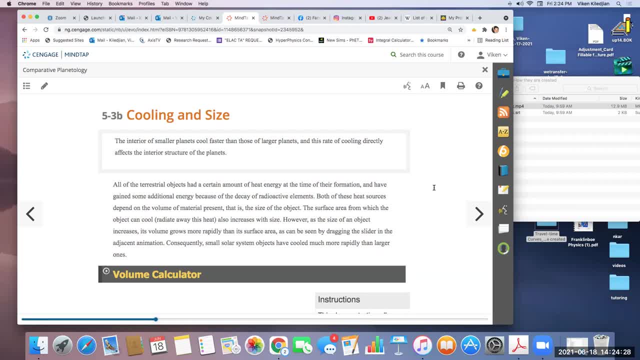 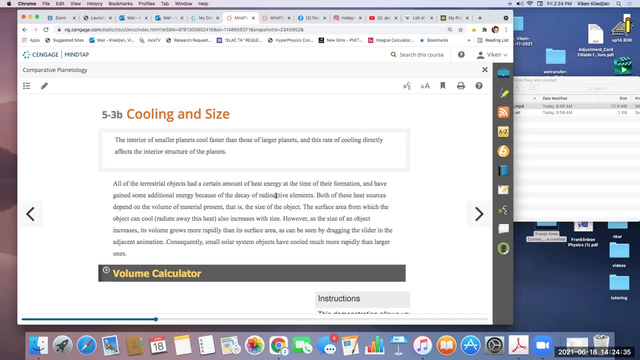 planet cools faster. So all of the terrestrial planets have a certain amount of heat energy at the time of their formation and have gained some additional energy because of the decay of radioactive elements. Both of these heat sources depend on the volume of material present, that is, the size of 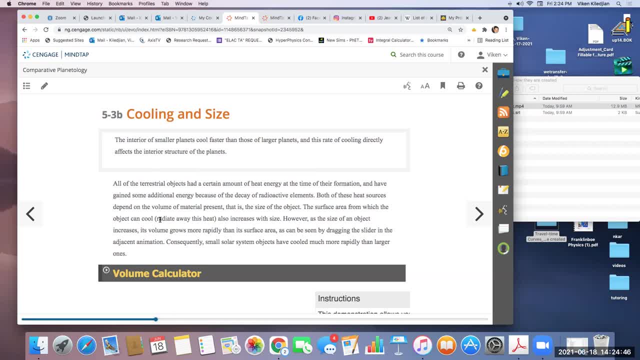 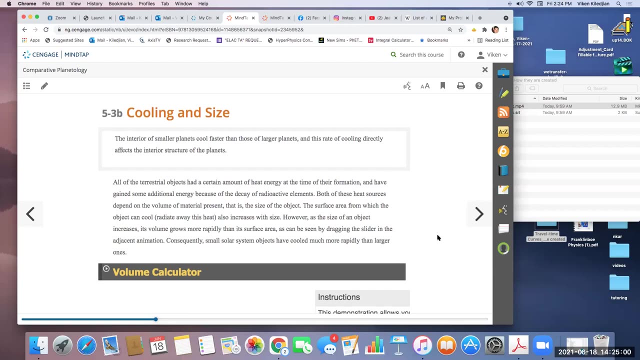 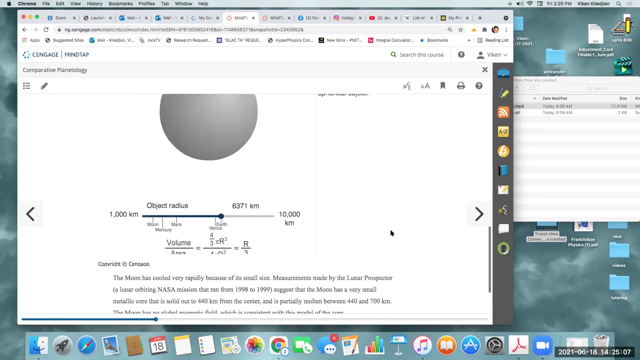 the object. The surface area from which the object can cool also increases with size. However, as the size of an object increases, its volume grows more rapidly than its surface area, as can be seen by dragging the slider in the adjacent animation. So this is trying to show you that larger planets have a bigger volume. 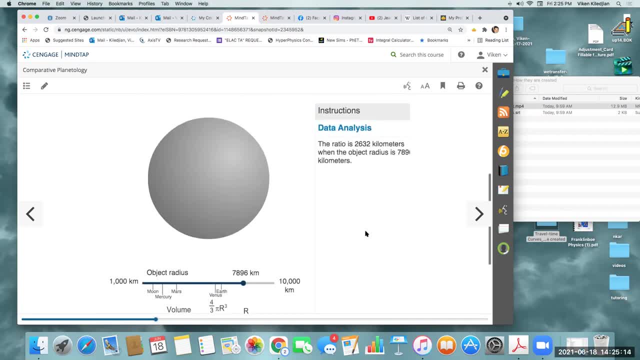 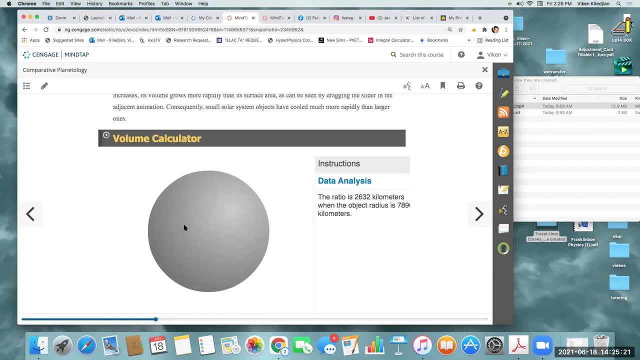 to surface area ratio. So the volume determines how hot the planet was to start with. So, such as Jupiter or those gaseous planets, they were hotter and if you compare Earth and Mars, they were hotter than Mars. sorry. if you compare earth and venus, they were hotter than mars and mercury. so bigger planets are. 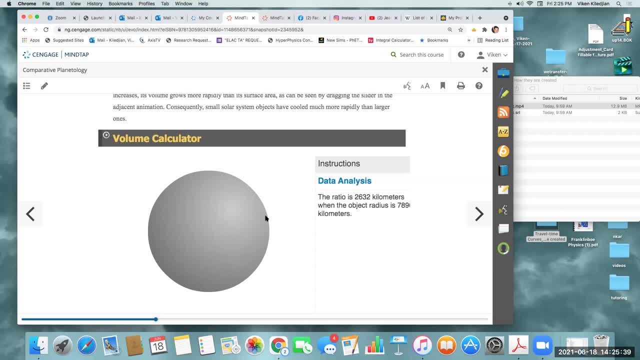 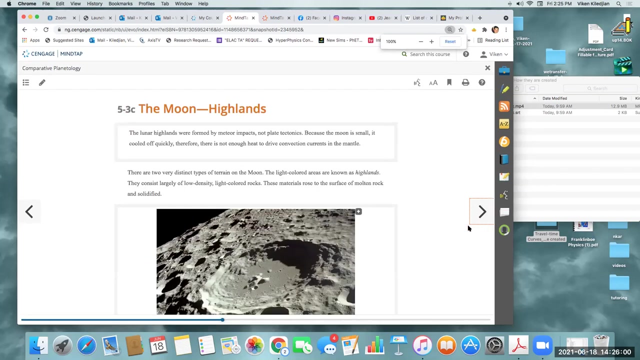 hotter to begin with, and then the surface area tells you how much heat the planet can radiate. but because bigger planets, volume grows larger than their surface area, they retain their heat longer- okay than smaller planets. so let me get a little bit smaller. the lunar highlands were formed by meteor impacts. 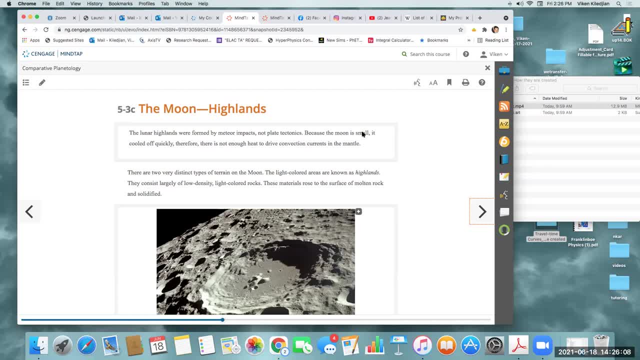 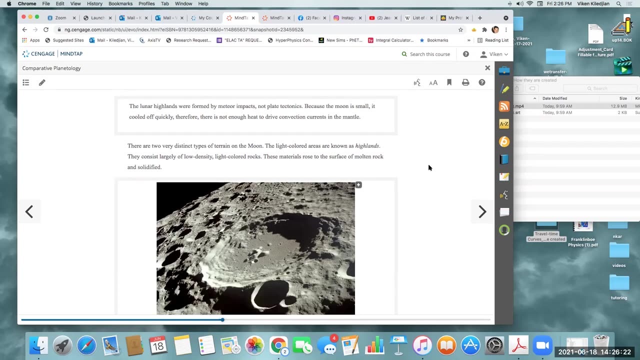 not plate tectonics. because the moon is small. it cooled off quickly. therefore there is not enough heat to drive convection currents in the mantle. you see? so very small objects cool off very quickly, so no convection currents. there are two very distinct properties of the lunar highlands. the lunar highlands are very small objects. 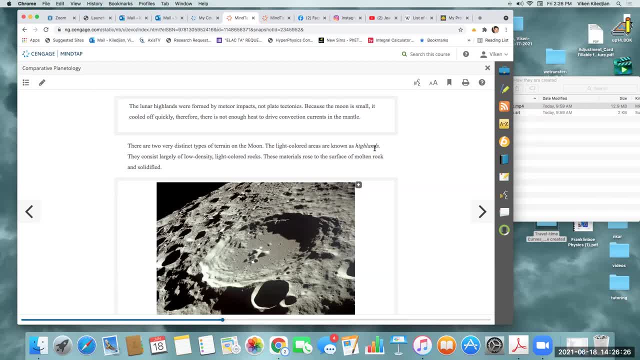 types of terrain on the moon. the light colored area is known as highlands. they consist largely of low density light colored rock. that would be this stuff right here. all this is the highlands, including this, because it's just a crater right there. these are actually all the. highlands right here. okay. these materials rose to the surface of molten rock and solidified. the mountain ranges of the moon were formed by a large impacts. around 4 billion years ago, large chunks of debris crashed into the moon at a high velocity and formed impact basins at the sites of the collisions. mountains formed around the impact. 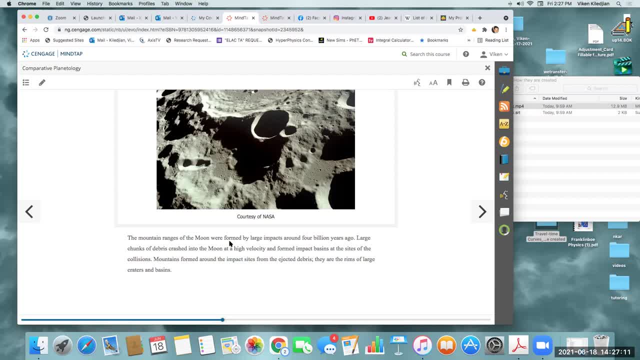 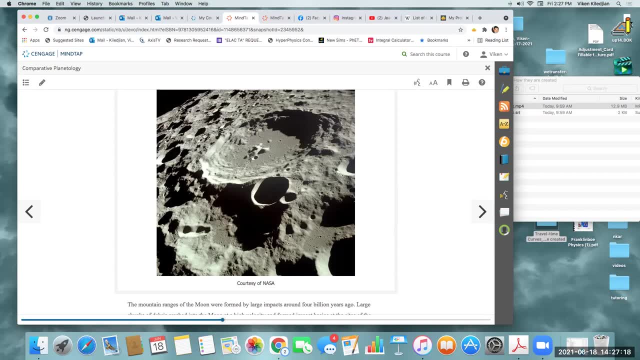 sites from the ejected debris. they are the rims of large craters like this one. you see, so this was our kind of like mountains- the moon is equivalent to a mountain. and then this is the impact basin where the crater was formed, and also another crater here, another crater here, and then 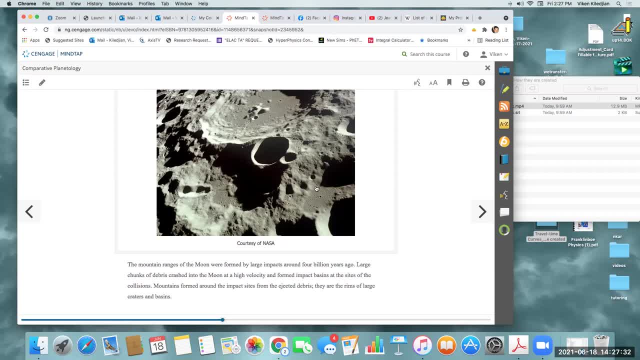 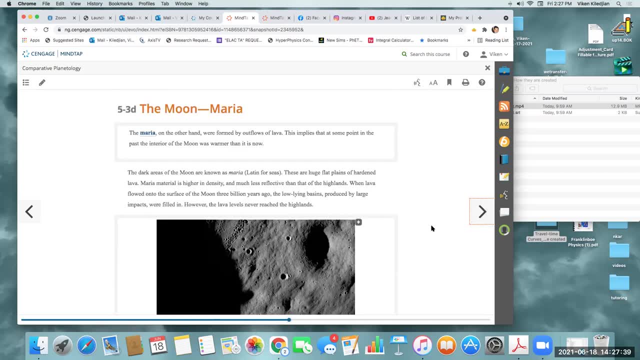 all these smaller craters. this is a large one. this is another large one. the Maria, on the other hand, were formed by outflows of lava. this implies that at some point in the past, the interior of the moon was warmer than it is now. the dark areas of the moon are known as Maria. 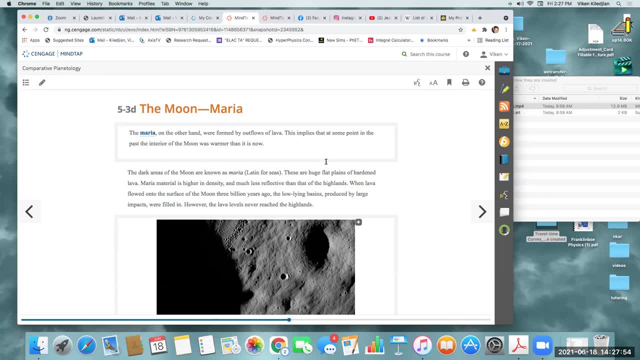 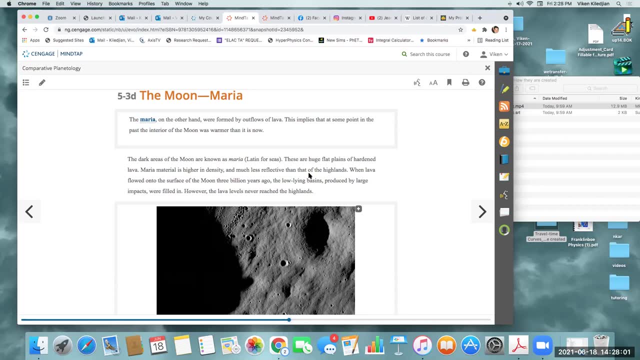 Latin for seas. These huge flat planes of hardened lava Maria material is higher in density and much less reflective than that of the highlands When lava flowed onto the surface of the moon three billion years ago. the low-lying basins produced by large impacts 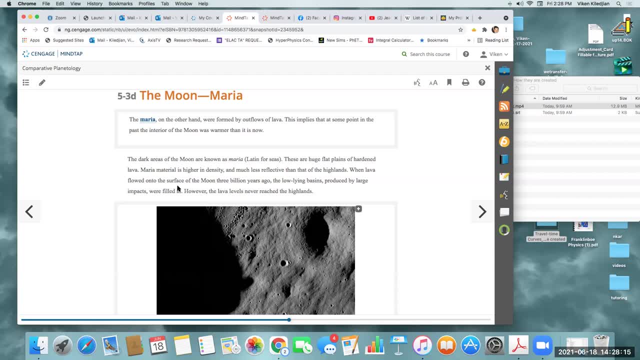 were filled in. However, the lava levels never reached the highlands. Oh, you see that. So the lava basically went up to the surface, flowed all the places where there were impact craters and all the lowlands, but they never reached way up to the highlands. 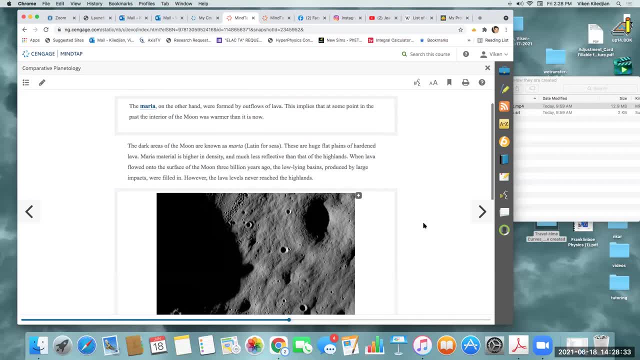 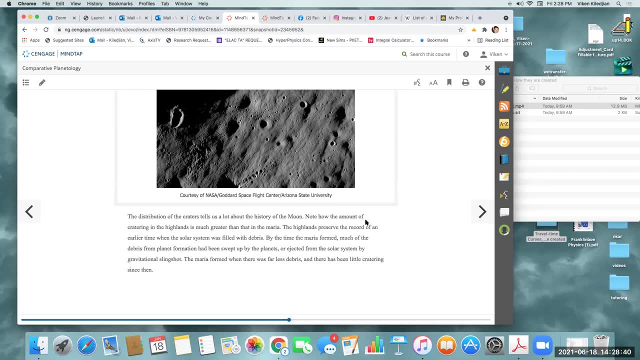 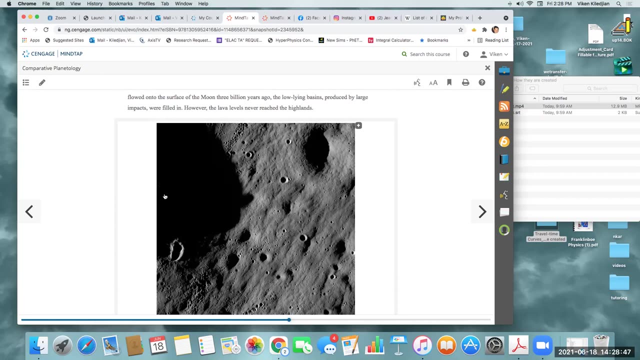 to cover all of the highlands. The distribution of the craters tells us a lot about the history of the moon. Note how the amount of cratering in the highlands is much greater than that in the Maria. So these are the Maria, right here the dark spots. 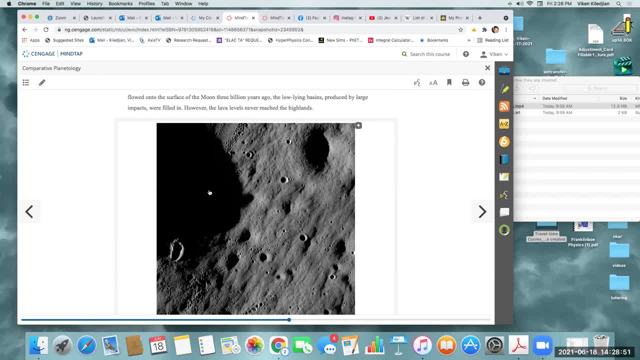 Well, there's a lot more craters on the highlands right here than in the Maria. So that tells us that the Maria formed after the cratering and then came and filled up that region. you see, So if I show you another images of the moon, 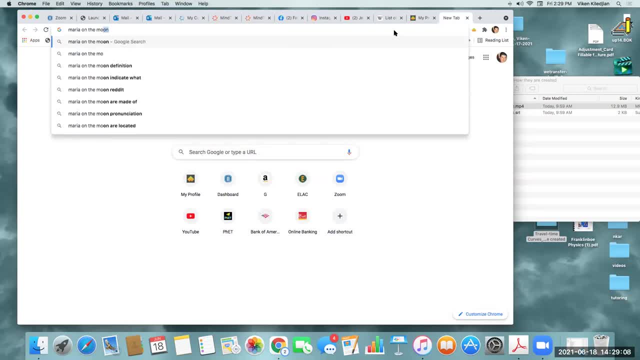 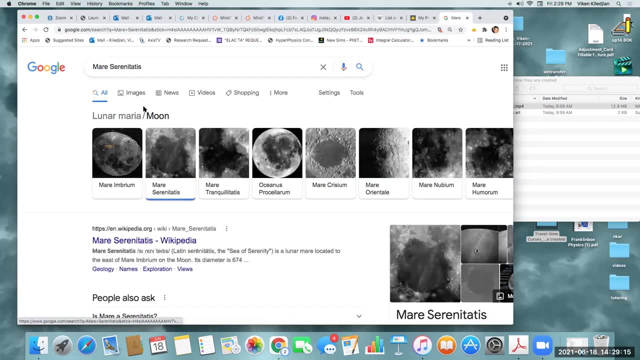 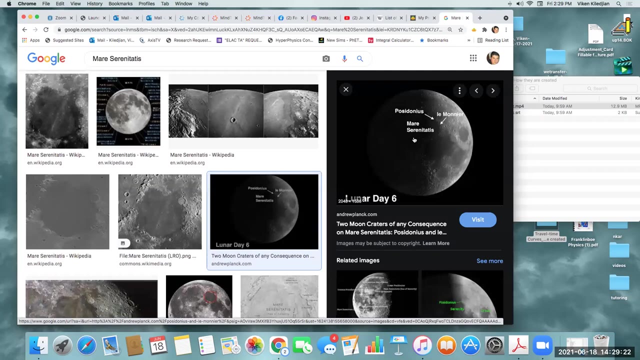 you could see Maria on the moon. You see there, those are all the Maria right there. That's a nice image. You see here, that's a Maria right there. That's Maria right there. Mare, it's Latin is mare. 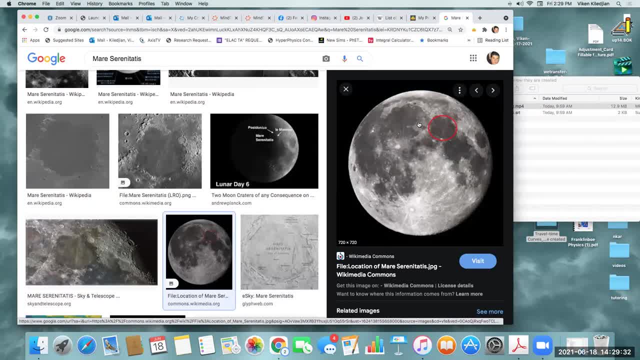 You see, this is another one. Oh, you see, the Maria, interestingly, are only found on the side of the moon facing us. You see, here, these are all the Maria, right here, They're denser and they are filling up the lower regions. 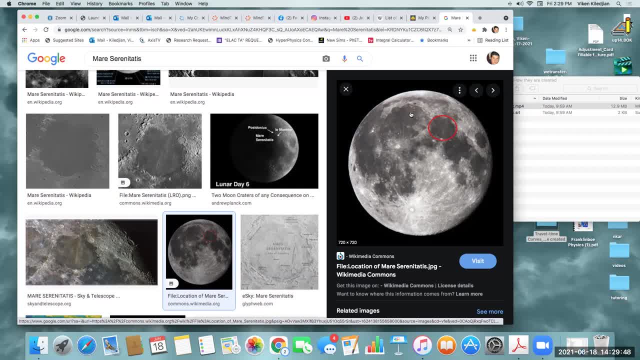 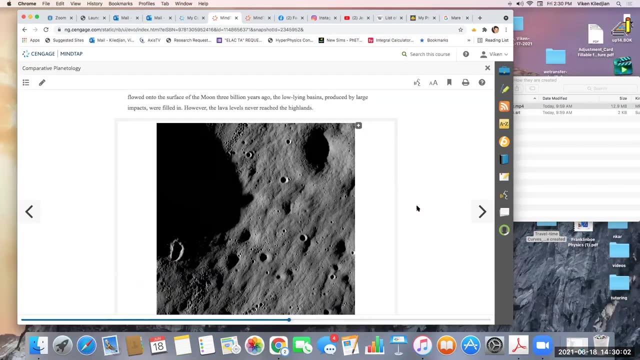 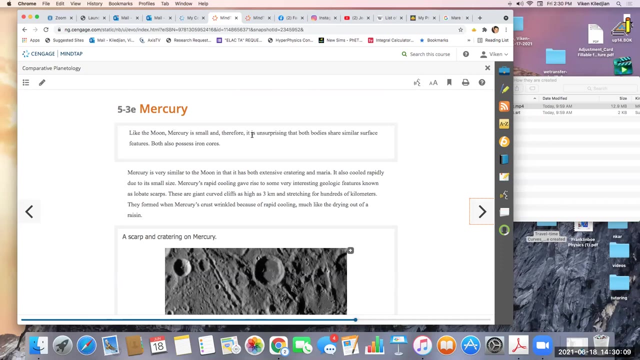 of the lower region. These are basins of the moon And they don't have as much craters, you see, as the highlands. These are all the highlands right here. Okay, Mercury, like the moon, Mercury is small. 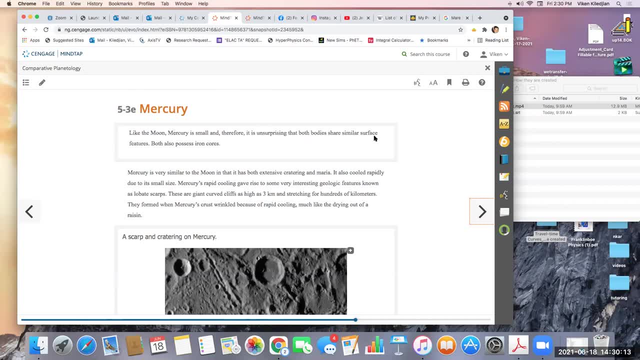 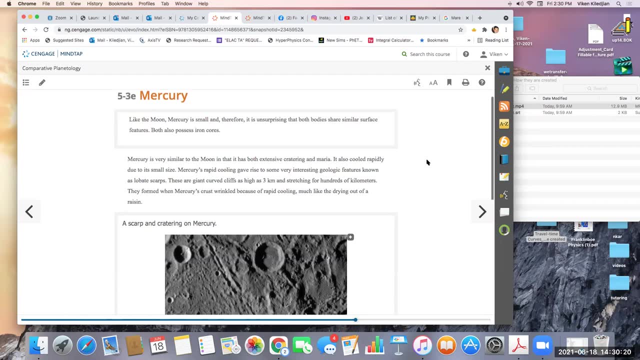 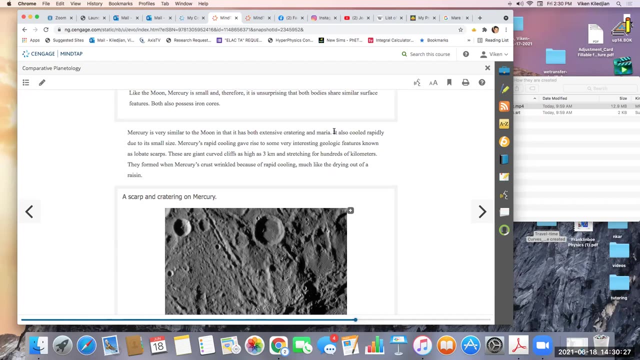 and therefore it is unsurprising that both bodies share similar surface features. Both also possess iron cores, Both the Mercury and the moon. Mercury is very similar to the moon in that it has both extensive cratering and Maria, So the Mercury does have both. 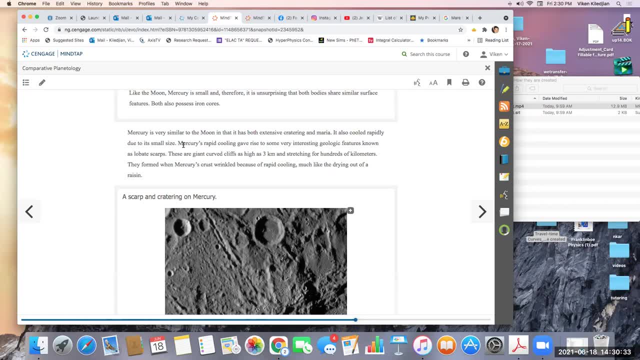 It also cooled rapidly due to its small size. Mercury's rapid cooling gave rise to some very interesting geologic features known as lobate scarps. These are giant curved cliffs as high as three kilometers and stretching for hundreds of kilometers. So there are three kilometers is actually pretty high. 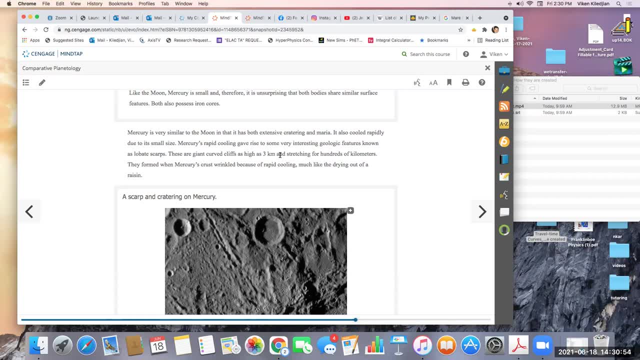 That's like one mile one and a half miles, So that's about a good 7,000 feet. That's how high the lobate scarps is. They form when Mercury's crust wrinkled because of rapid cooling, much like the drying out of a raisin. 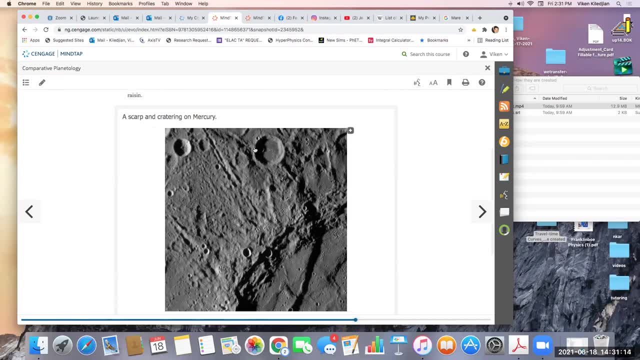 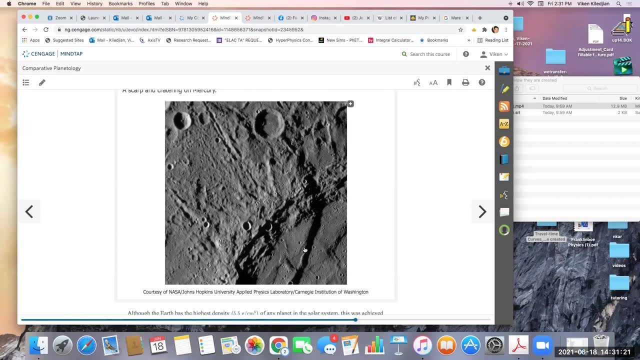 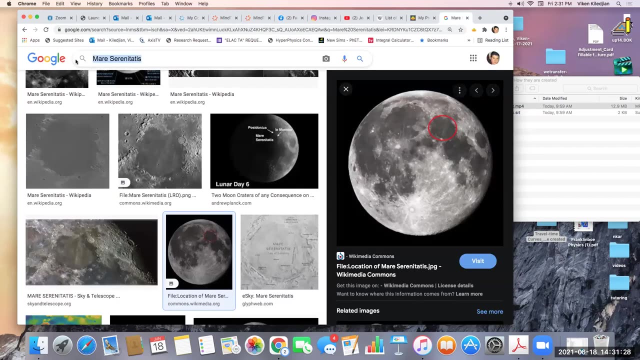 Her scarps and cratering on Mercury. This is the lobate scarps right here, I believe right here. all of this. One side of it is higher than the other side by about three kilometers. Let's see. So we can see her lobate scarp on Mercury. 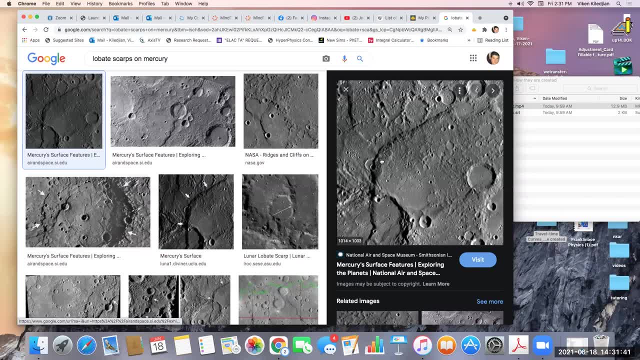 So several pictures of it you see here. Now we can't tell that one side of it is that much higher than the other because we're looking at it from the top. But if we go- on the surface and take a picture, this side will appear a mountain. 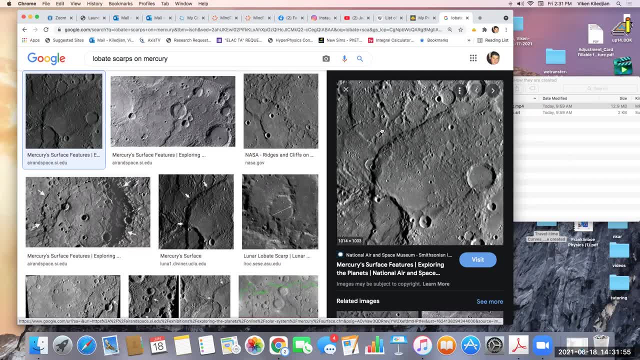 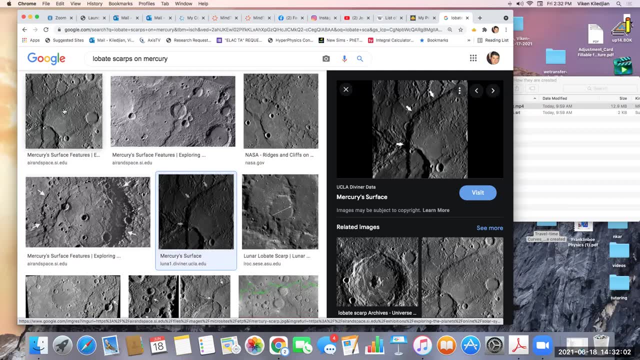 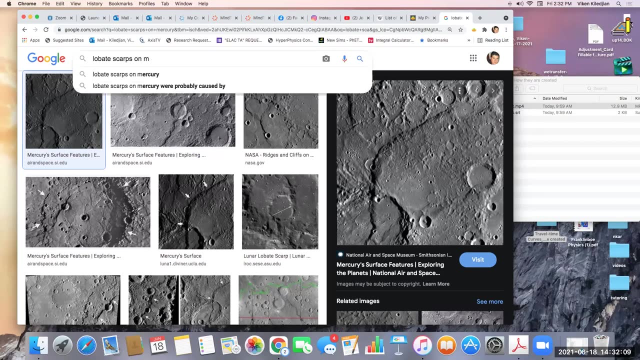 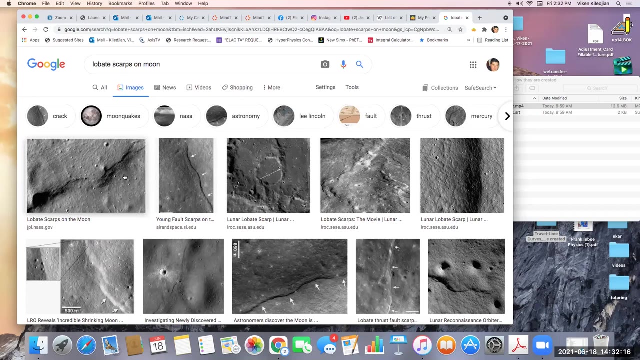 like a mile or a half higher than this. you see, Yeah, those are some good pictures there. you see, Like that, Probably the moon has some too, but maybe not as extensive. Yeah, there are some. Yeah, right there. 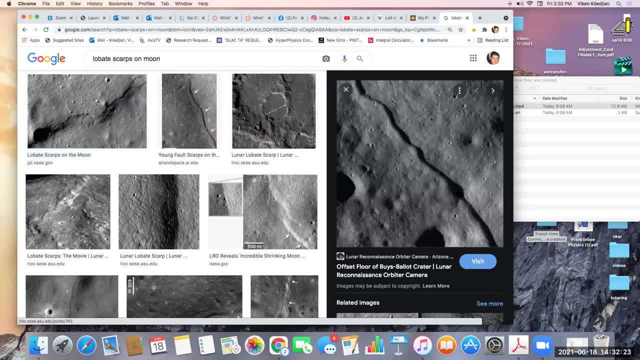 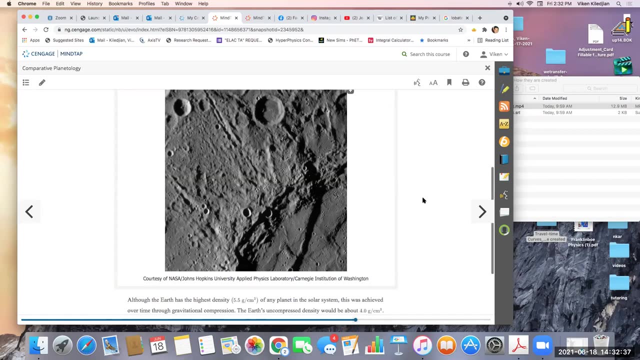 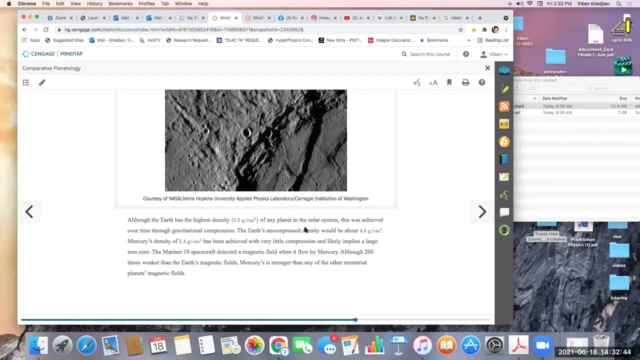 This is for the moon. Yeah, right there, Okay. So it says: although the earth has the highest density- remember it was 5.5, this was achieved over time through gravitational compression. The earth's uncompressed density would be about four gram per cubic centimeter. 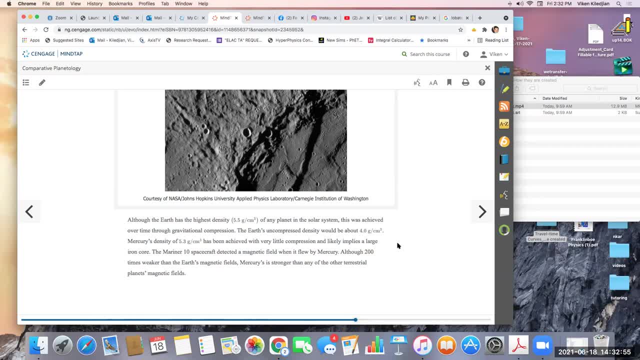 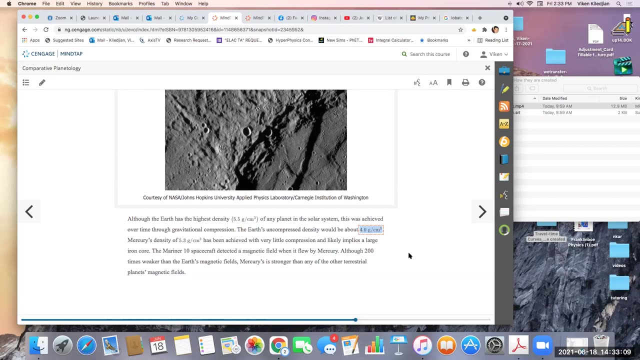 Remember the fact that you compress it, something that also tends to increase its density because you're squishing it into a smaller size. So if the earth wasn't compressed due to its gravity, it would have a density of four grams per cubic centimeter. 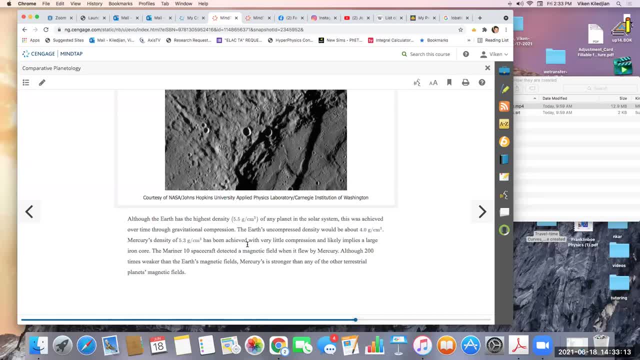 Mercury's density is 5.3, has been achieved with very little compression and likely implies a large iron core. Okay, so Mercury's density is more pure density, without compression, Because, since it's small, it doesn't have as much gravity as the earth. 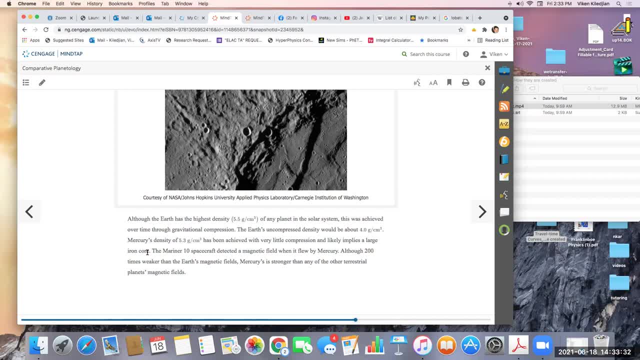 so it's not being compressed due to gravity as much, So the fact that Mercury's density is 5.3 is more real with that density. That means you wouldn't want a planet like that impacting you. It's pretty much made of solid, a lot of solid, solid, solid. 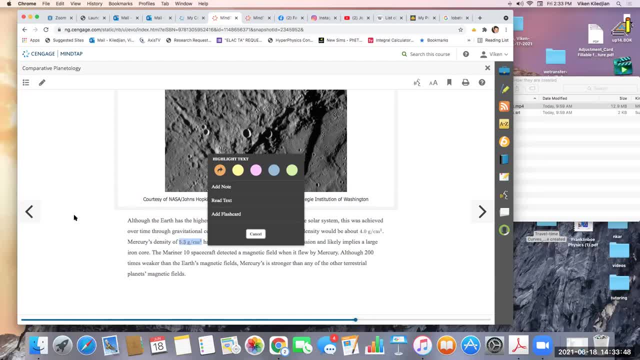 It's pretty much made of solid, a lot of solid, solid, solid. It's pretty much made of solid, a lot of solid, solid, solid. We saw that the earth didn't have solid iron in there, Mercury. That's why it has that density. So we were to compare the uncompressed density of Mercury to the earth, Mercury would be higher. The Marin-Arten spacecraft detected the magnetic field when it flew by Mercury. Although 200 times weaker than the earth's magnetic field, Mercury's is stronger. 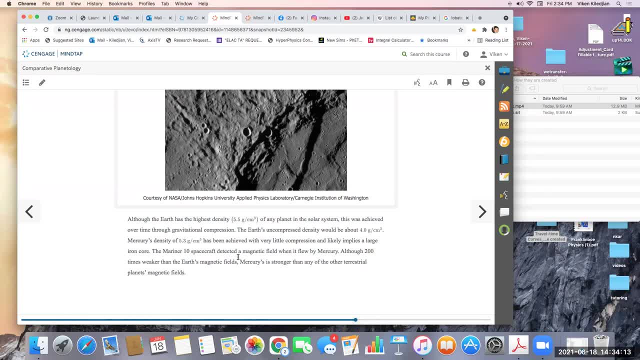 than any other terrestrial planets magnetic field. That's interesting, Even though it doesn't have molten core inside, it doesn't have a liquid core, but because it has iron core so big that is still enough to create the second strongest magnetic field from the terrestrial planets. 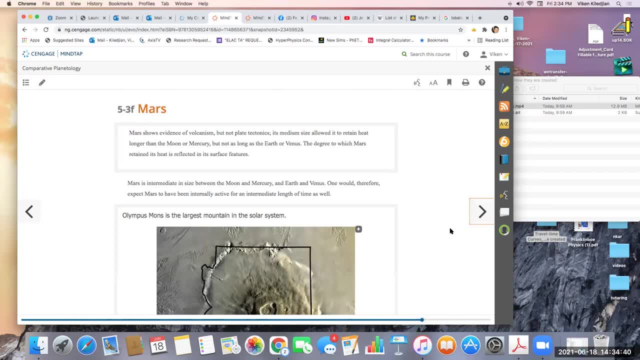 okay, now we go to mars. mars shows evidence of volcanism, but not plate tectonics. so it does have a lot of volcanoes, but not plate tectonics. its medium size allowed it to retain heat longer than the moon or mercury, but not as long as the earth or venus. 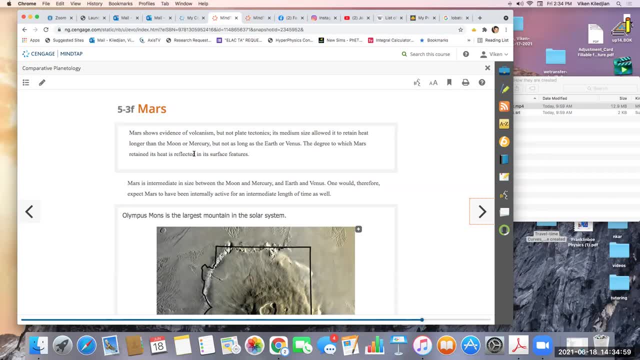 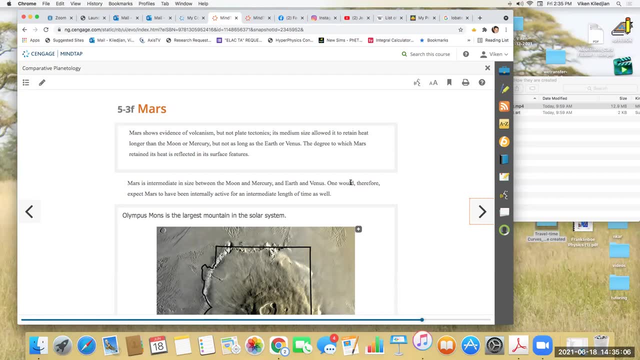 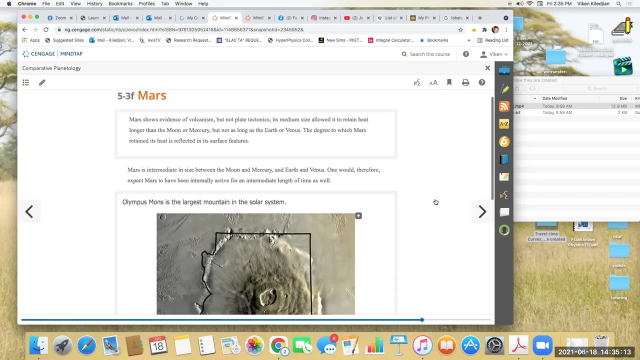 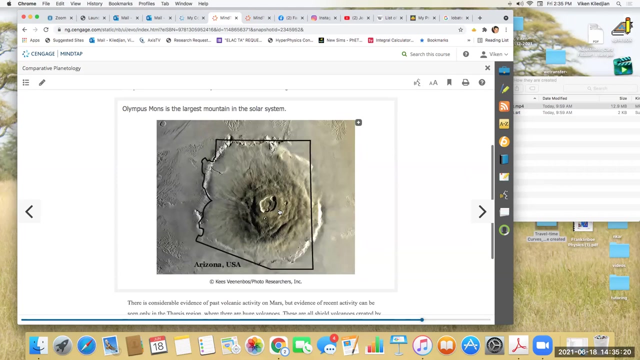 the degree to which mars retained its heat is reflected in its surface features. mars is intermediate in size between moon and mercury, and earth and venus. one would therefore expect mars to have been internally active for an intermediate length of time. olympus moon is the largest mountain in the solar system. this is a view of the olympus bones from the top. 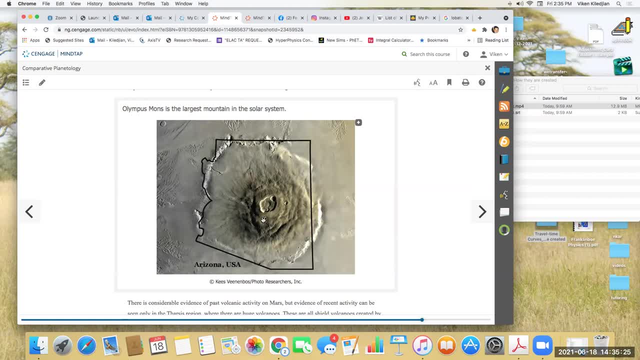 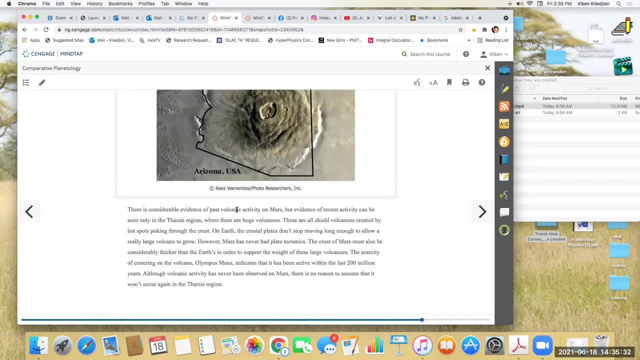 look at it it looks like as big as arizona. that is huge mountain. so there's considerable evidence of past volcanic activity on mars. but evidence of recent activity can be seen only in the tharsis region, where there are huge volcanoes, all shield volcanoes created by hot spots poking through the crust, so kind of like the one that we 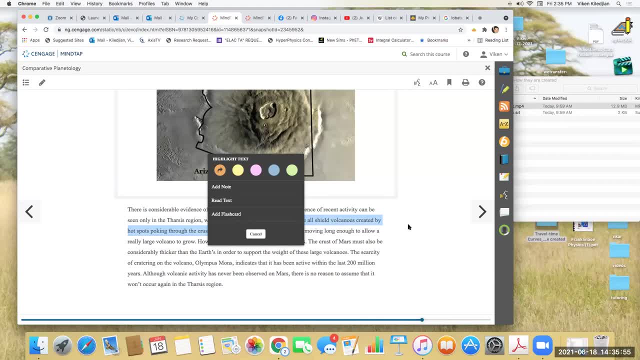 called um hawaii. hawaii is also an example of a shield: volcanoes coming from the hot spots on earth. the crustal plates don't stop moving long enough to allow a real large volcano to grow. remember how they keep moving. that's why you get the formation of the hawaiian islands. right, but on mars the crust doesn't move, so a hot spot keeps creating a mountain. that's why you get a mountain like olympus moans in the same spot. it's the largest mountain in the solar system. so it says: olympus moans indicates that he has been active within the last 200 million years. 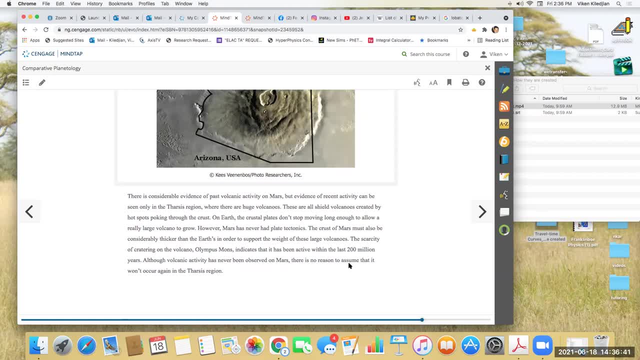 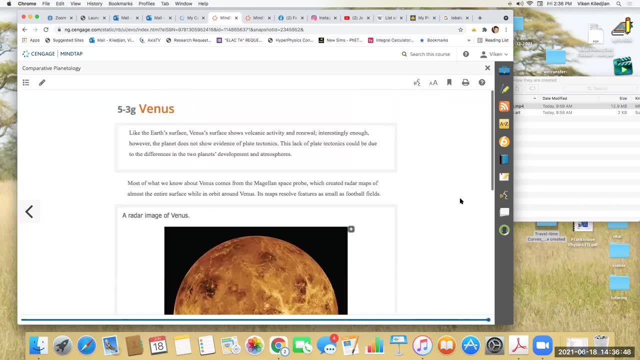 although volcanic activity has never been observed on mars, there's no reason to assume that it won't occur again in the tharsis region. now on to venus. like the earth's surface, venus's surface shows volcanic activity and renewal, so that one that means we keep seeing more volcanic activity on venus. 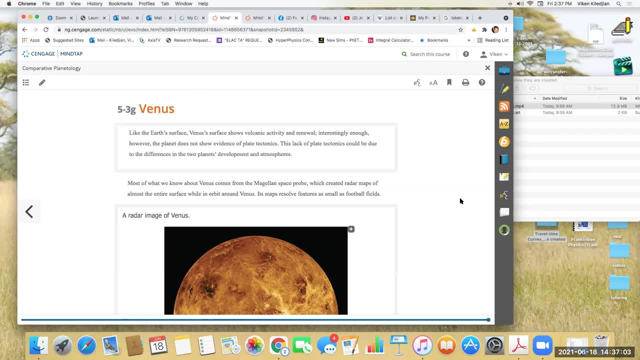 whereas in mars not as much, but in the past there has been. interestingly enough, however, the planet does not show evidence of plate tectonics. this lack of plate tectonics is a sign of the fact that the planet is moving in the right direction. 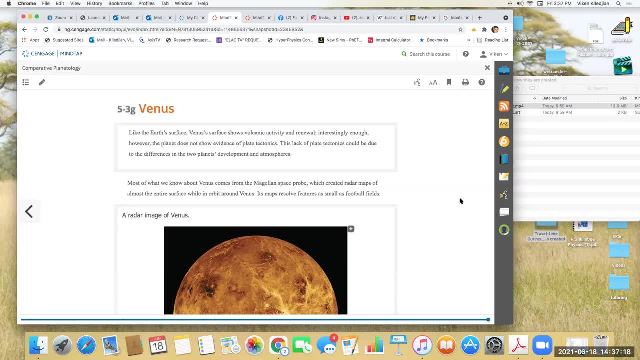 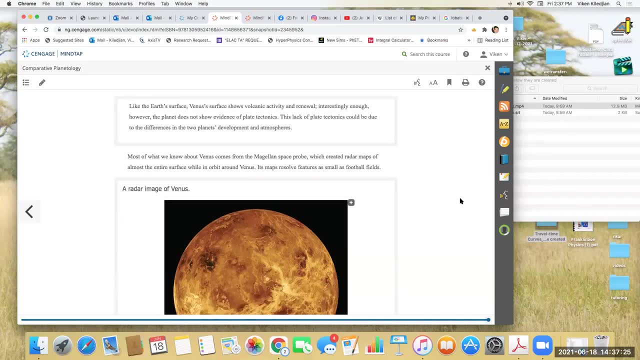 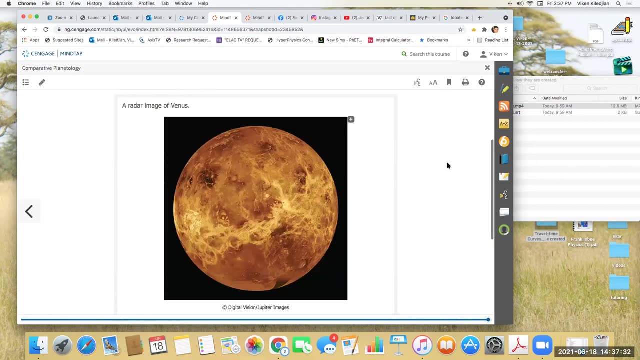 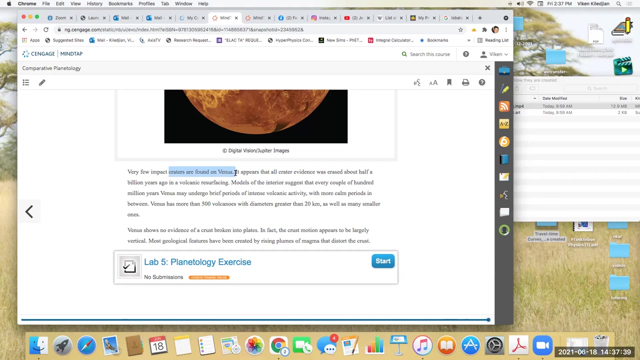 so, then, the difference is in the two planets, development and atmospheres. most of what we know about venus comes from the magellan space probe, which created radar maps of almost the entire surface. so, venus, very few impact craters are found on venus. it appears that all crater evidence was. 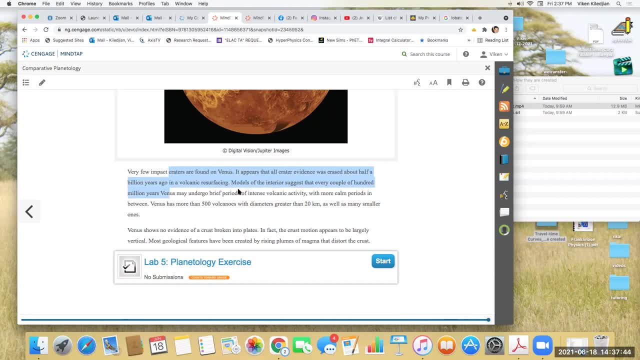 erased about a half a billion years ago in bohon. volcanic resurfacing. It's kind of how the earth rejuvenates its crust. Similar thing is happening on Venus, but without plate tectonics. The volcanoes, eruptions, the lava flow is just. 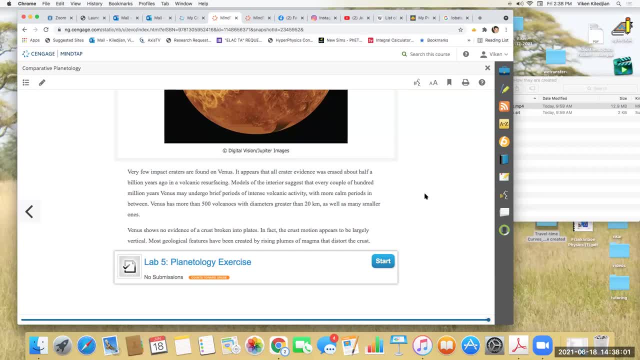 covering up the cratering so you don't really see it. So all the craters, about half of them. so sorry. it appears that all crater evidence was erased about a half a billion years ago. Most of the interior suggested every couple hundred million years Venus may undergo. 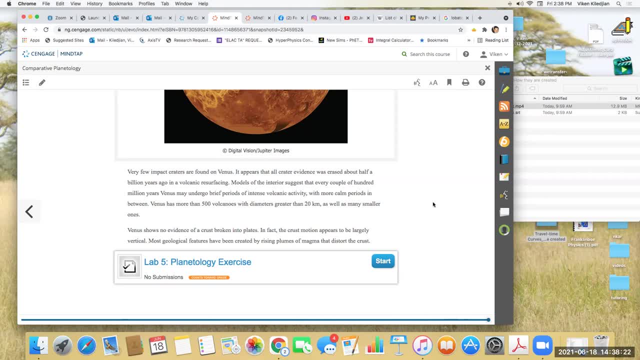 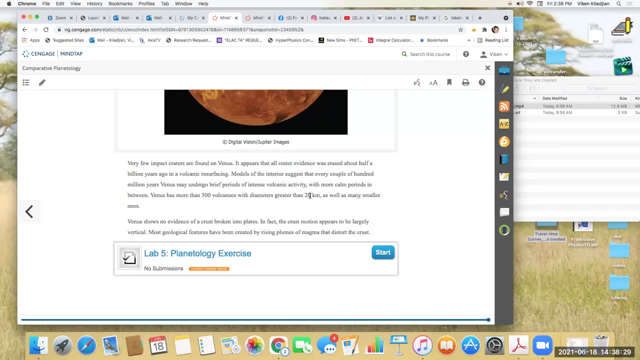 brief periods of intense volcanic activity. Venus has more than 500 volcanoes with diameters greater than 20 kilometers. That's a lot, a lot. So Venus shows no evidence of crusts broken into plates. In fact, the crust motion appears to be. 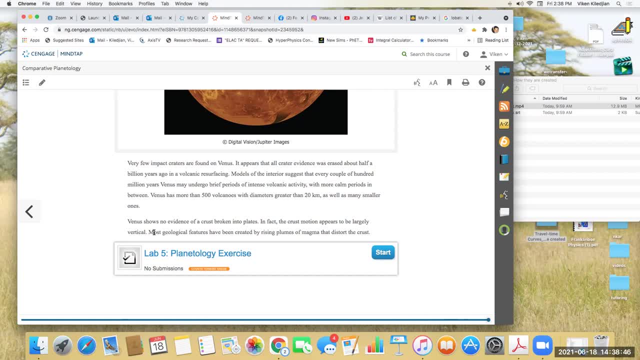 largely broken into plates. So Venus shows no evidence of crusts broken into plates. In fact, the crust motion appears to be largely broken into plates. So Venus shows no evidence of crusts broken into plates. Oh, okay, so the crust goes up and down, but not sideways. Okay, start. 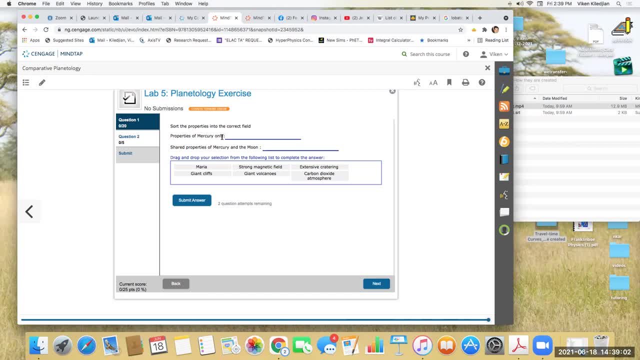 Sort the properties into the correct field- Properties of Mercury. only then you can just sort them here- Shared properties of Mercury and the Moon- and then you could put those over here, And then that one is just pretty much just doing it. So then question two: 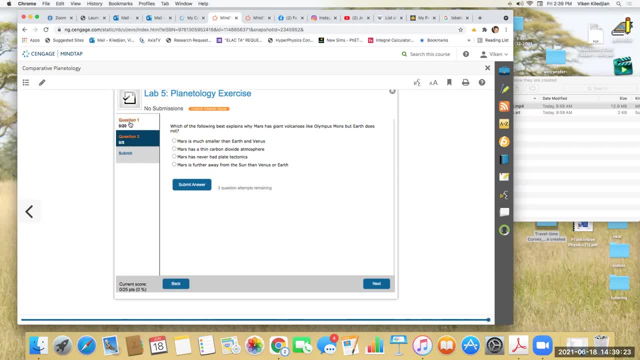 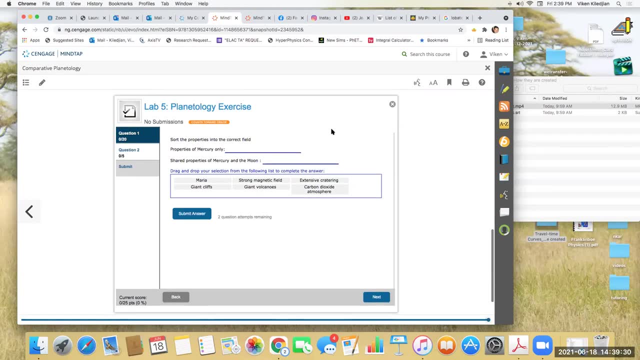 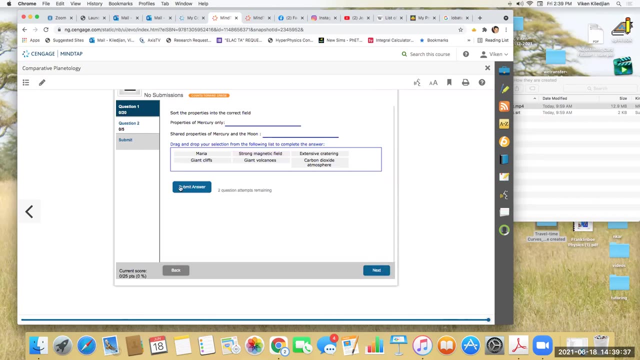 this is why Mars is a giant volcano like Olympus Mons. Okay, that one. you can just take a picture of your final score, So it's not really based on anything that you do on top here. So just answer this, hit submit question two, and then hit submit And then, once you, 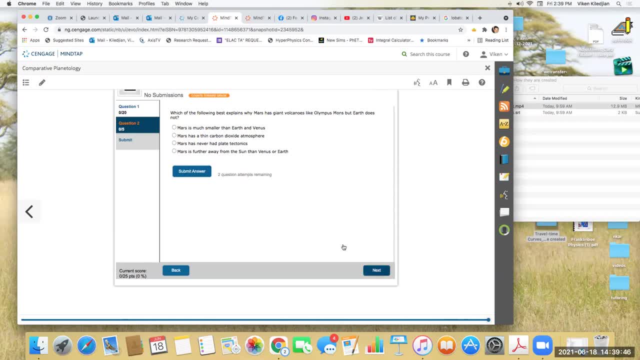 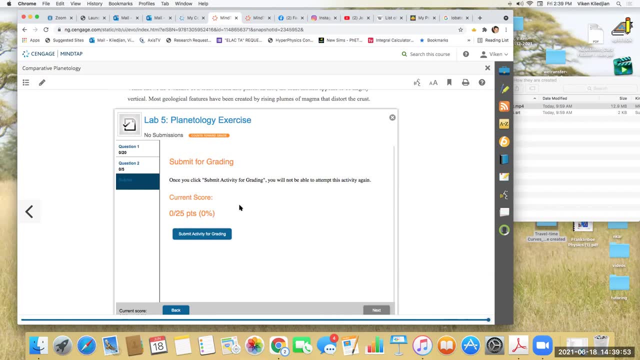 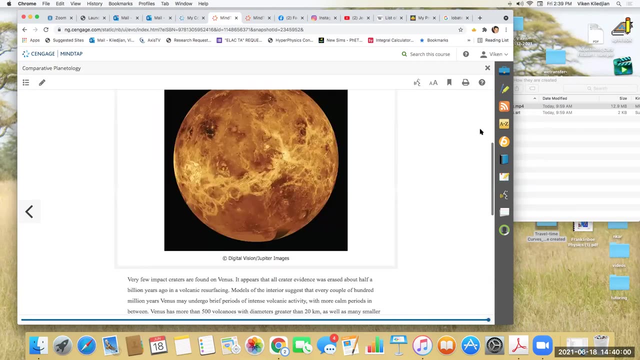 press next it shows the score And that's all. that's all you need for that one. Just show the score of how many you got. I think that's it Very interesting stuff. So even though this one, this section didn't have much exercise on it, but I still usually like to read this section.